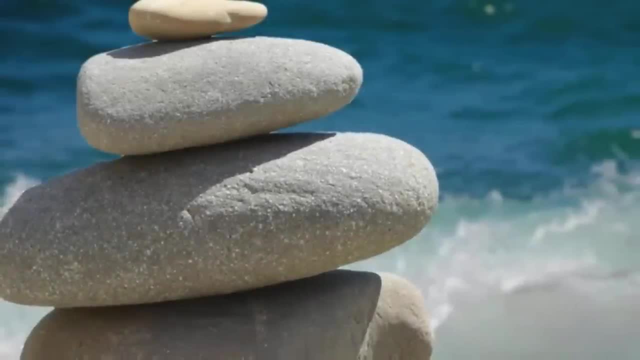 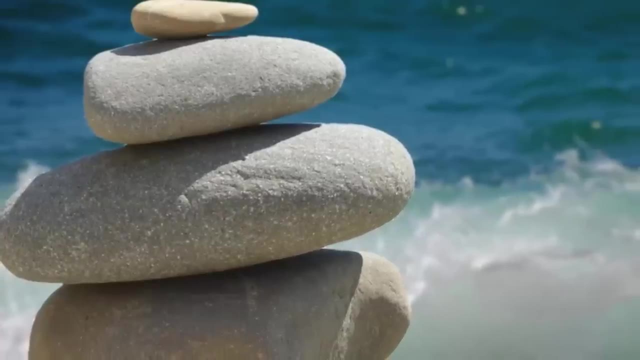 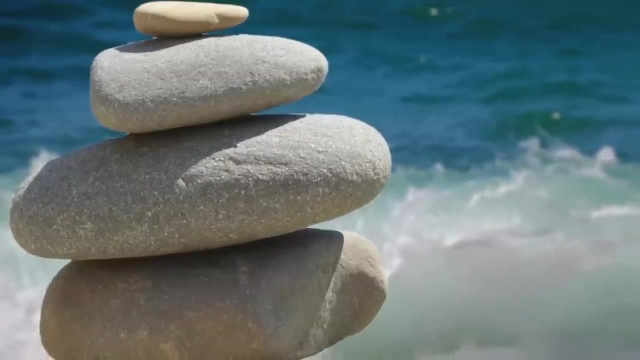 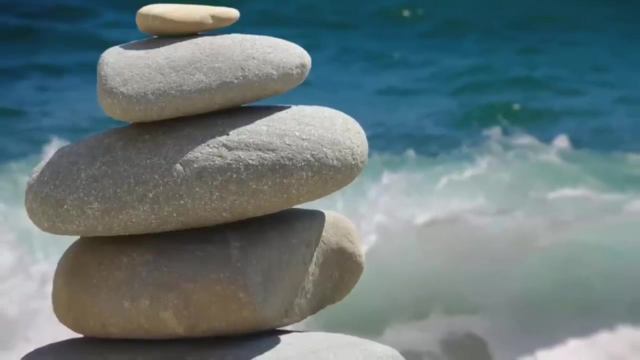 As you say, these affirmations know that they will help you adopt a better belief system in all areas of your life And in doing so, you can develop a higher, more positive consciousness. To support these affirmations even more, I also have a hypnosis version of this recording. 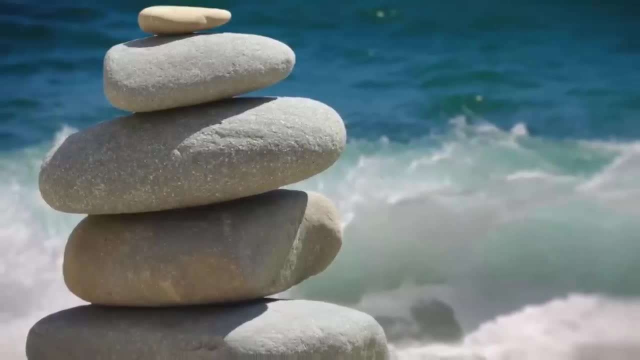 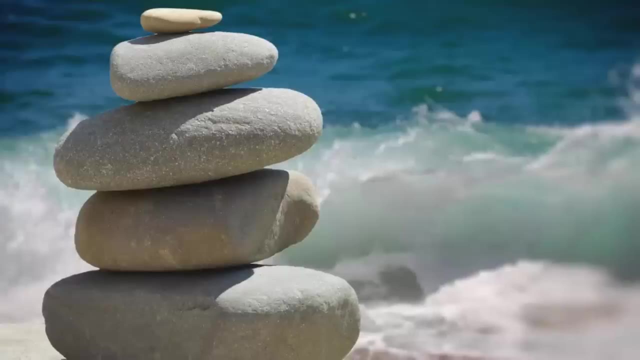 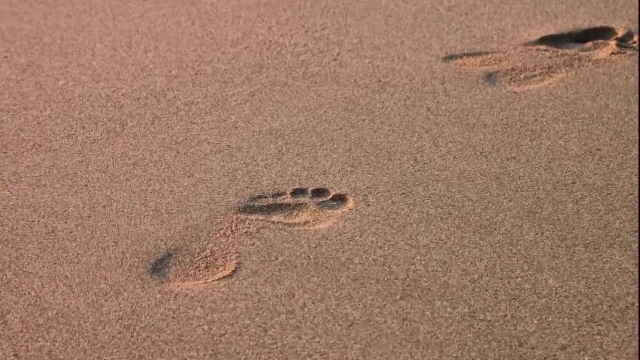 You can use it to reinforce these affirmations if you so wish. So just look out for my next recording, which can be used as a companion to this one, And, generally speaking, continue your affirmations until you begin to see some positive changes taking place in yourself. 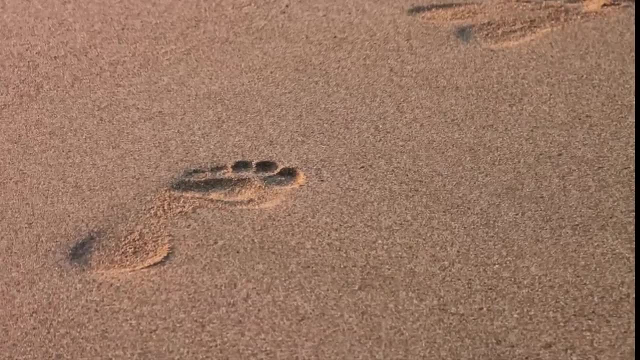 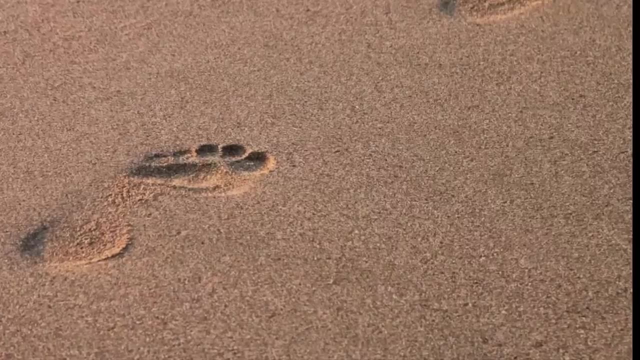 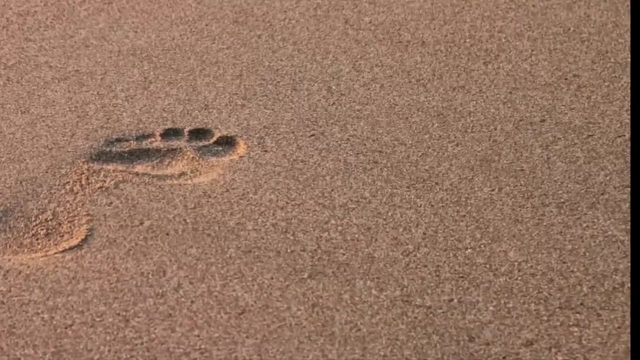 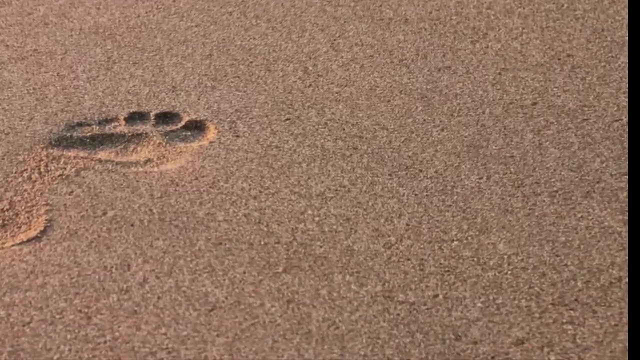 It doesn't matter where you're starting from, when you begin the work of self-transformation or self-improvement. We all have the capacity for improvement. Just know that the changes are gradually happening on the inside. It's like planting seeds. Release your expectations of how and when things will happen. 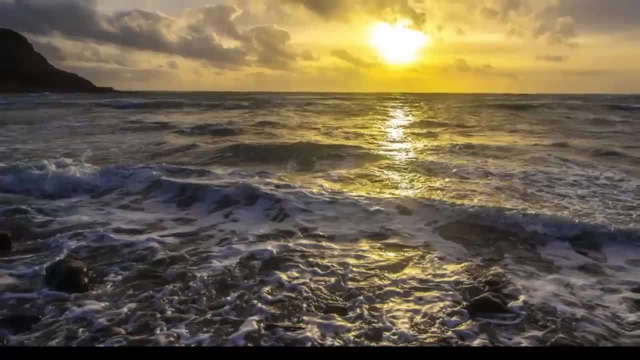 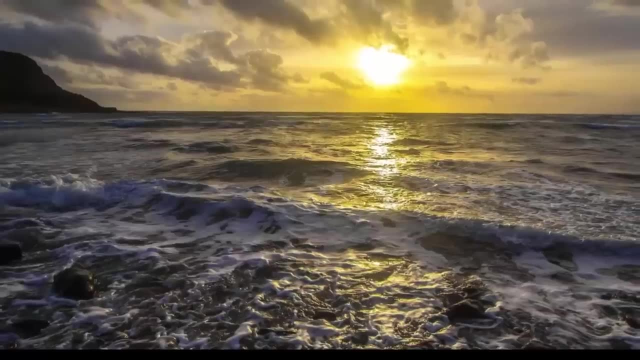 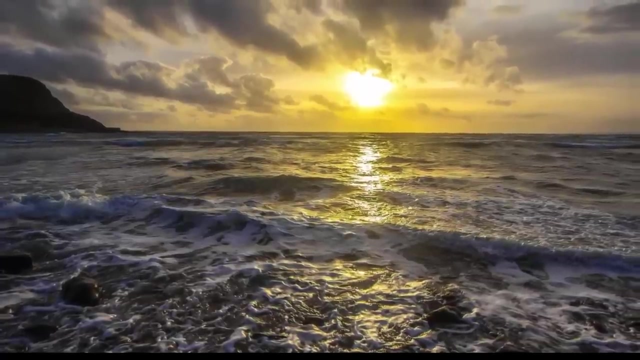 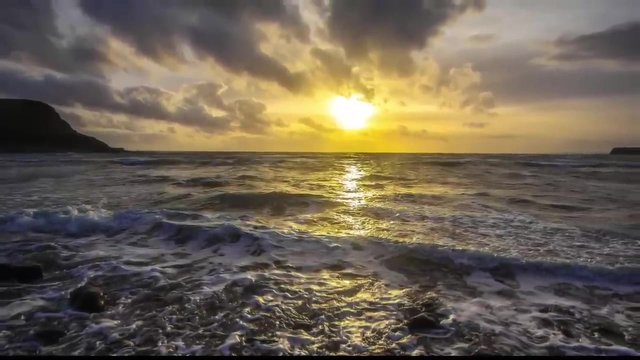 Expectations can cause resistance and slow down your progress, And all change happens on an internal and deeper subconscious level And sooner or later manifests outward into an external reality. As we elevate our consciousness even higher, we open ourselves up to more of the good things that we have. 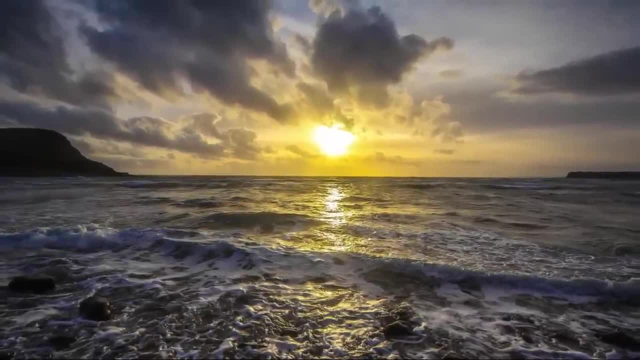 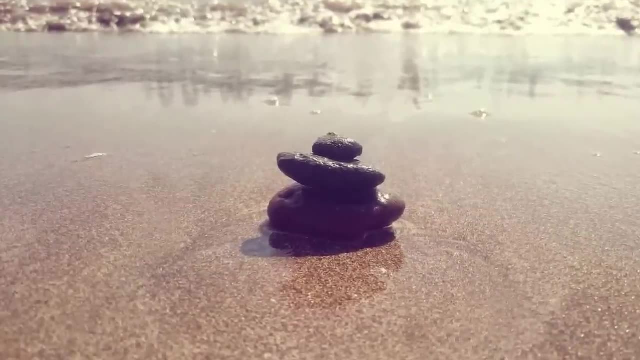 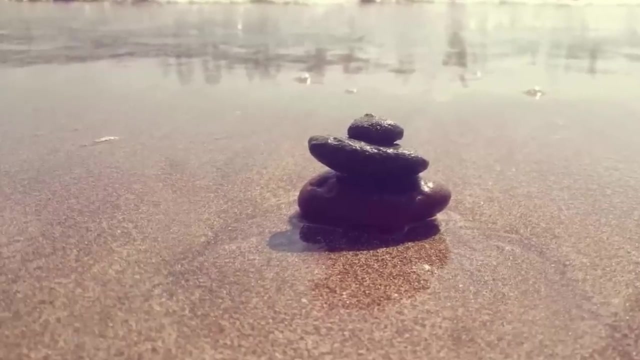 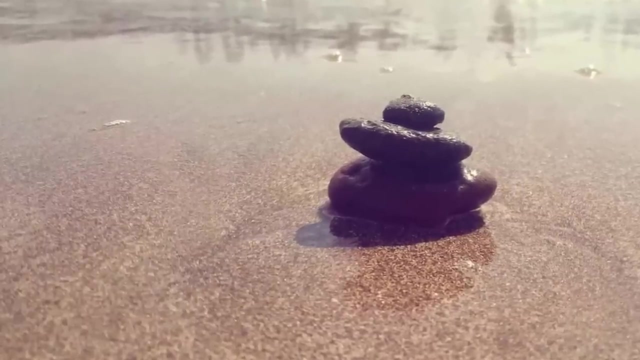 We open ourselves up to more of the goodness that life in the universe has to offer. So take a few big, deep breaths, Allowing your stomach to rise and fall with each breath. Breathe in all the goodness of wonderful things yet to come. 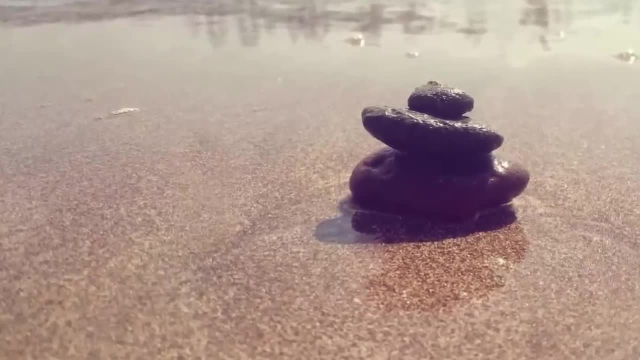 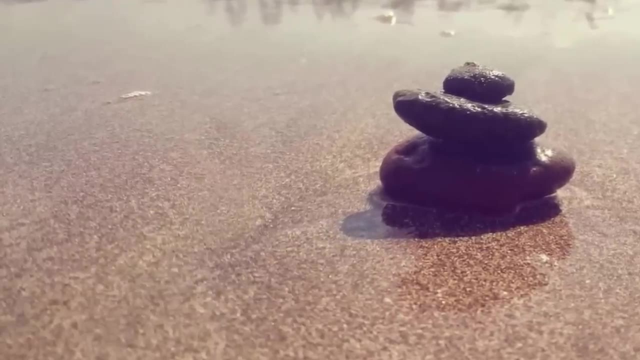 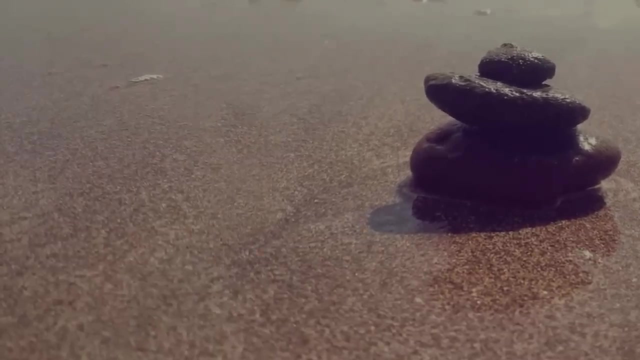 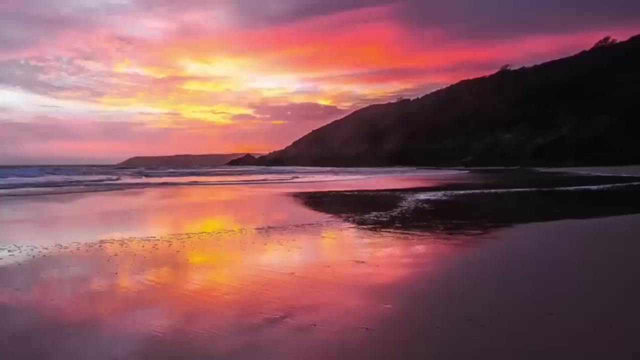 And, on the out-breath, release all that which you need to let go of, Breathe in and, in your mind's eye, Create a vision of a better you. And, on the out-breath, let go of any and all self-criticism. 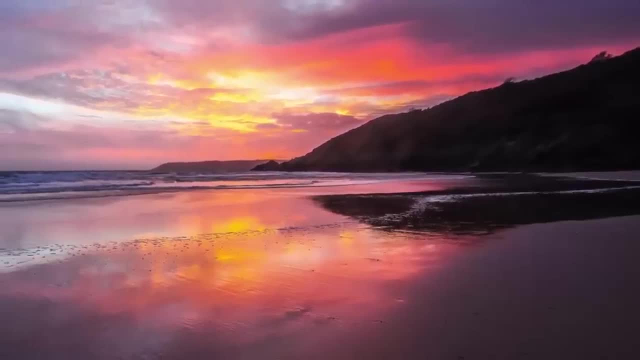 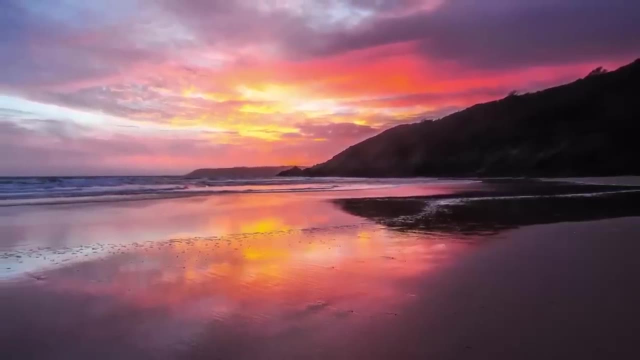 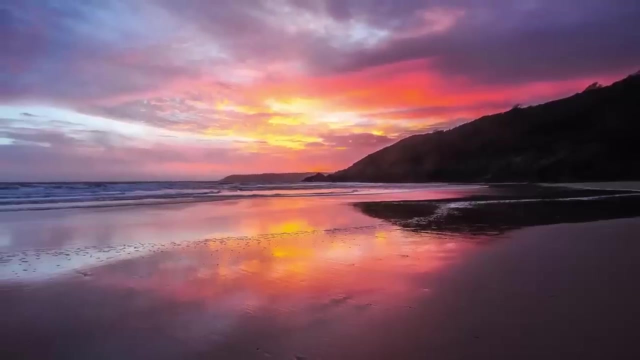 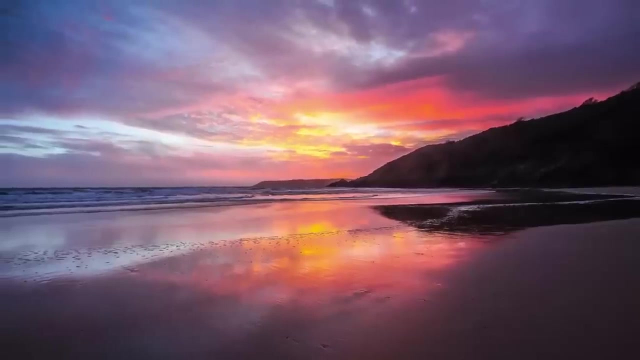 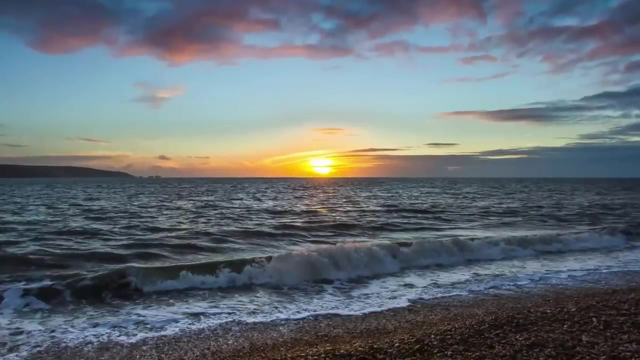 Just let it go. Just let it go, Breathe in this vision of a new you, All your hopes and dreams, And breathe out any tension over things that didn't work out previously. Everything will be okay And when you feel comfortable and relaxed. 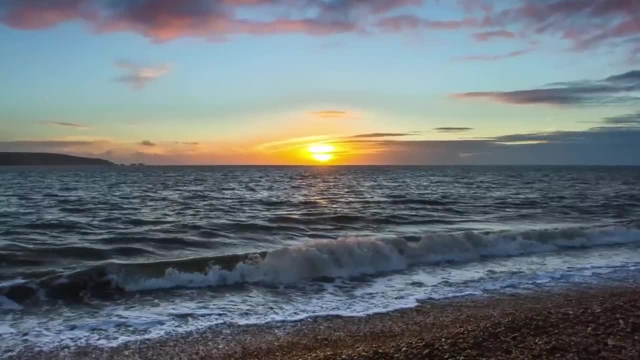 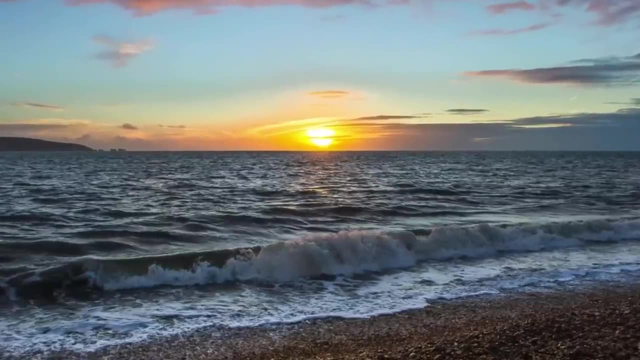 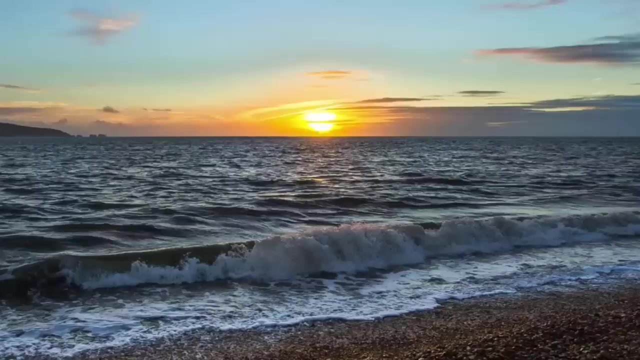 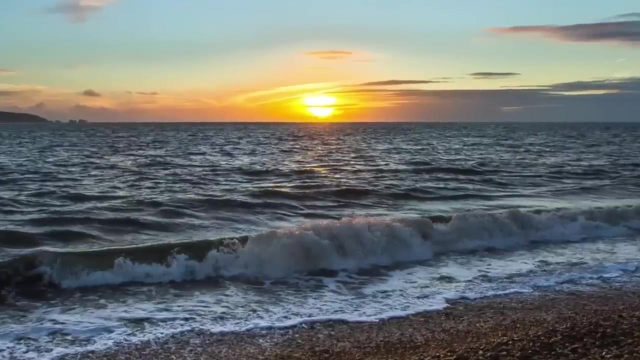 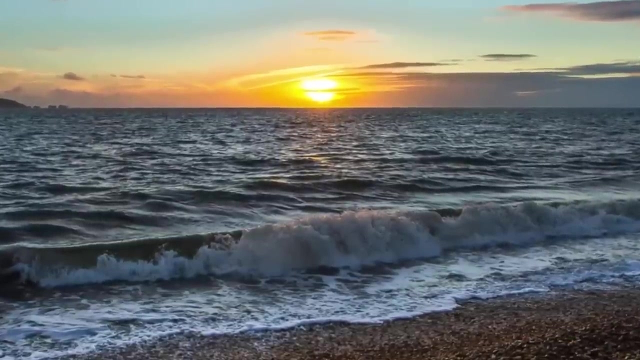 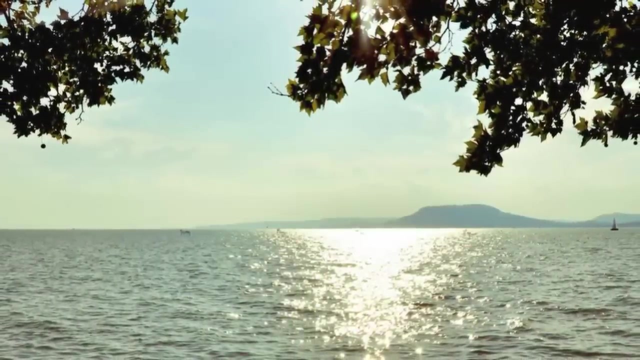 just open yourself up to the idea of becoming a better version of you, Growing stronger, Wiser, More resilient, Someone who lives deliberately, A conscious creator of your own life, As you create your future one day at a time. The following affirmations are in the first person: 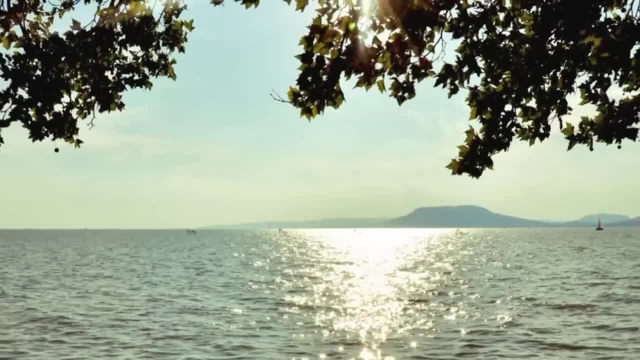 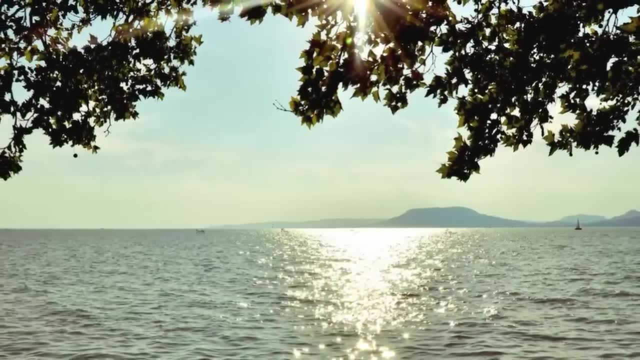 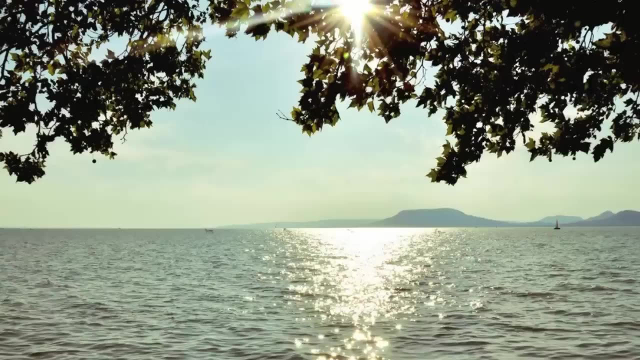 With pauses in between, So you can repeat the affirmations to yourself quietly, Or you can repeat them slowly in your mind And if you encounter an affirmation or phrase that doesn't align with you, Doesn't resonate with you or doesn't apply to you, 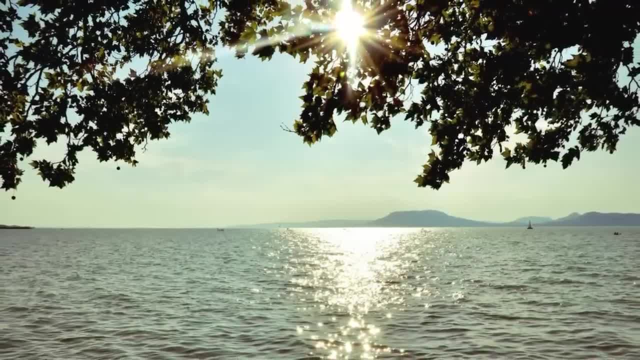 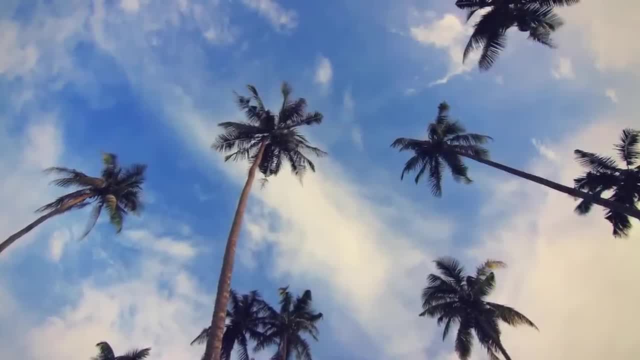 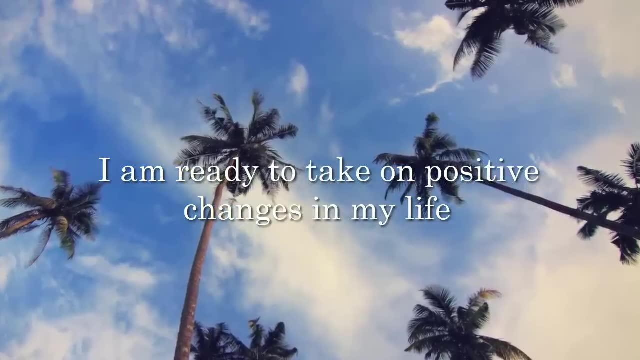 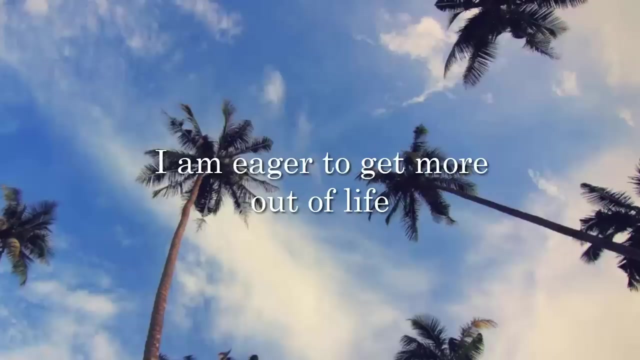 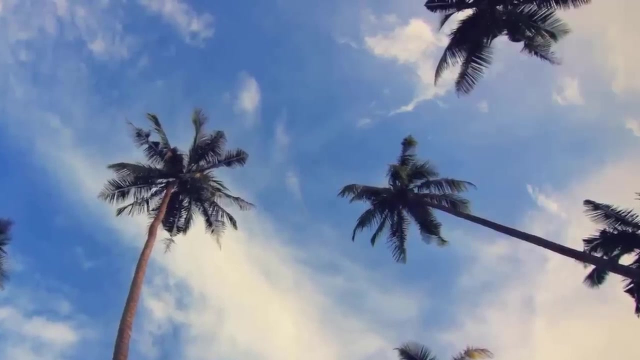 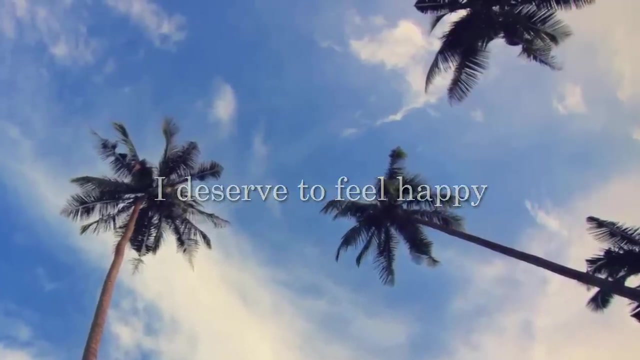 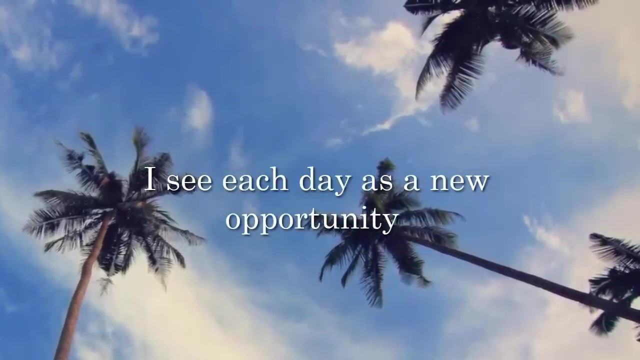 Just put it aside and move on to the next one. So let's begin. I am ready to take on positive changes in my life. I am eager to get more out of life. I deserve to feel happy. I see each day as a new opportunity. 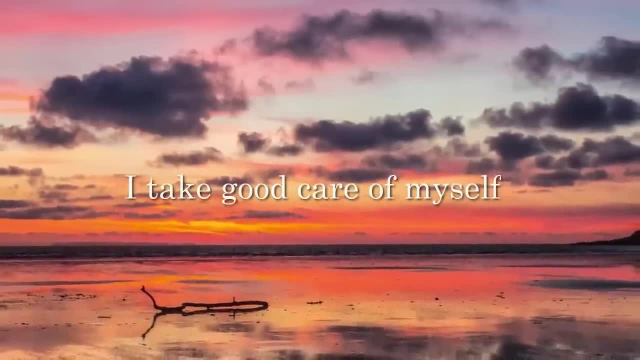 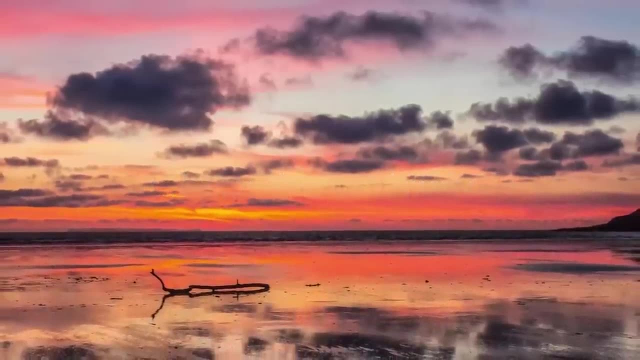 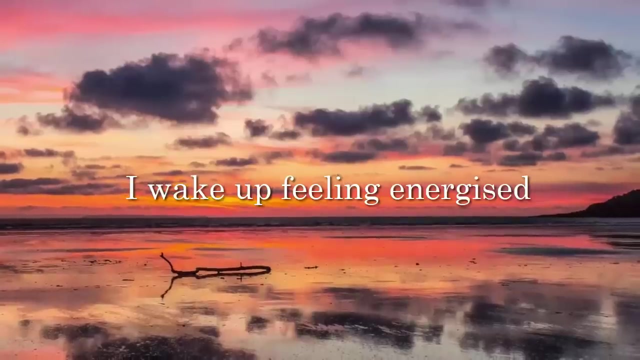 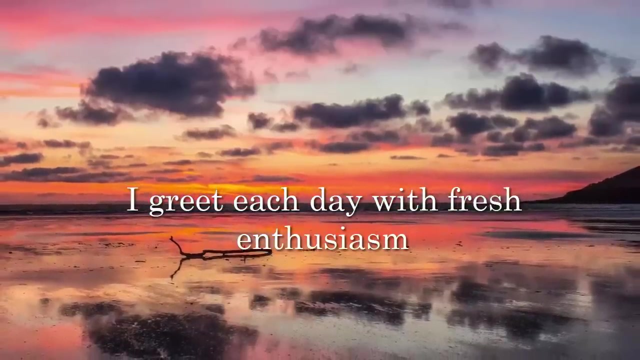 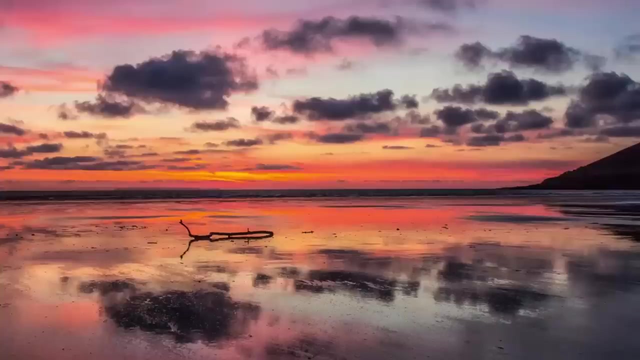 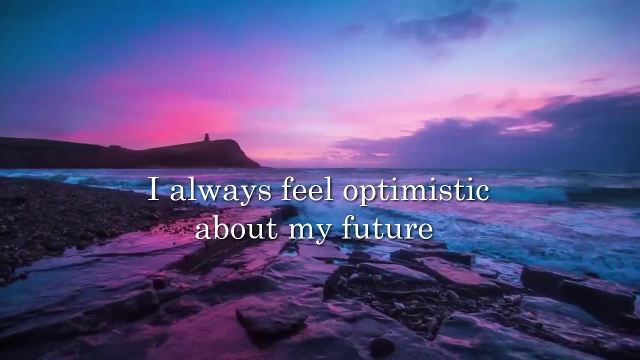 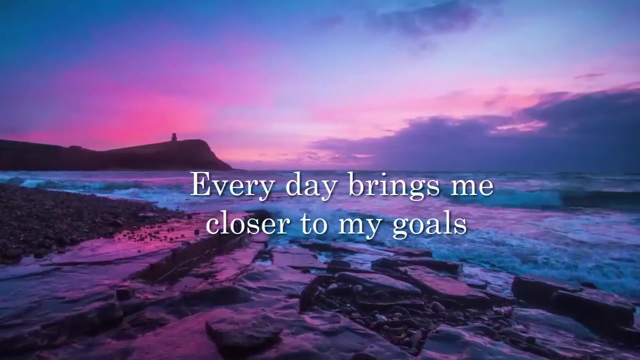 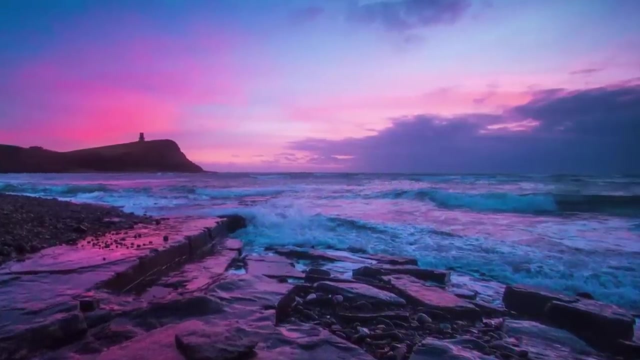 I take good care of myself. I wake up feeling energized. I greet each day with fresh enthusiasm. I am ready to take on positive changes in my life. I always feel optimistic about my future. Every day brings me closer to my goals. 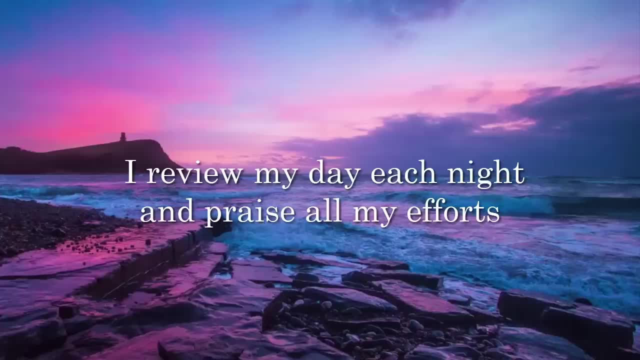 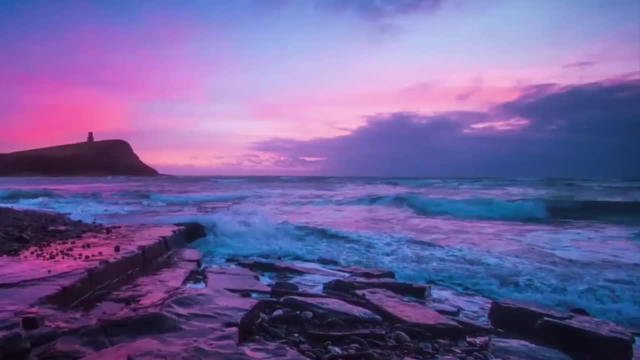 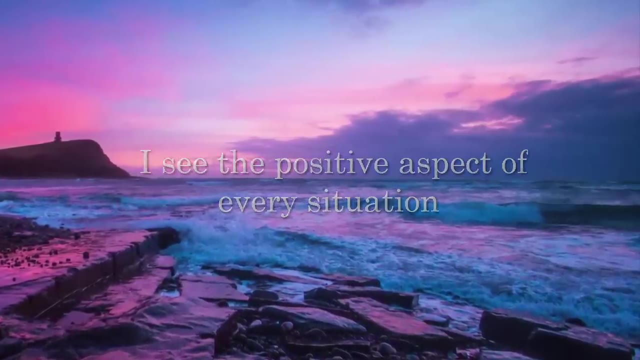 I review my day each night and praise all my efforts. I am ready to take on positive changes in my life. I see the positive aspect of every situation. I am ready to take on positive changes in my life. I create my own world. 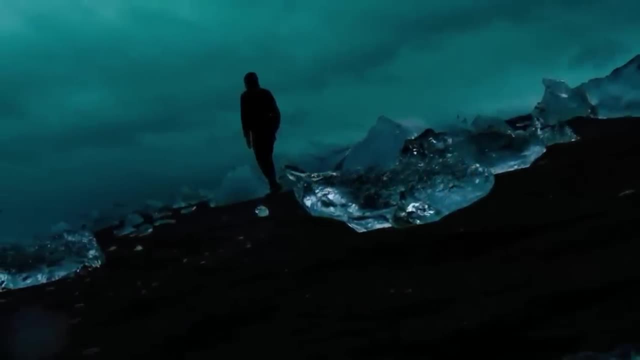 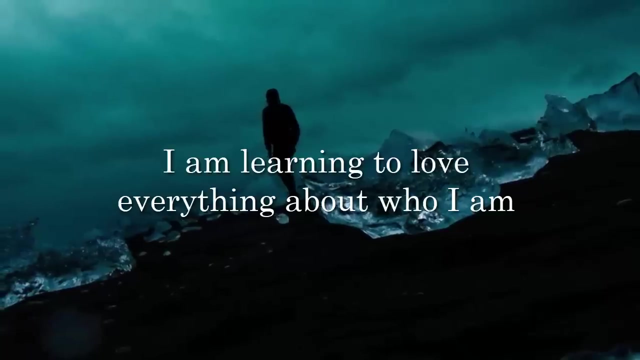 I am ready to take on positive changes in my life. I am learning to love everything about who I am. I am learning to love everything about who I am. I am more of a friend to people I love. I am more willing to take on positive changes in my life. 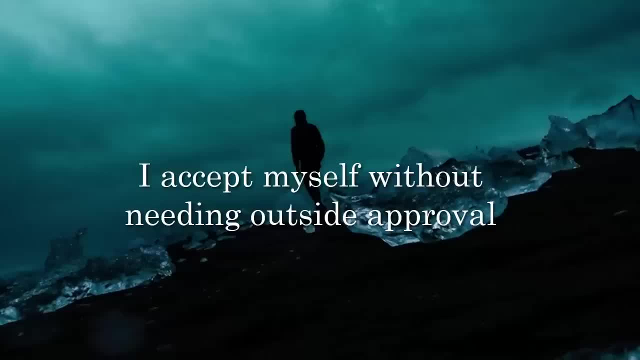 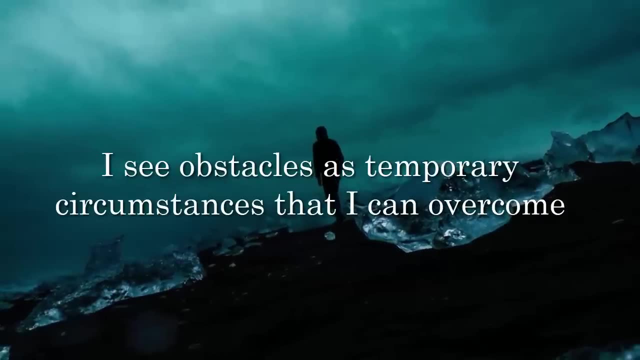 I am ready to learn to be Żywnier than others. I am ready to be a Tomi who screams in the morning. I am ready to improve and pass on all thepertinent spiritual abilities of others. I am ready to take on positive changes in my life. 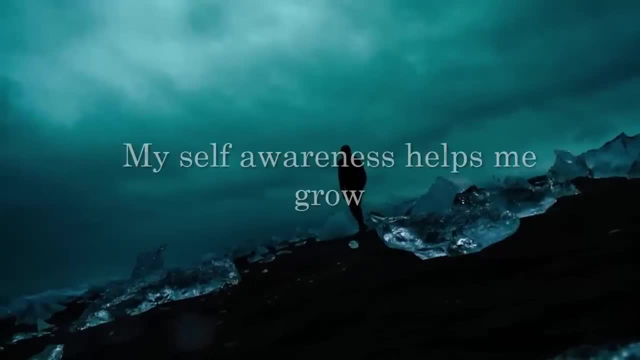 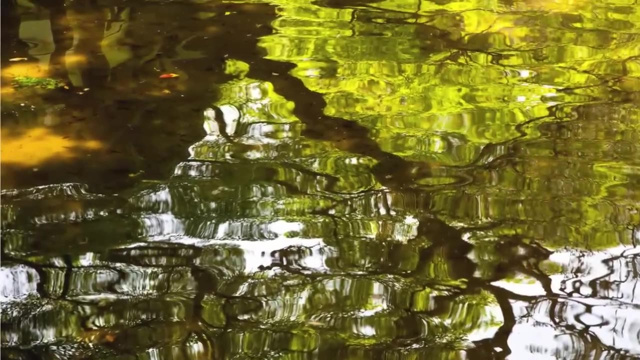 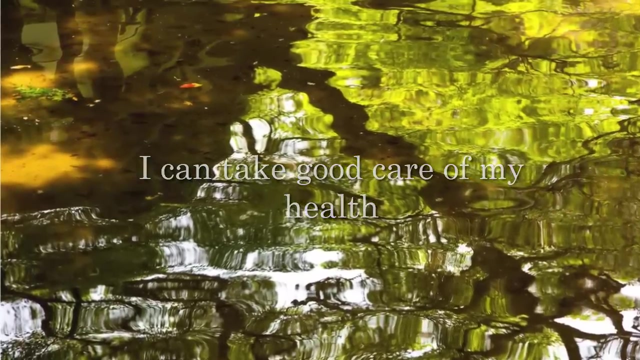 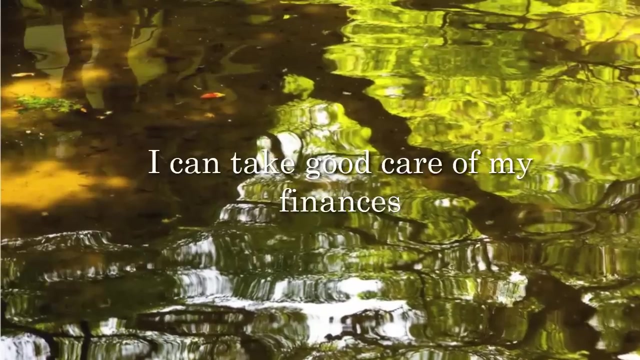 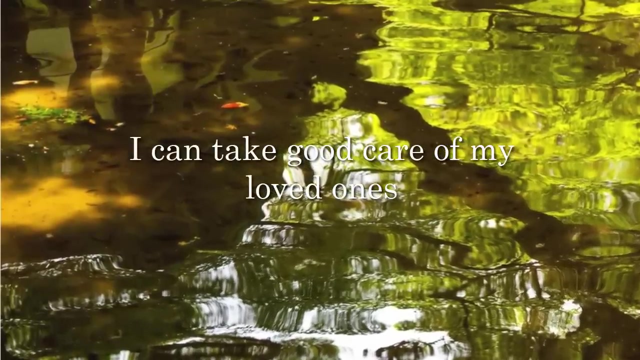 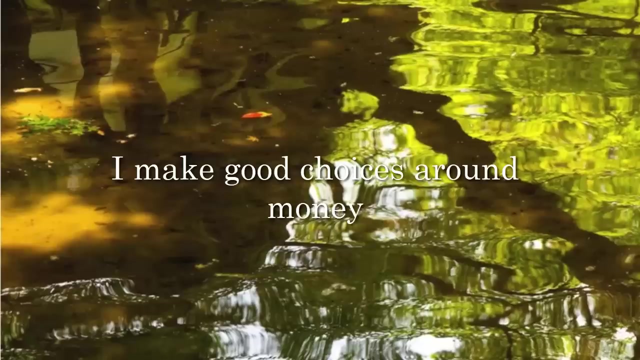 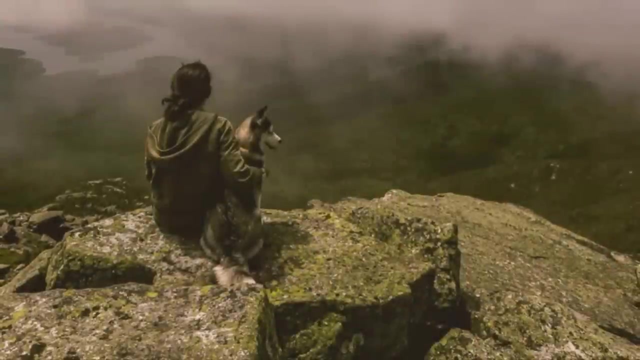 I am constantly doing all kinds of でя arbets. This helps me grow. I can take good care of my health. I can take good care of my finances. I can take good care of my loved ones. I make good choices around money. 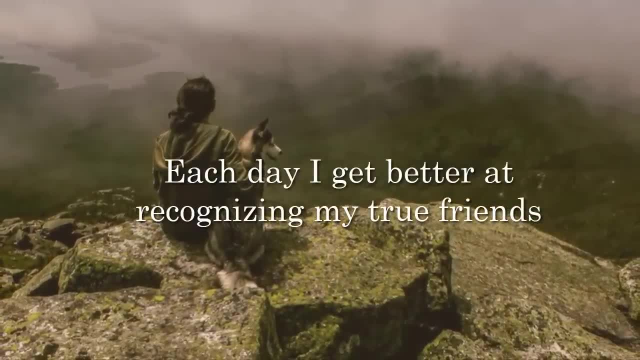 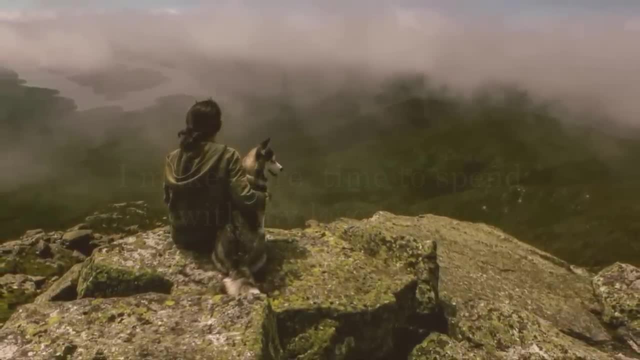 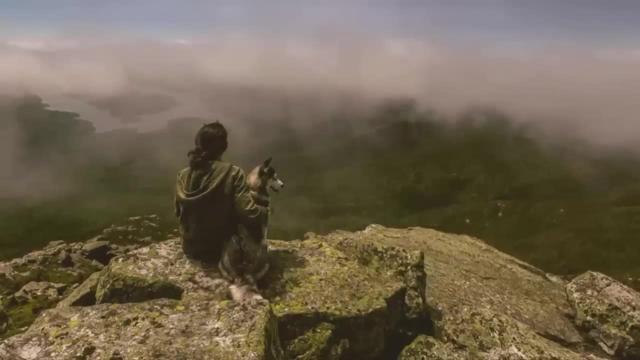 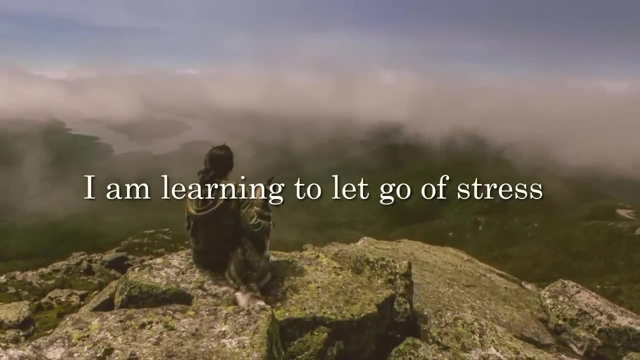 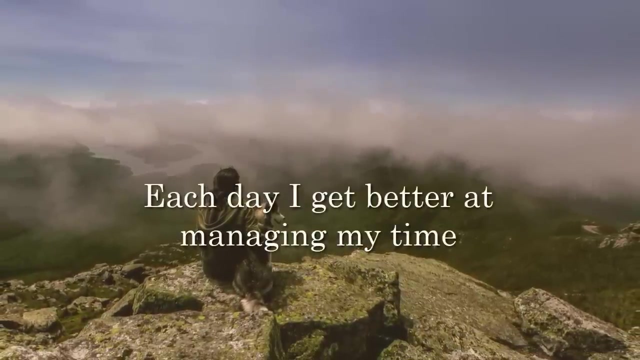 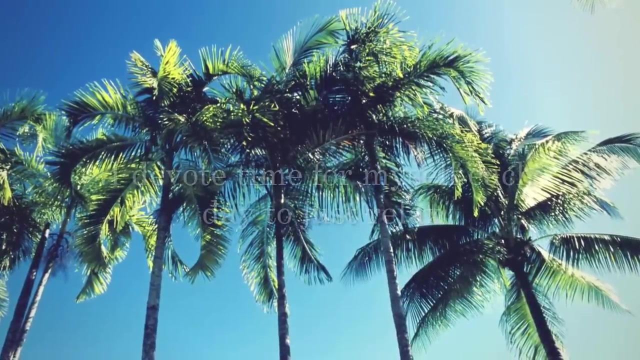 Each day, I get better at recognising my true friends. I make more time for myself. I make more time to spend with my loved ones. I am learning to let go of stress. Each day, I get better at managing my time. I devote time for myself each day. 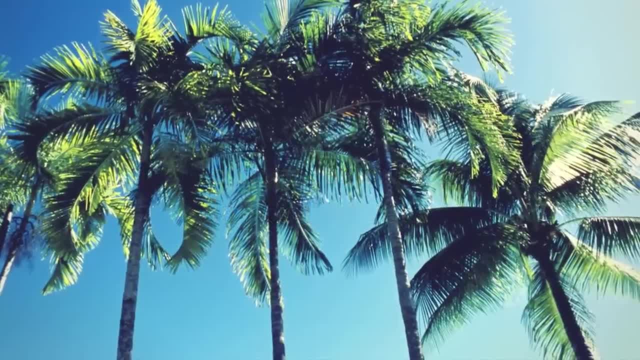 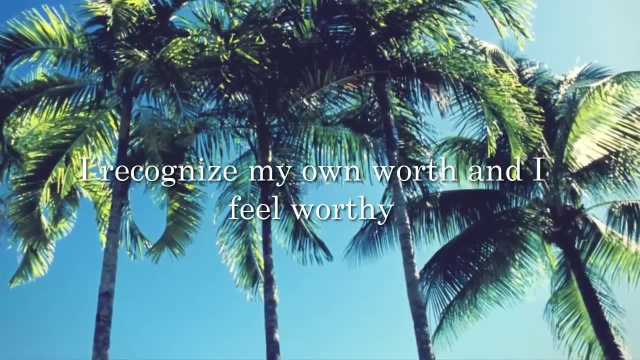 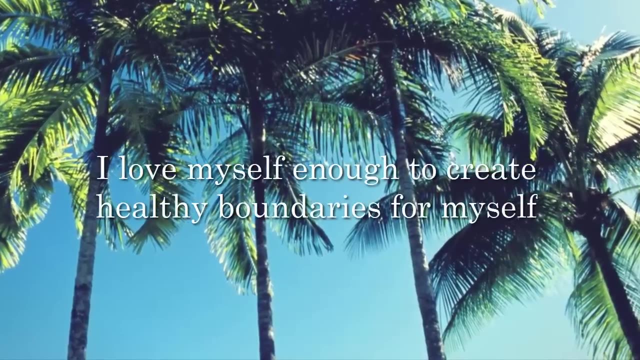 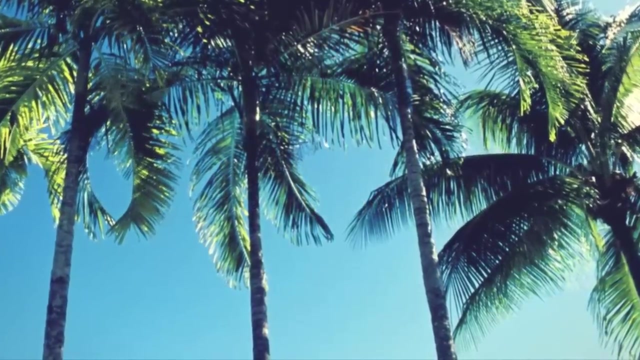 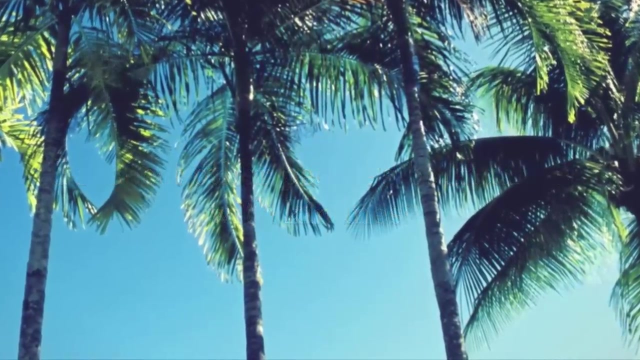 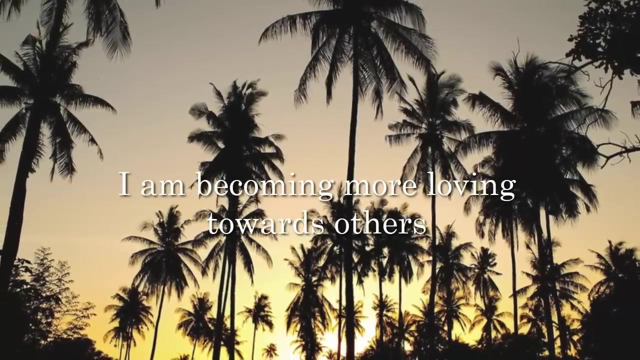 To just relax. I recognise my own worth and I feel worthy. I love myself enough to create healthy boundaries for myself. I respect other people's boundaries with kindness. I am becoming more loving towards others. I am opening myself up to receive love. 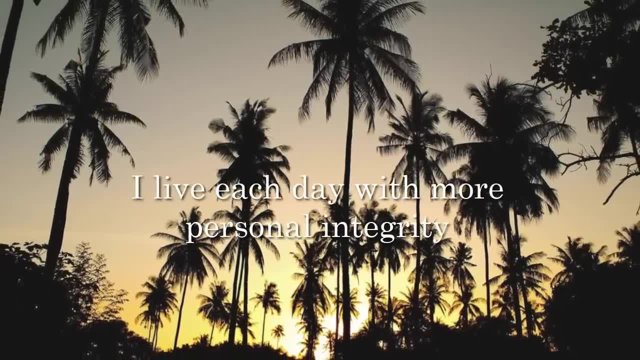 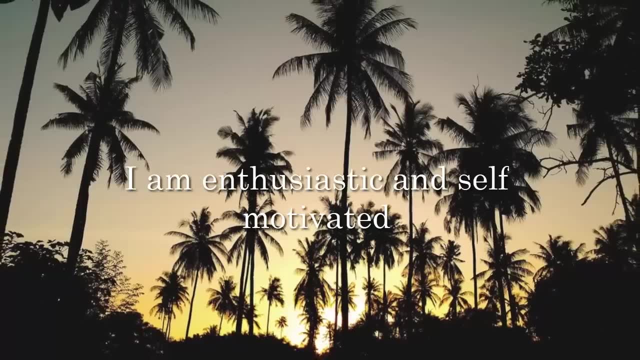 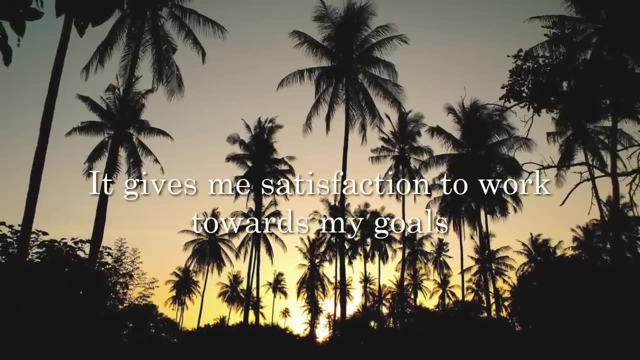 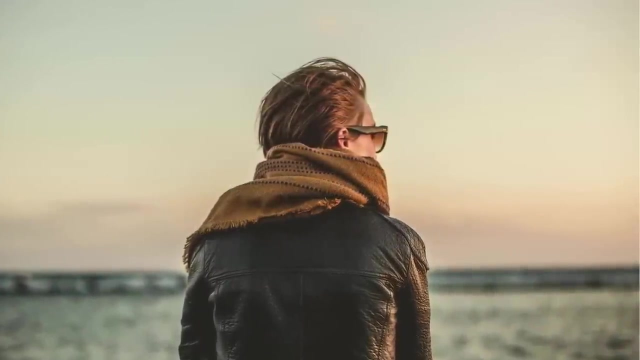 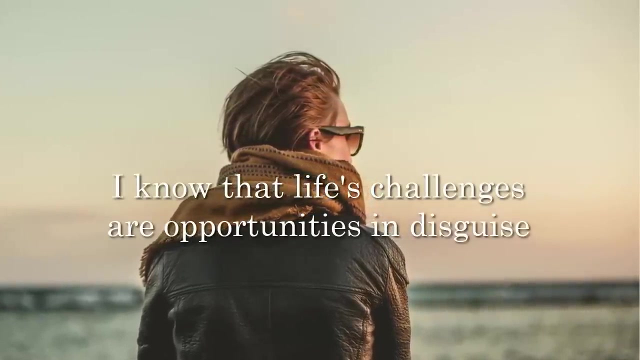 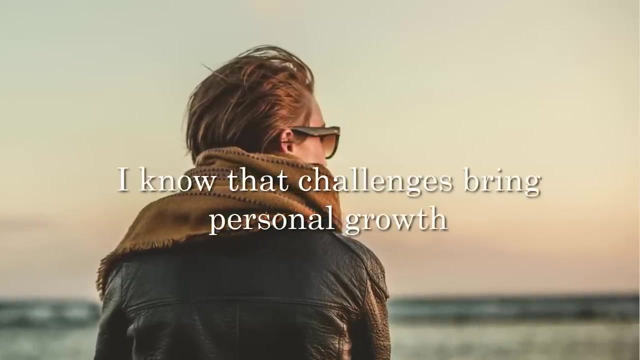 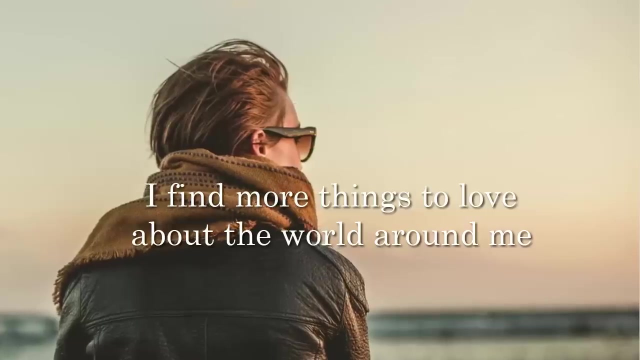 I live each day with more personal integrity. I am enthusiastic and self-motivated. It gives me great satisfaction to work towards my goals. I know that life's challenges are opportunities in disguise. I know that challenges bring personal growth. I find more things to love about the world around me. 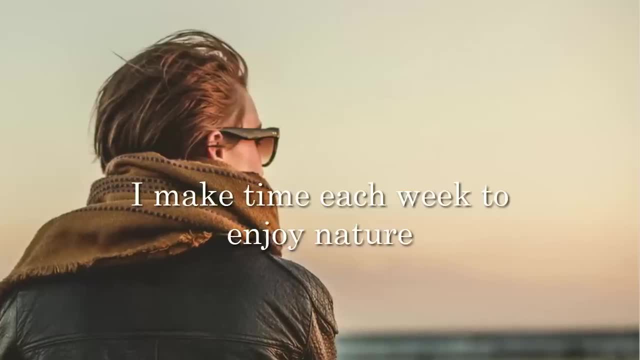 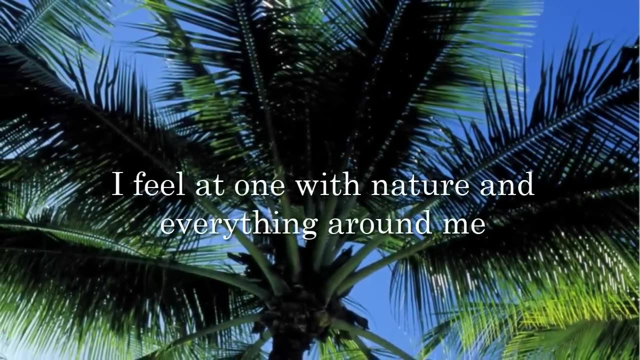 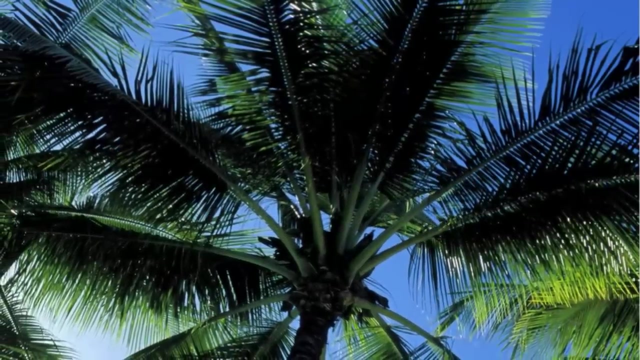 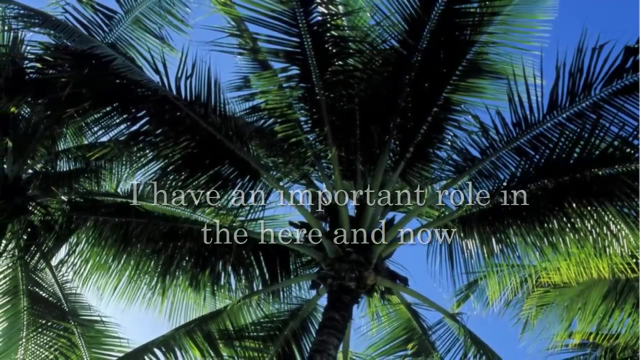 I make time each week to enjoy nature. I feel at one with nature. I feel at one with nature. I feel at one with nature and everything around me. I have an important role in the here and now. I live life with more passion. 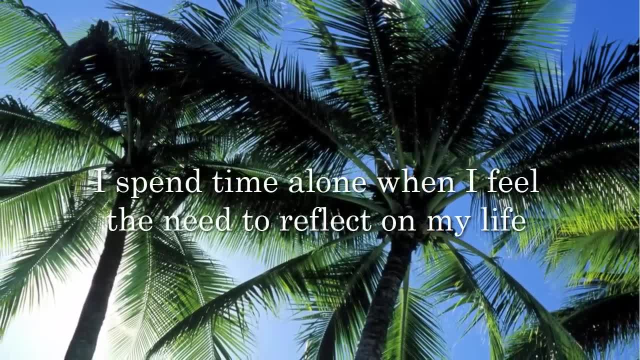 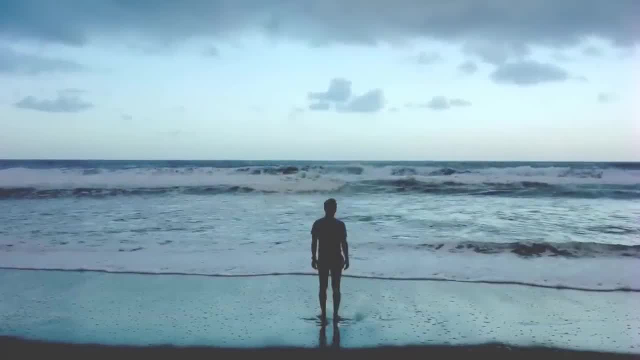 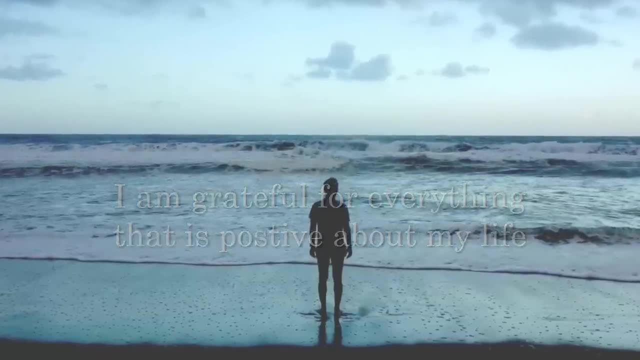 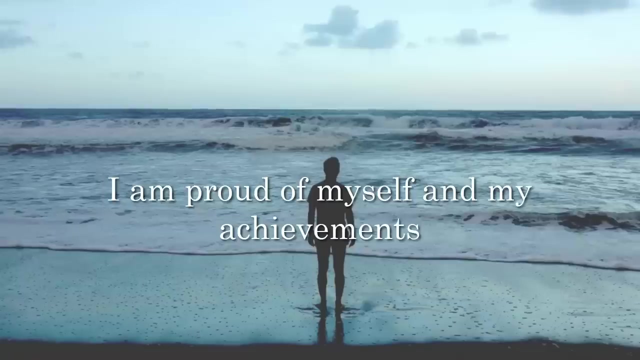 I spend time alone when I feel the need. I spend time alone when I feel the need to reflect on my life. I am grateful for everything that is positive about my life. I am proud of myself and my achievements. I am proud of myself and my achievements. 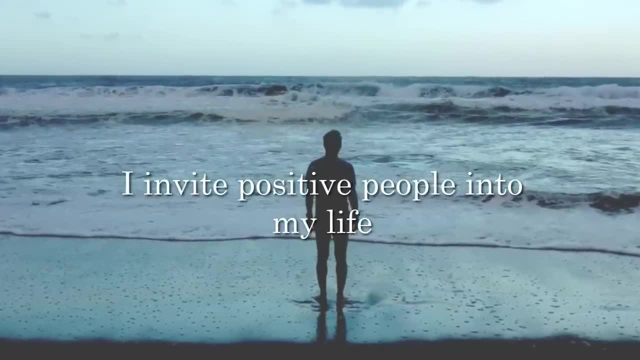 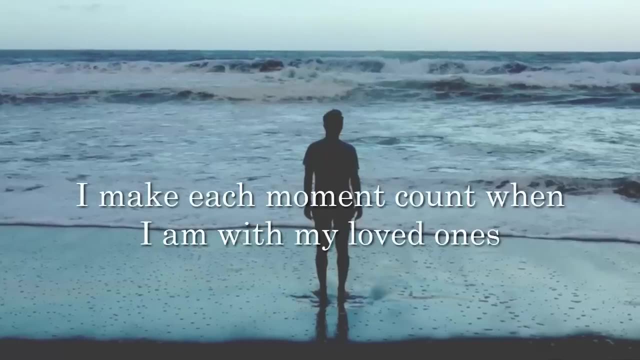 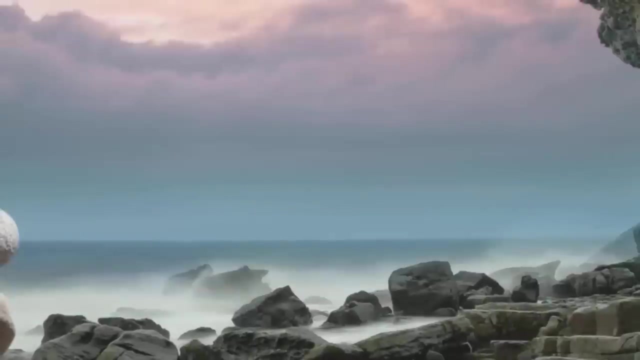 I invite positive people into my life. I welcome positive people to change my life. I make each moment count. when I'm with my loved one's, I check in with myself to balance my emotions. I'm cool with my heart. I let go of other people's opinions of my life and my brushes. 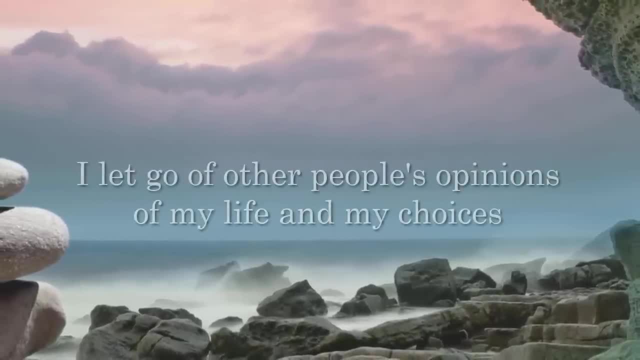 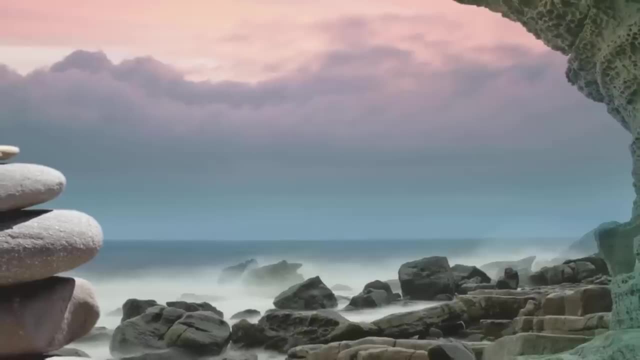 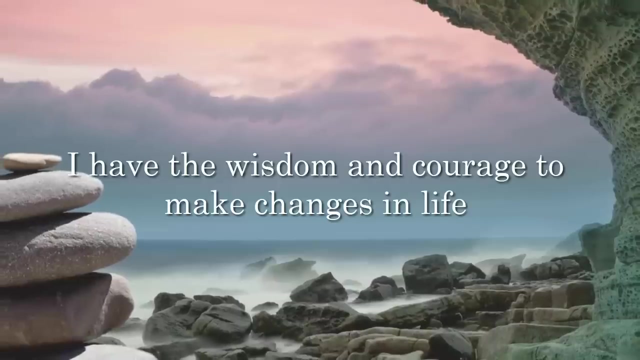 I love calm, different processes. I'm wonderful about how I've been doing something from the start: My worth, reason, my identity, my passion, myink, you conception, my More ability than simpler. I have the wisdom and courage to make changes in life. 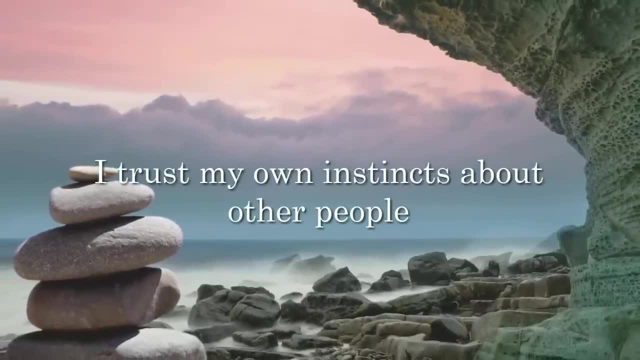 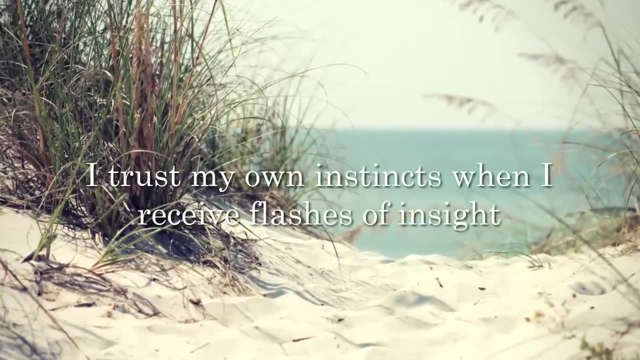 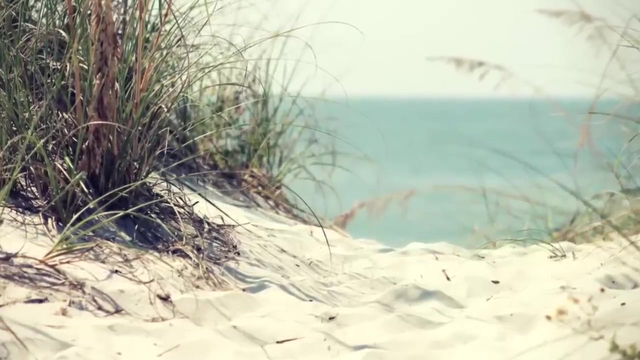 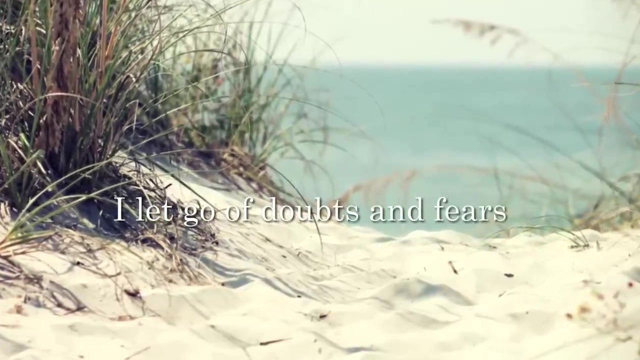 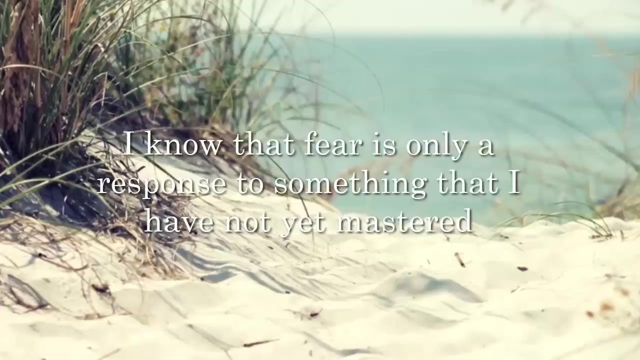 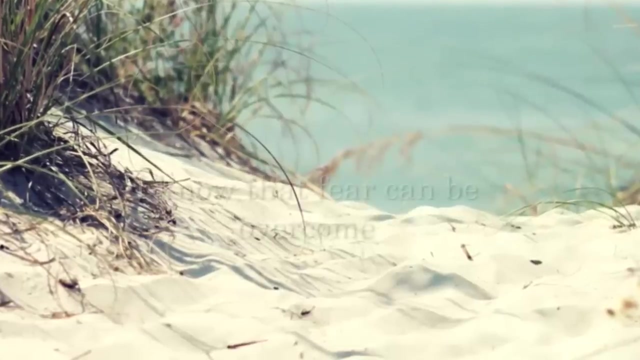 I trust my own instincts about other people. I trust my own instincts when I receive flashes of insight. I let go of doubts and fears. I know that fear is only a response to something I have not yet mastered. I know that fear is only a response to something I have not yet mastered. 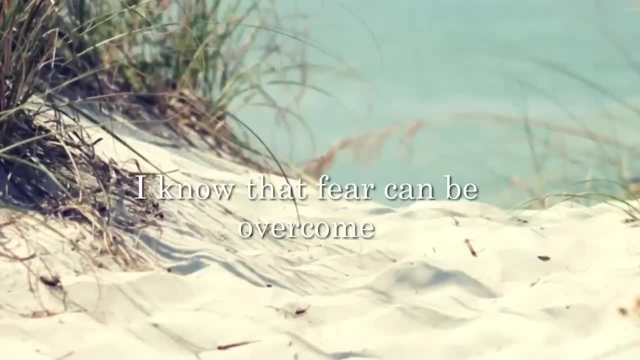 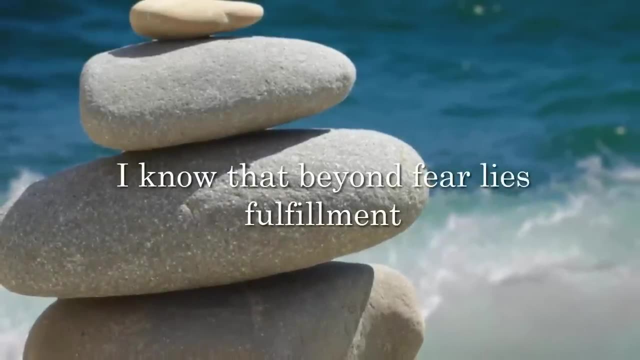 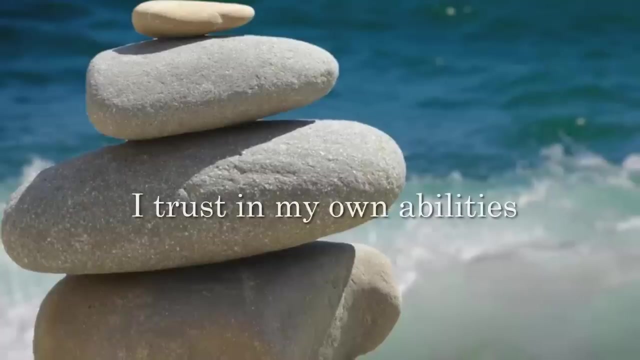 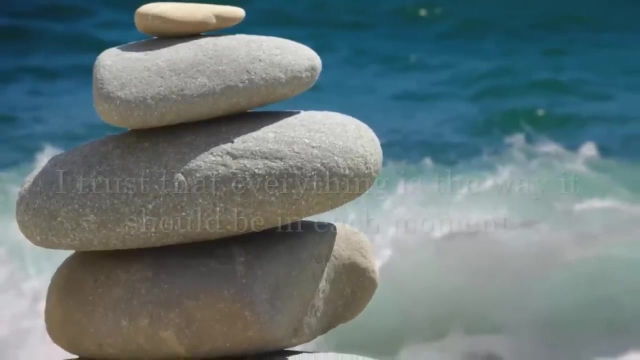 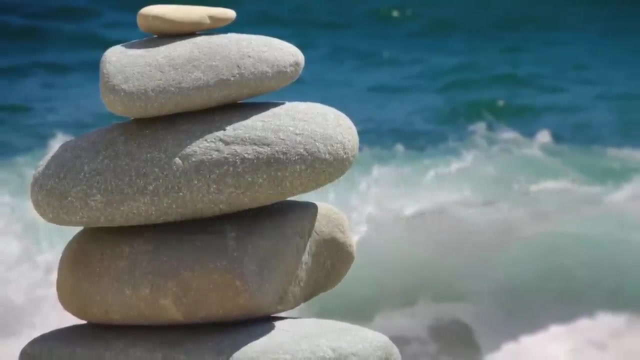 I know that fear can be overcome. I know that beyond fear lies fulfillment. I trust in my own abilities. I trust that everything is the way it should be in each moment. I know that I don't yet have all the answers and that it's okay. 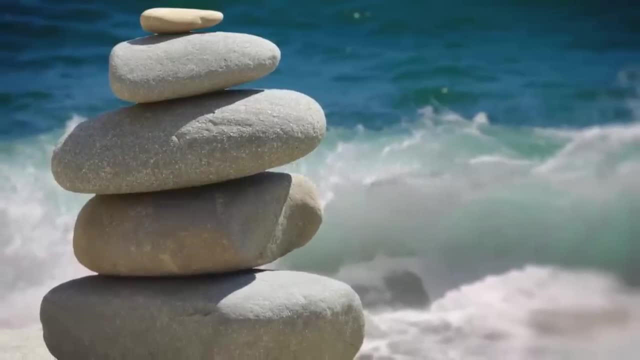 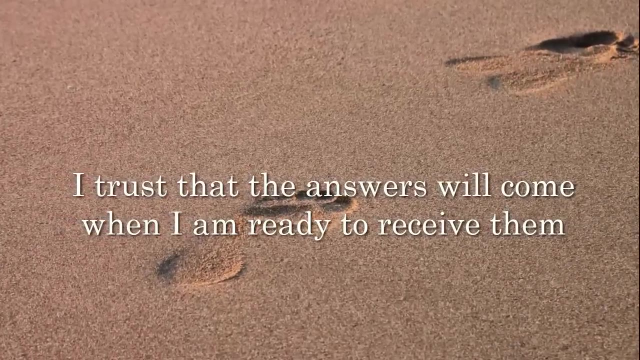 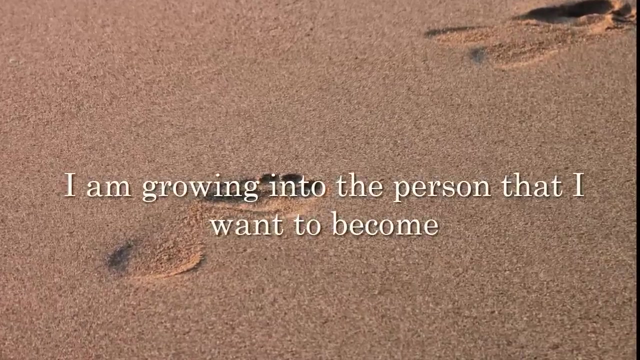 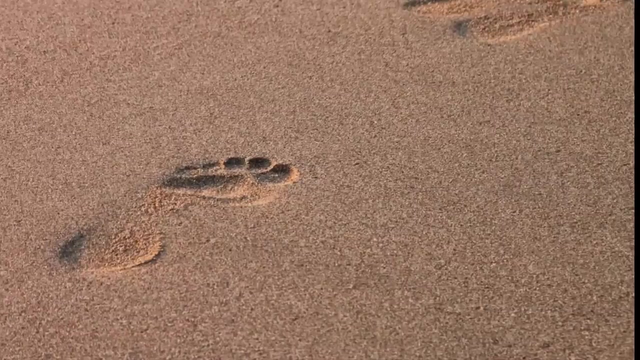 I trust that the answers will come when I'm ready to receive them. I trust that the answers will come when I'm ready to receive them. I'm growing into the person I want to become. I trust that I can take this Maison. I see the ways to improve and have some self-improvement. 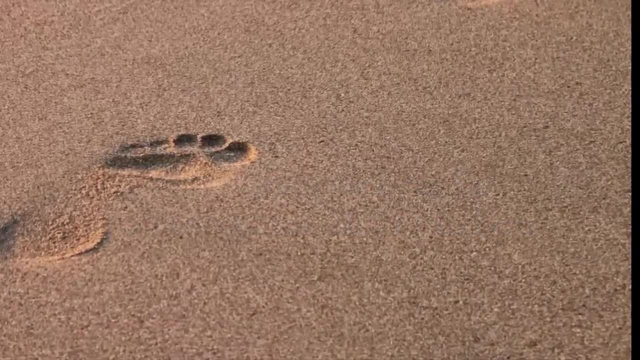 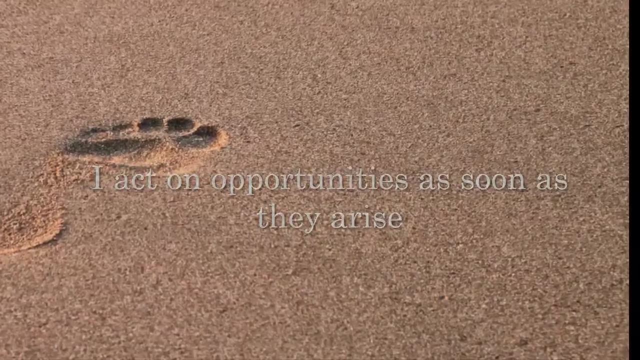 I see the end of the road looking fresh in the sûr gl者's eyes, starting at his previous flat. again, I see opportunities for improvement, for, whether I am happy or not, I see opportunities for advancement all around me. I know the truth. 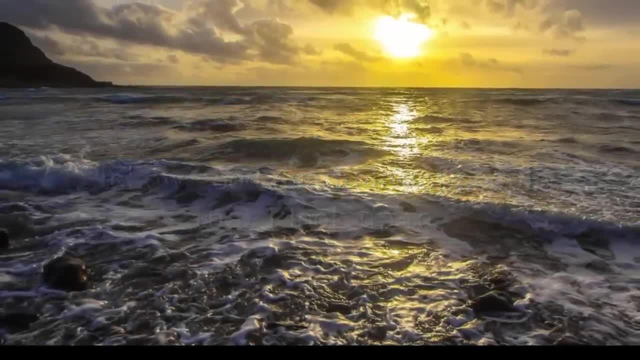 I see opportunities for advancement. I act on opportunities as soon as they arise. I see opportunities for advancement all around me. I act on opportunities as soon as they arise. 하고 widha, Get our hearts tuned together Or get answers online, or follow my workshops. Are there any good examples to follow? I see them all around me. 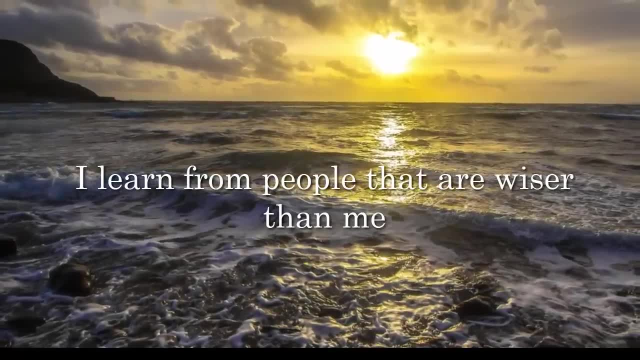 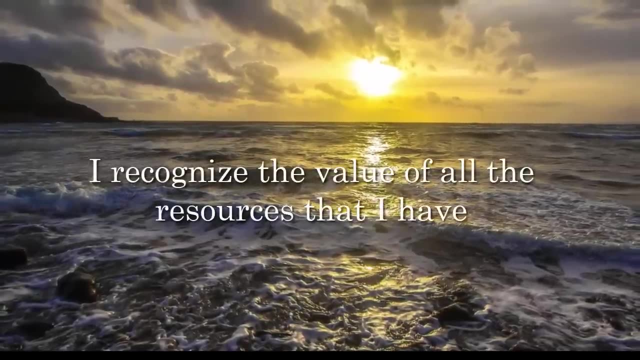 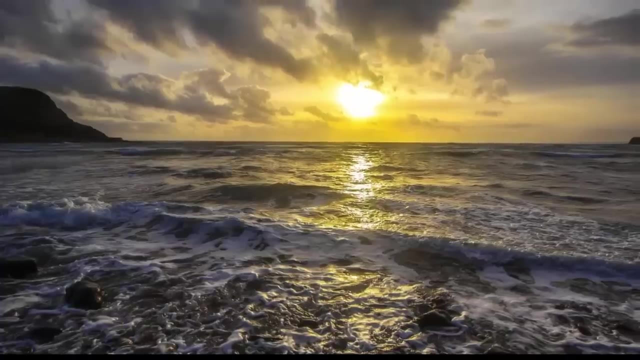 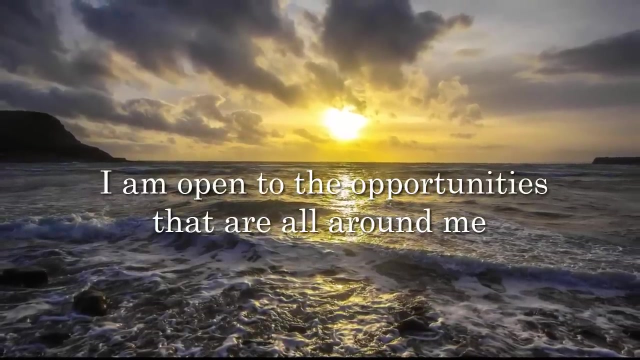 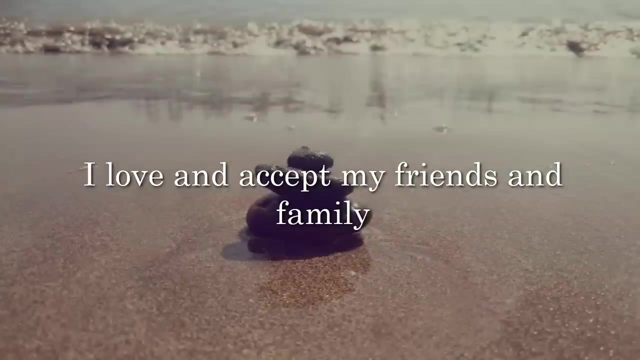 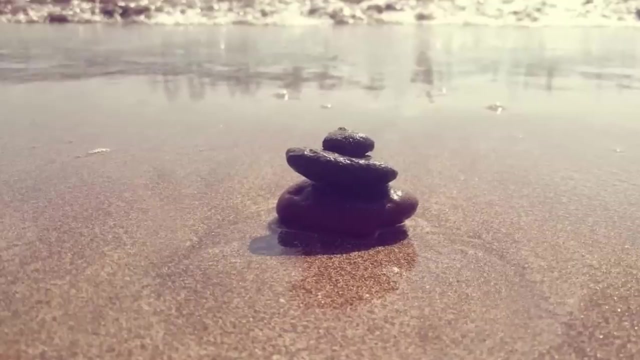 I learn from people that are wiser than me. I recognise the value of all the resources that I have. I am open to the opportunities that are all around me. I love and accept my friends and family. I love and accept my close companions. 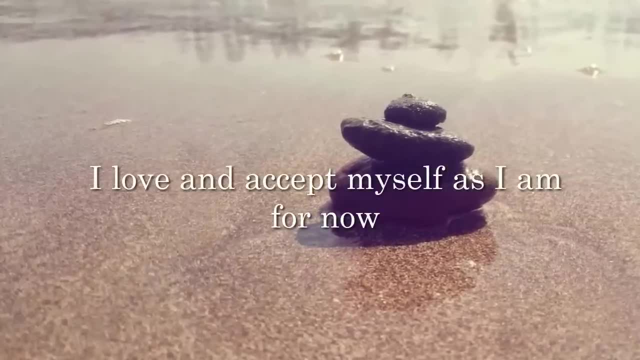 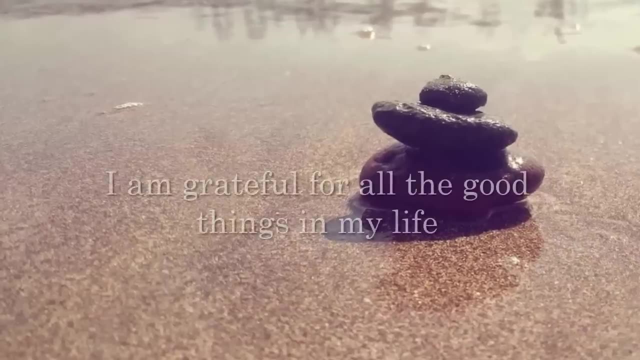 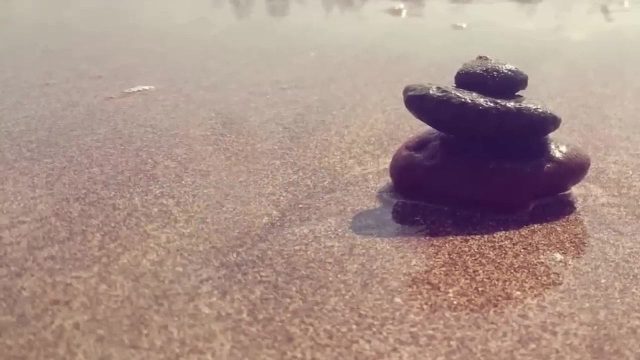 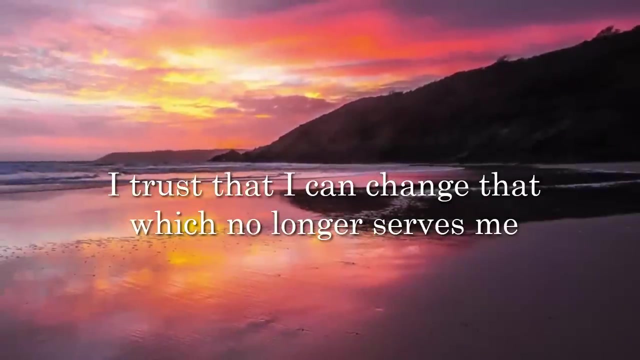 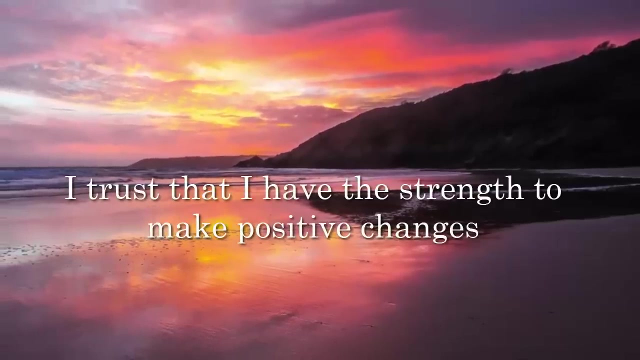 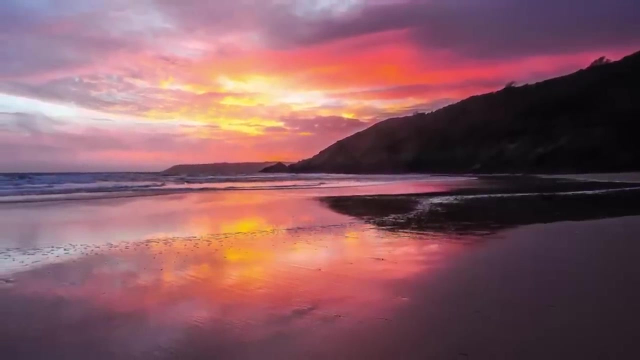 I love and accept myself as I am. for now, I am grateful for all the good things in my life. I trust that I can change that which no longer serves me. I trust that I have the strength to make positive changes. I let go of past disappointments. 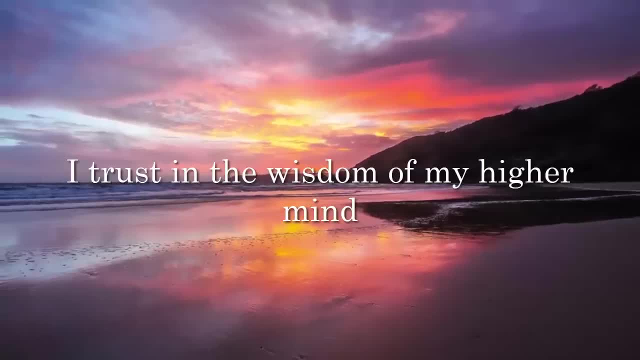 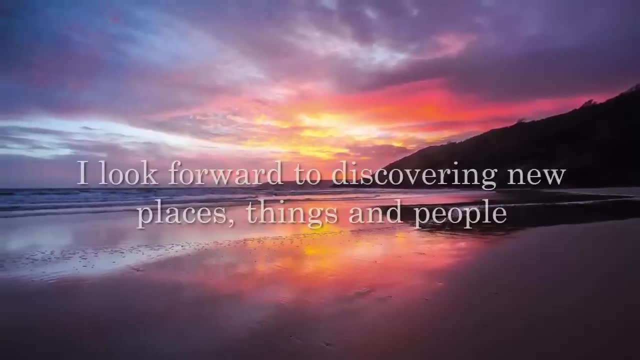 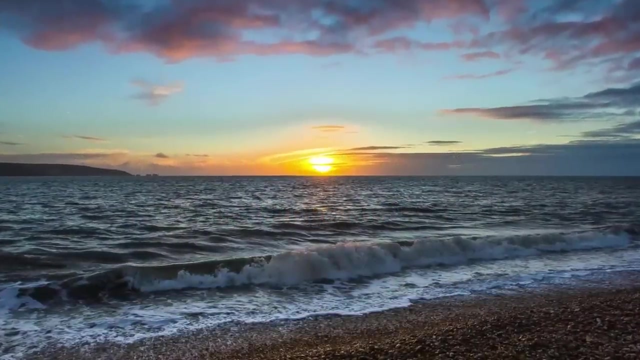 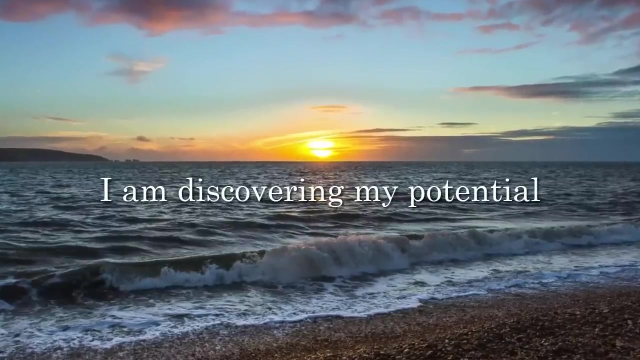 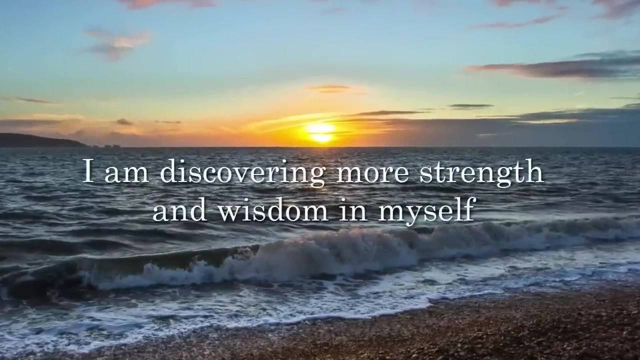 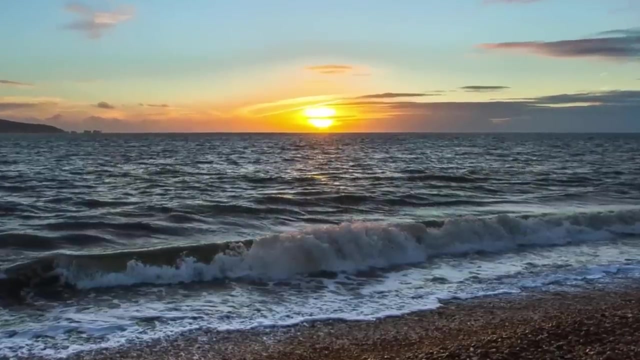 I trust in the wisdom of my higher mind. I look forward to discovering new places, things and people. I am discovering my potential. I am discovering more strength and wisdom in myself. I am determined to achieve whatever I hold in my mind's eye. 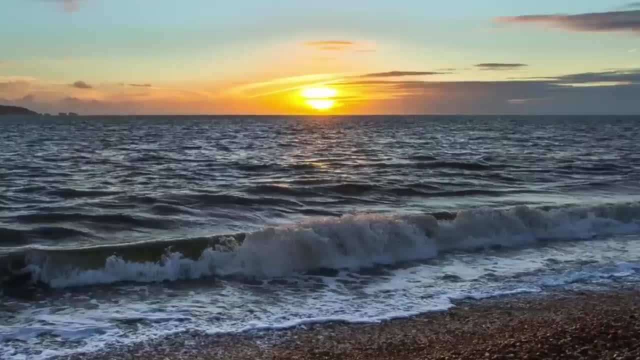 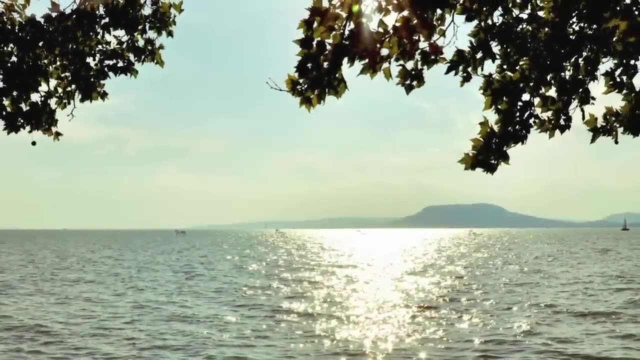 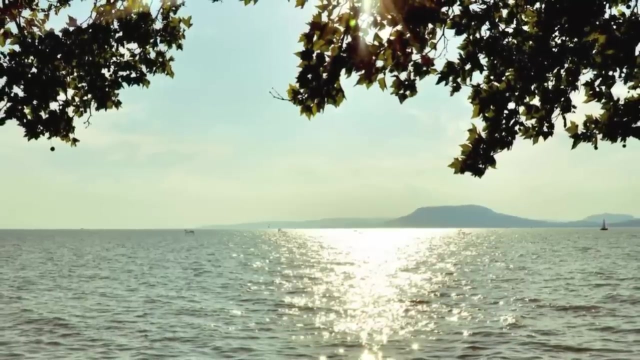 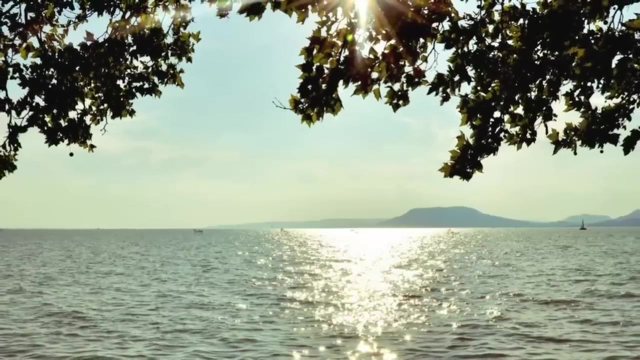 I am determined to achieve whatever I hold in my mind's eye, And so it is. My words become the truth. The next part of this audio is the same affirmations, replaying a few more times. You can just relax while listening passively. 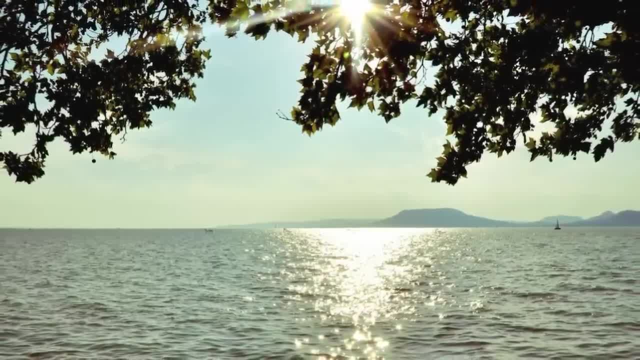 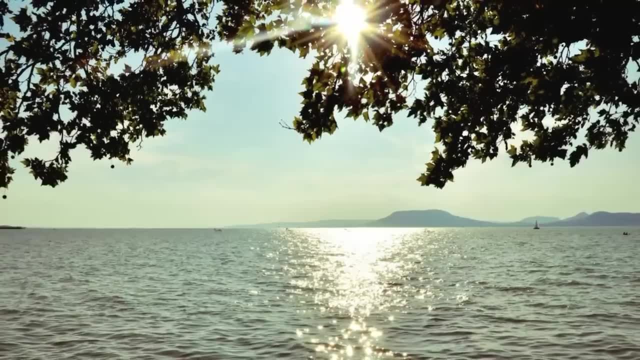 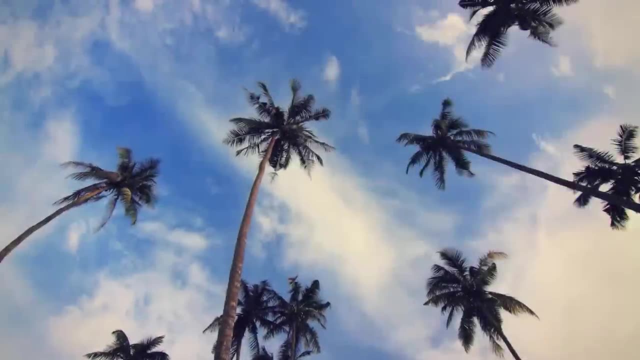 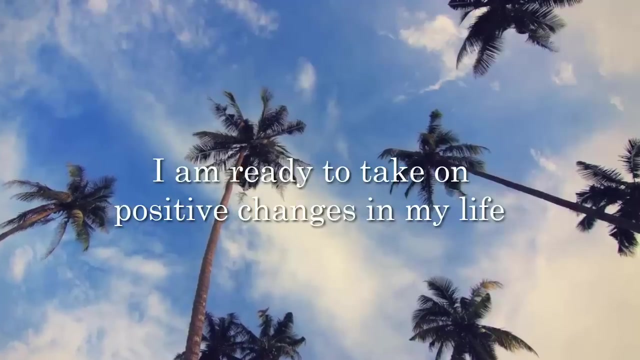 Or, if you would like to, you can go to sleep And you can absorb them a little more, Or you can absorb them a little more into your subconscious. It's your choice And I wish you the best. I am ready to take on positive changes in my life. 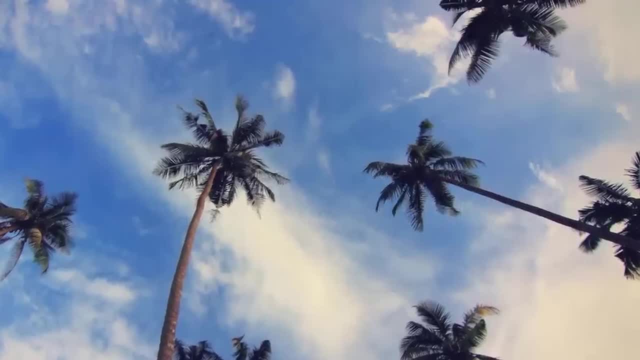 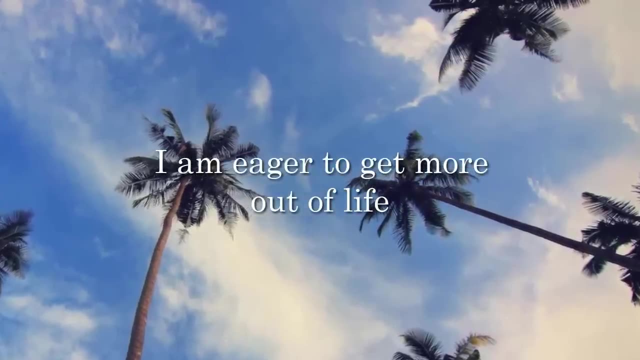 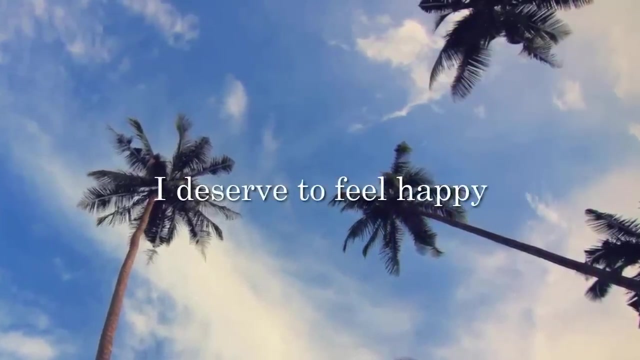 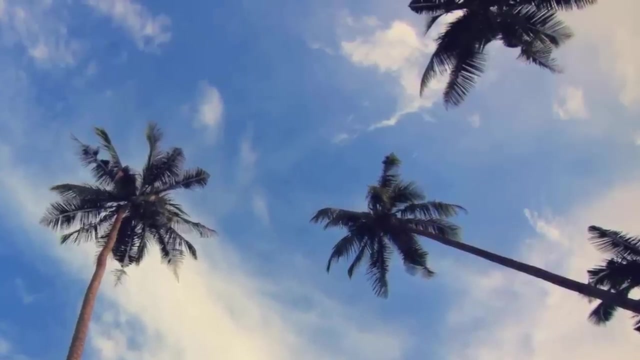 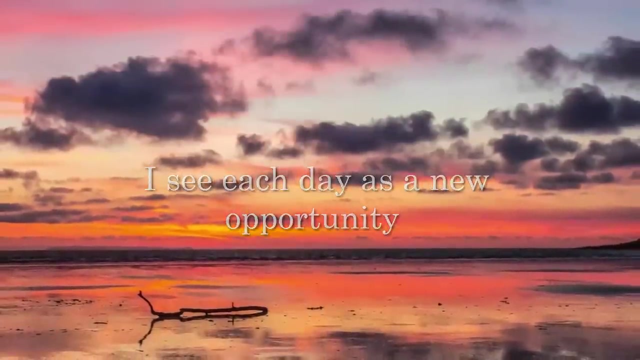 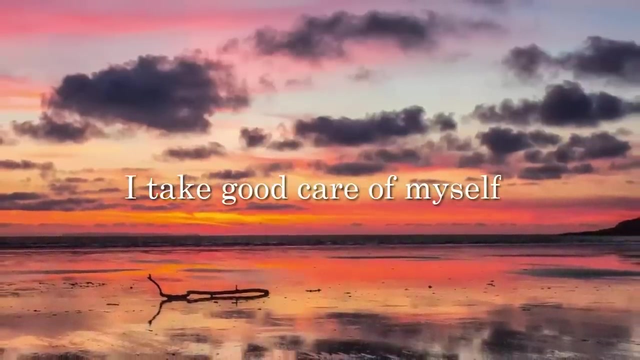 I am ready to take on positive changes in my life. I am ready to take on positive changes in my life. I am eager to get more out of life. I deserve to feel happy. I see each day as a new opportunity. I take good care of myself. 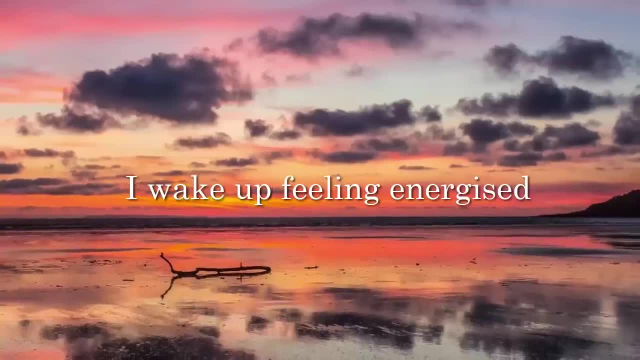 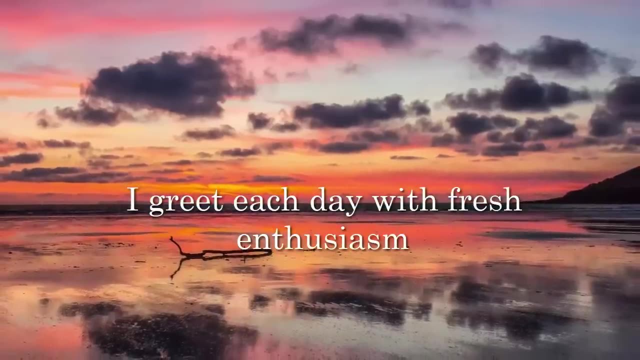 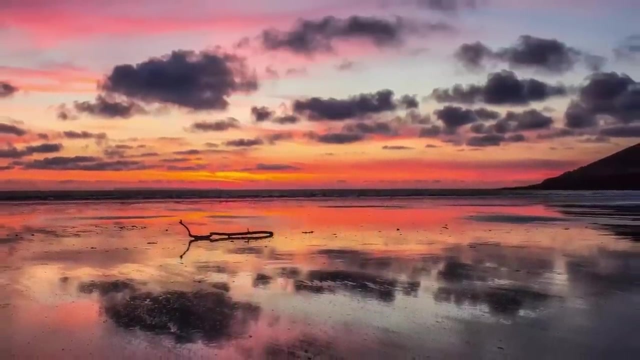 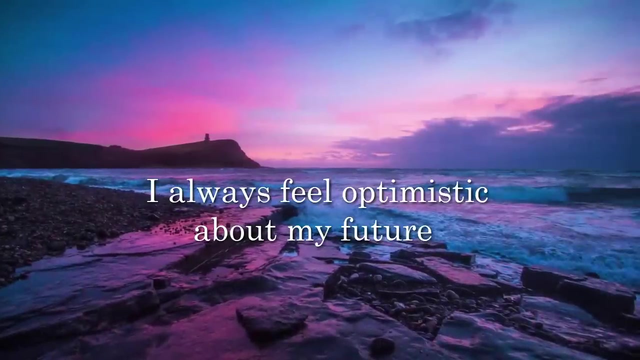 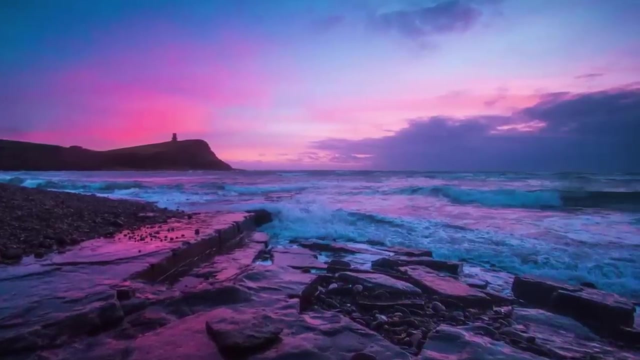 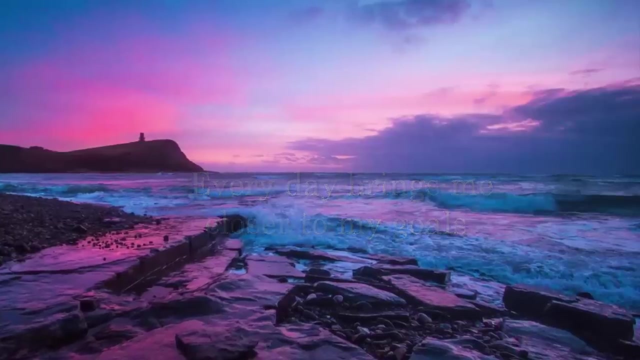 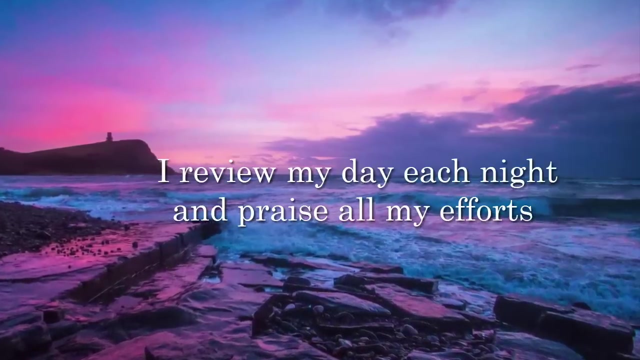 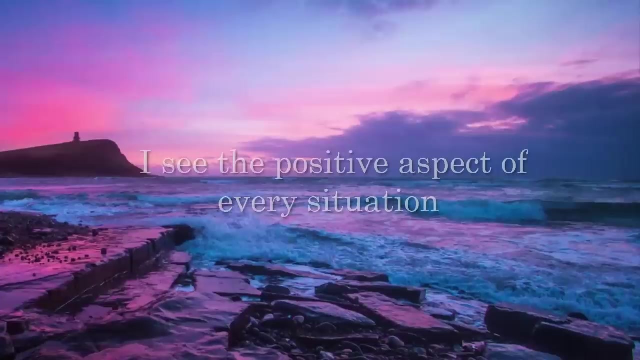 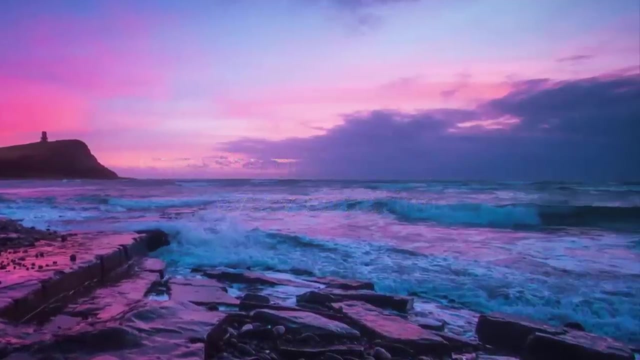 I wake up feeling energized. I greet each day with fresh enthusiasm. I always feel optimistic about my future. Every day brings me closer to my goals. I review my day each night and praise all my efforts. I see the positive aspect of every situation. 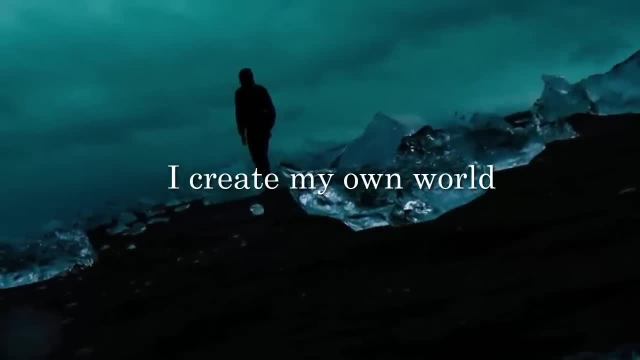 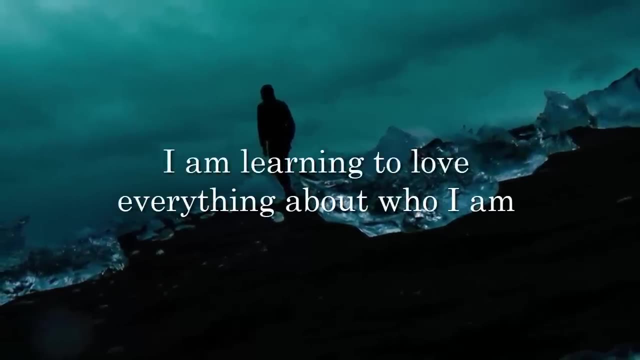 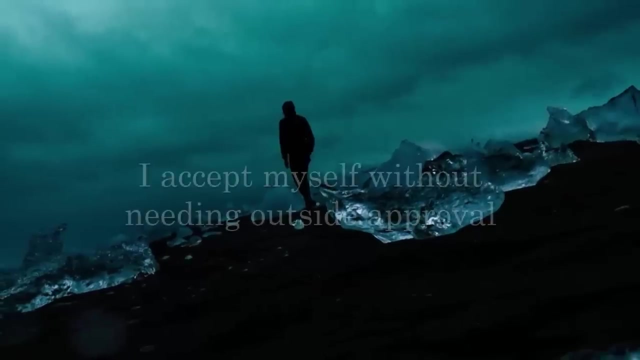 I create my own world. I am learning to love everything about who I am. I accept myself without needing anything. I know every step of the way I am living my life. I am learning to love everything about who I am. I am learning to love everything about who I am. 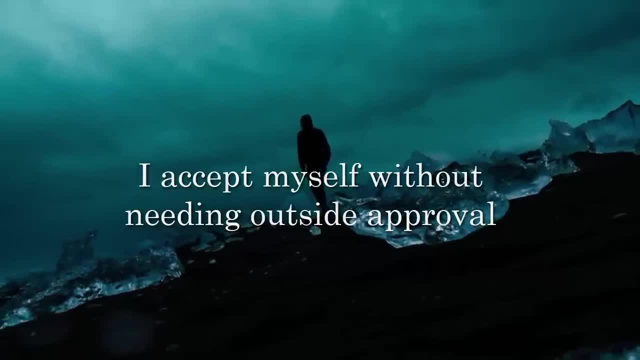 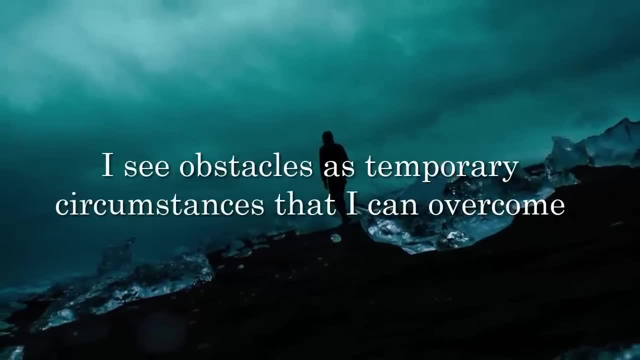 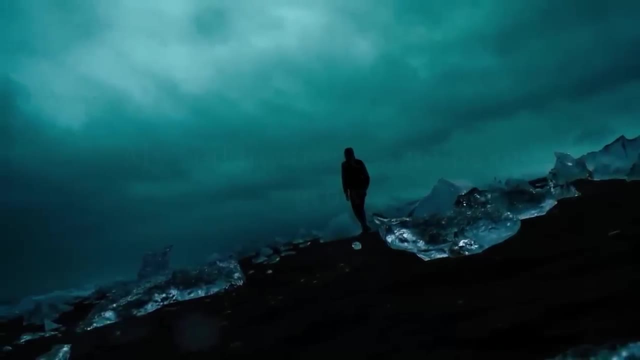 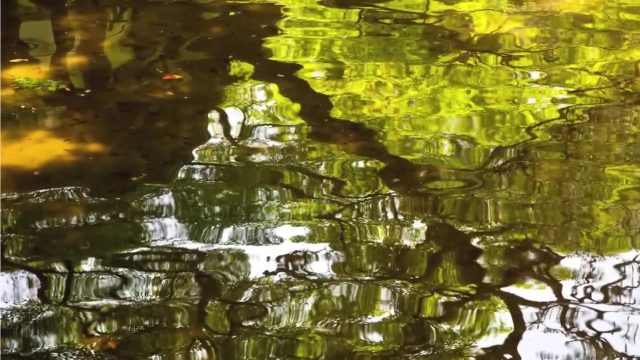 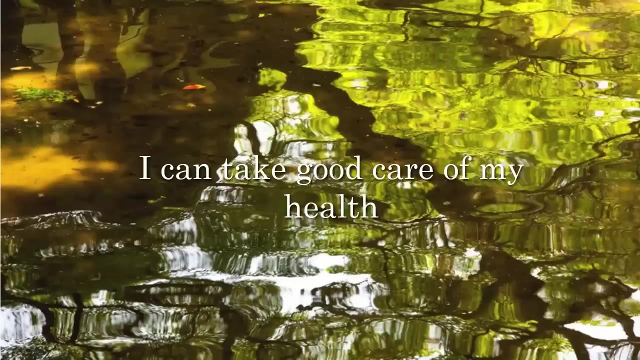 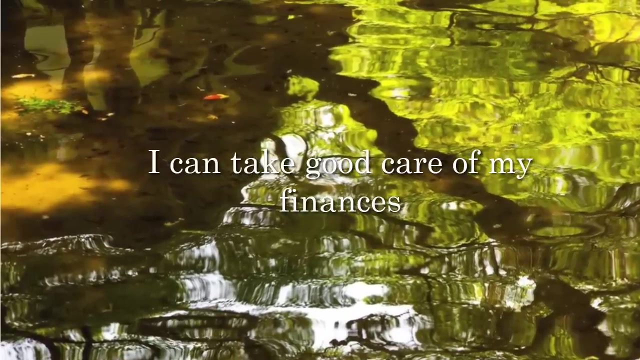 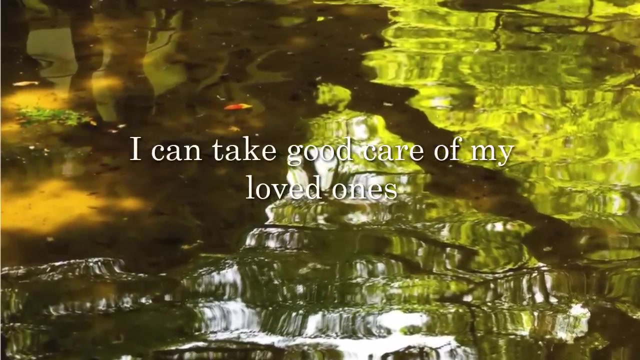 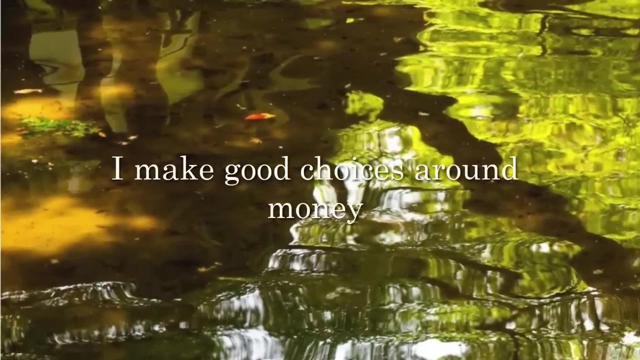 outside approval. I see obstacles as temporary circumstances that I can overcome. My self-awareness helps me grow. I can take good care of my health. I can take good care of my finances. I can take good care of my loved ones. I make good choices around money. 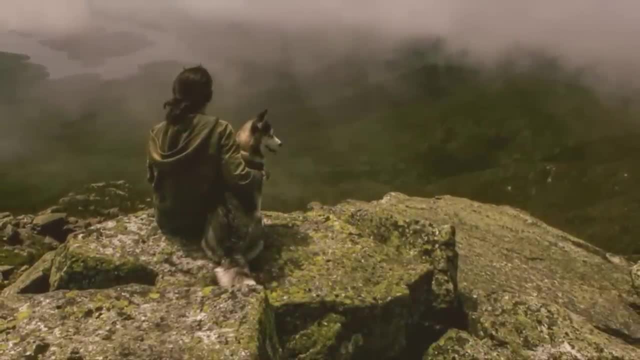 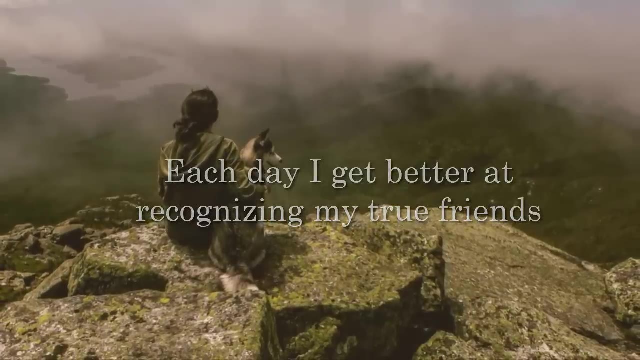 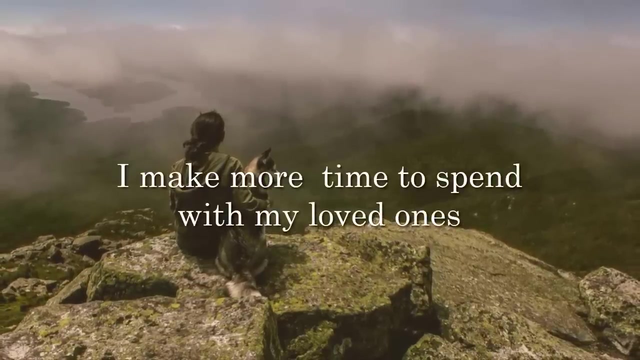 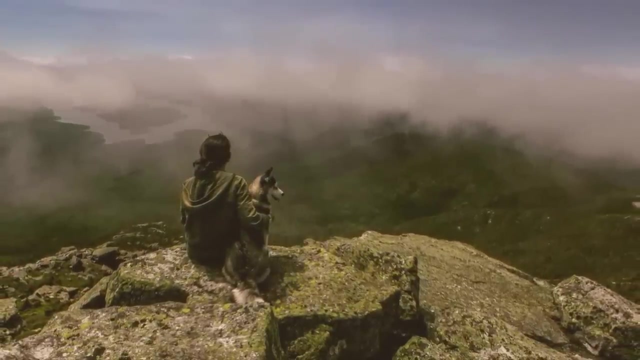 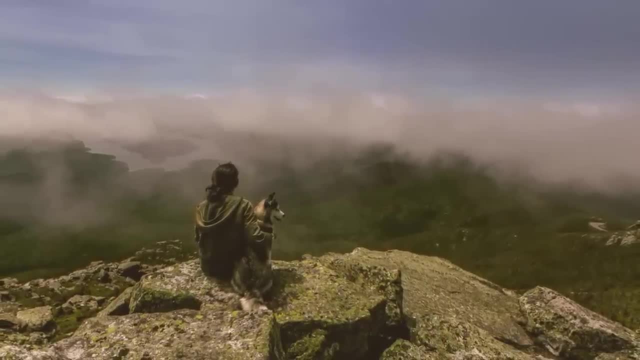 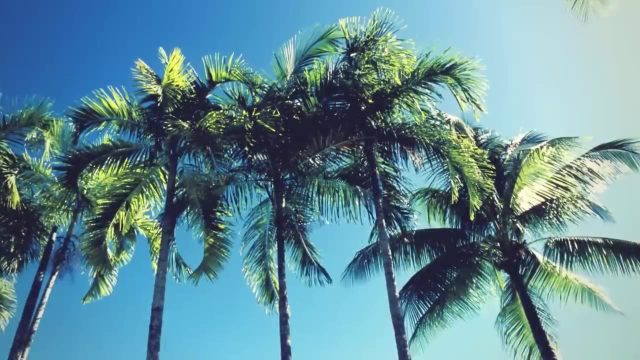 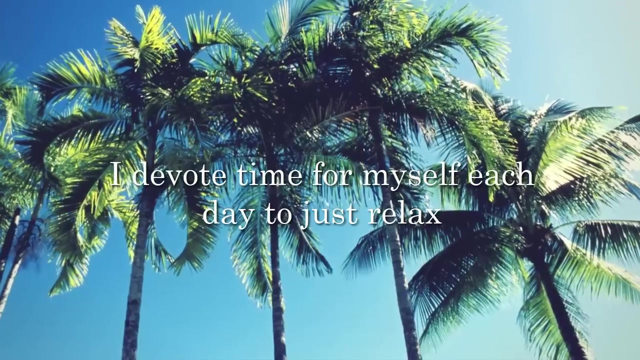 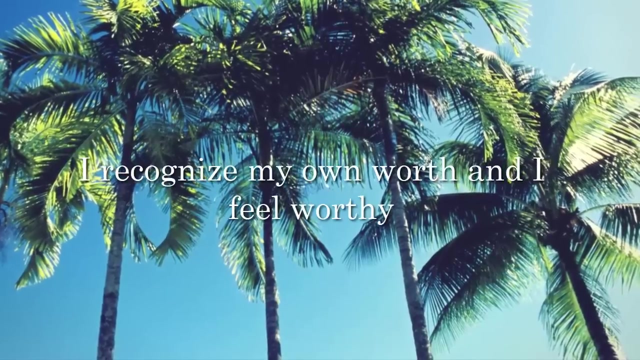 Each day I get better at managing my time. Each day I get better at managing my time. I devote time for myself each day to just relax. I recognise my own worth and I feel worthy. I love myself enough to create healthy boundaries for myself. 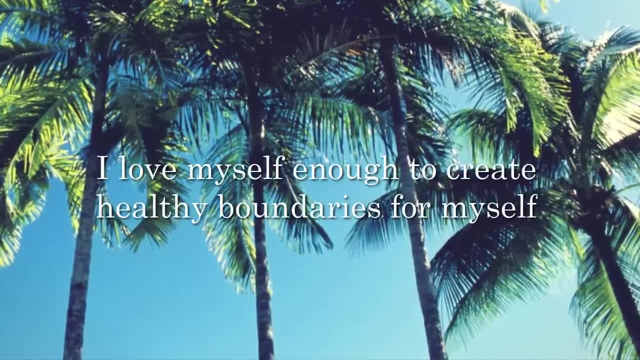 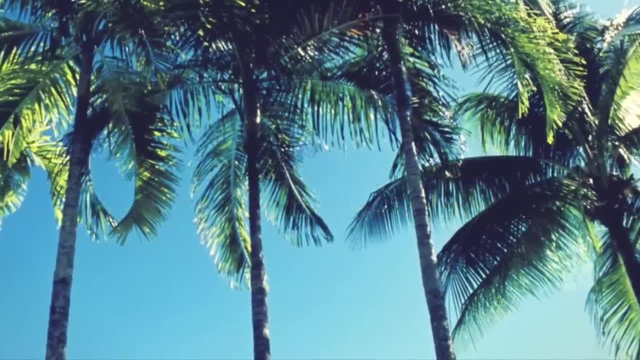 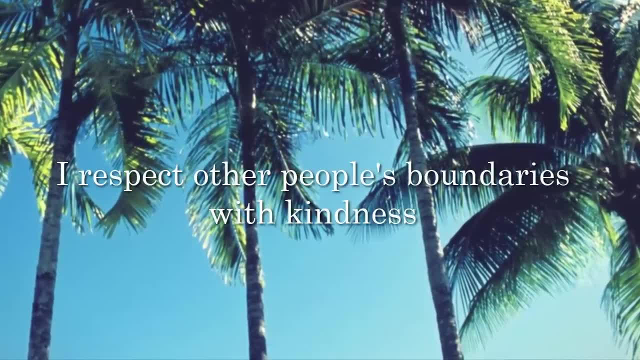 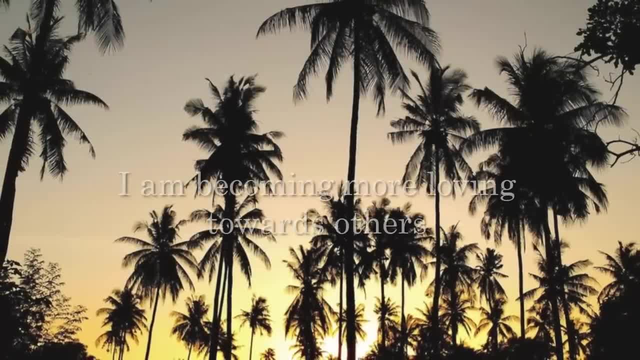 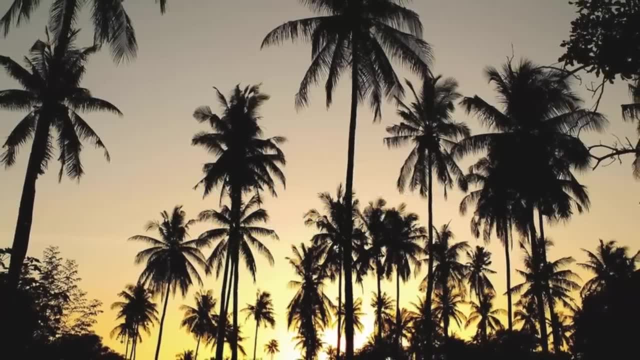 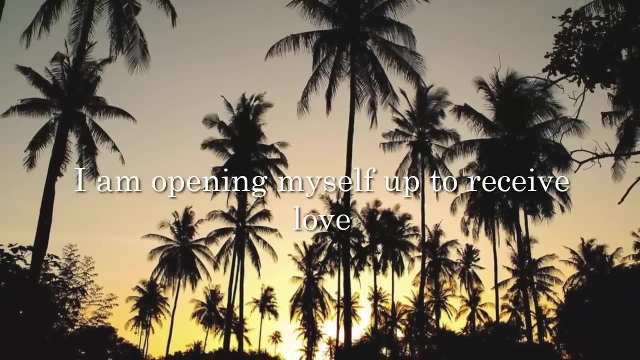 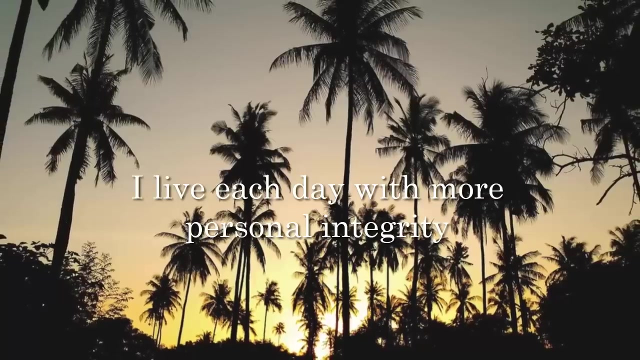 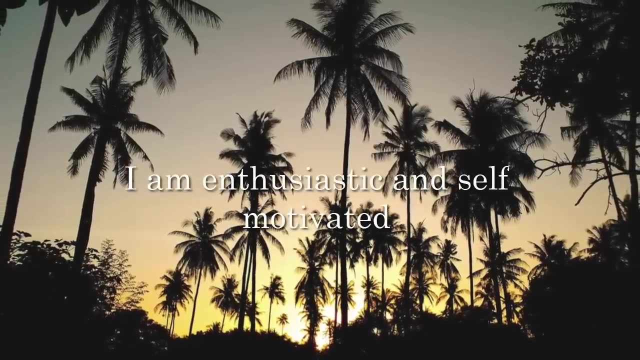 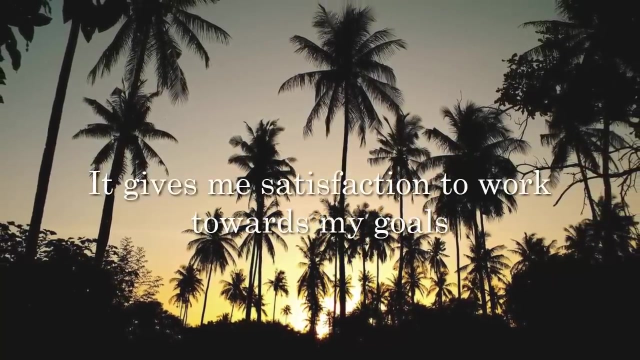 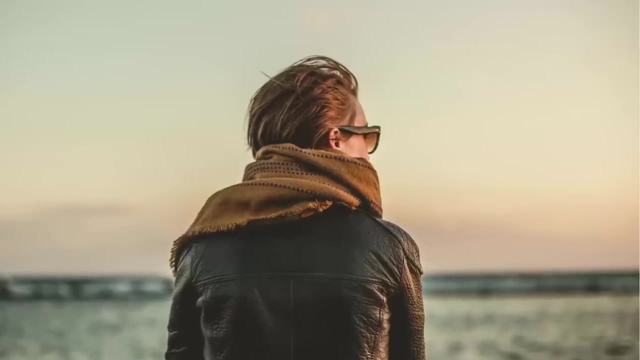 I am becoming more loving towards others. I am becoming more loving towards others. I am opening myself up to receive love. I live each day with more personal integrity. I am enthusiastic and self-motivated. It gives me great satisfaction to work towards my goals. 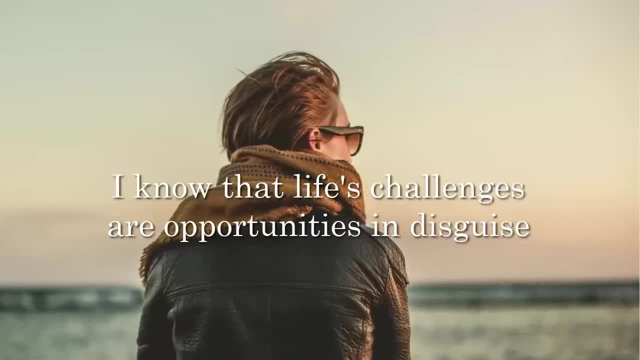 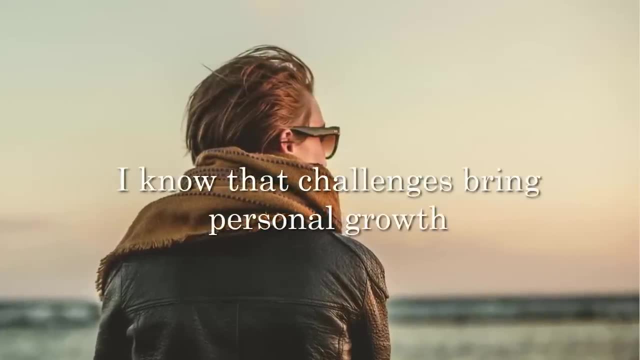 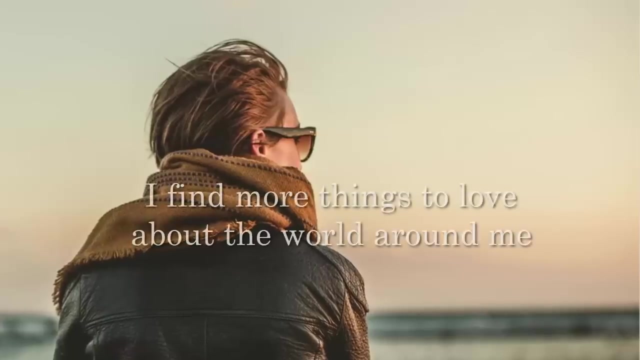 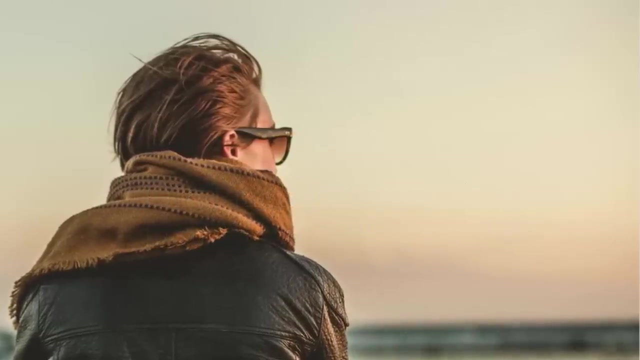 I know that life's challenges are opportunities in disguise. I know that challenges bring personal growth. I am a self-motivated person. I am enthusiastic and self-motivated. I find more things to love about the world around me. I make time each week to enjoy nature. 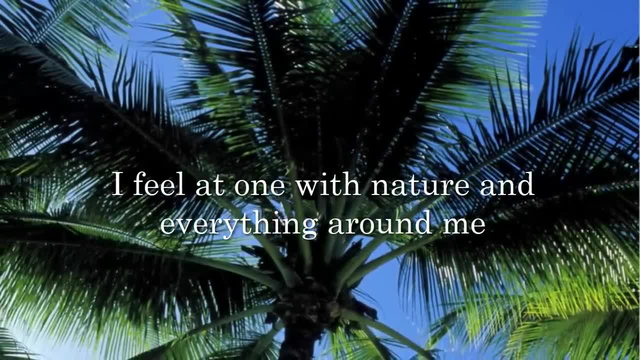 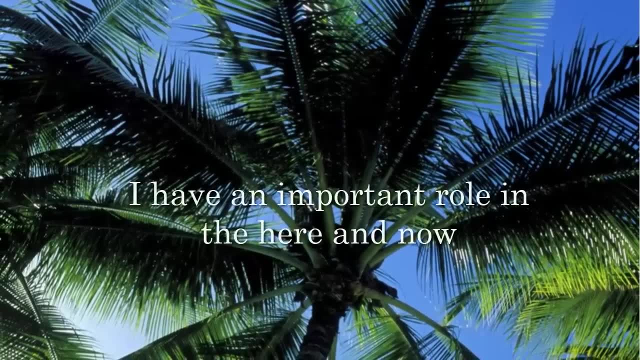 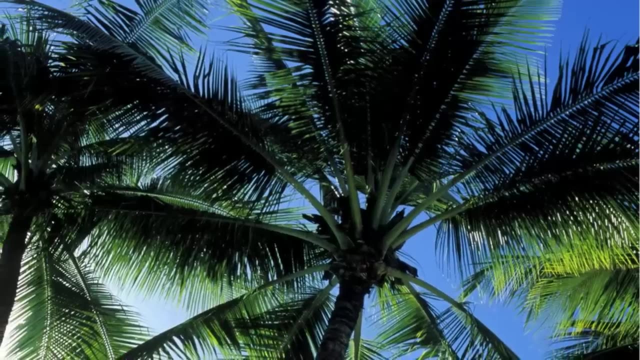 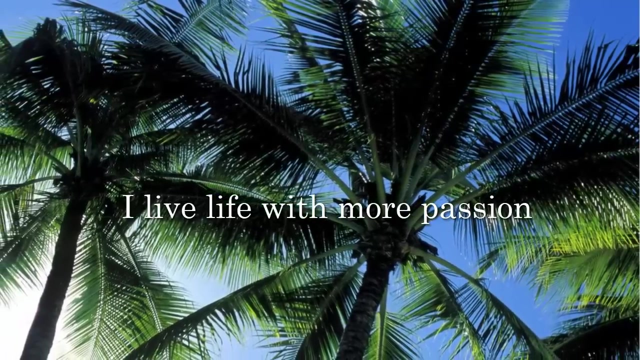 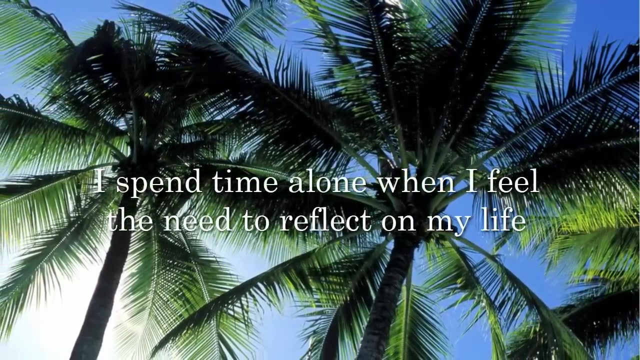 I feel at one with nature and everything around me. I have an important role in the here and now. I live life with more passion. I spend time alone when I feel the need to reflect on my life. I am given a new perspective and focus which allows me to Это. 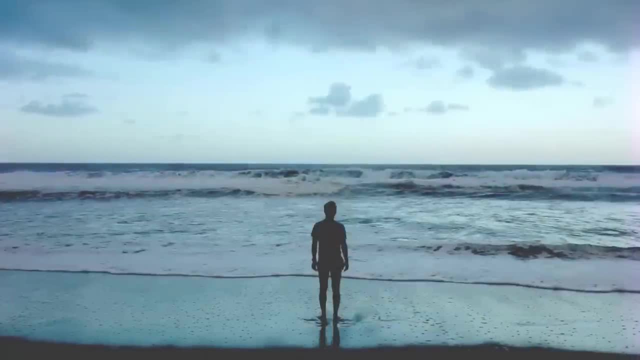 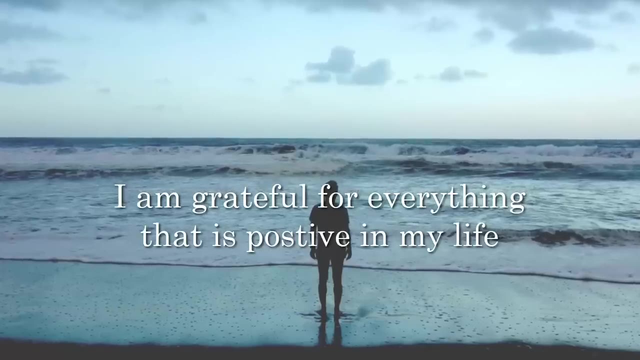 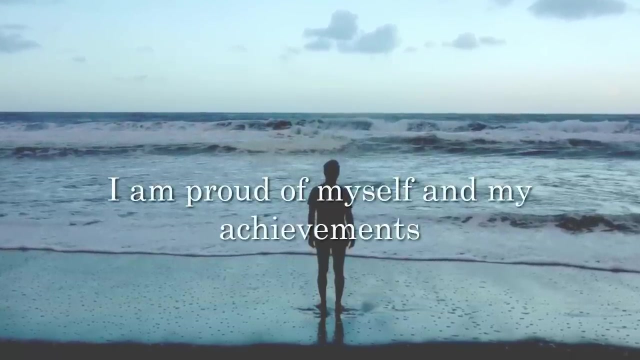 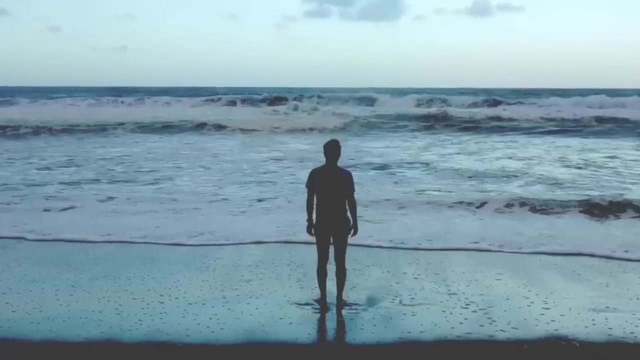 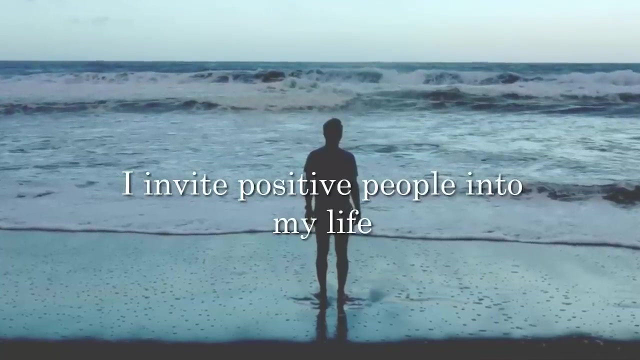 That 제сstedти to live, That takes me into perspective, that συpering to life That makes me feel good and good. I am grateful for everything that is positive about my life. I am proud of myself and my achievements. I invite positive people into my life. 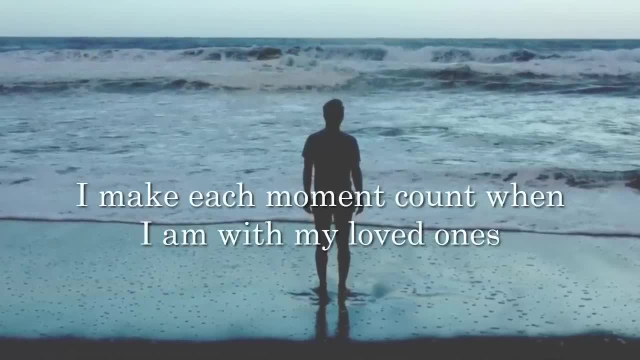 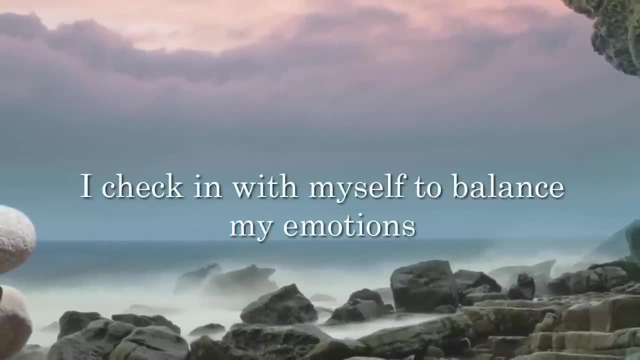 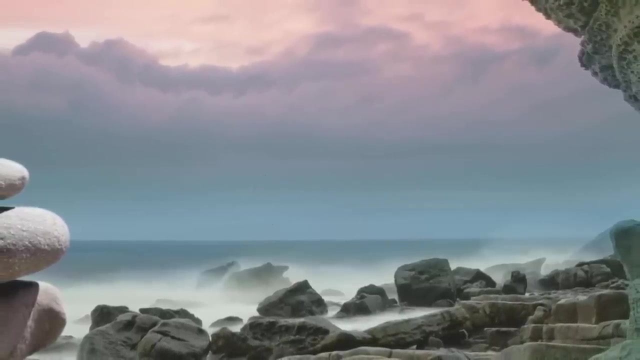 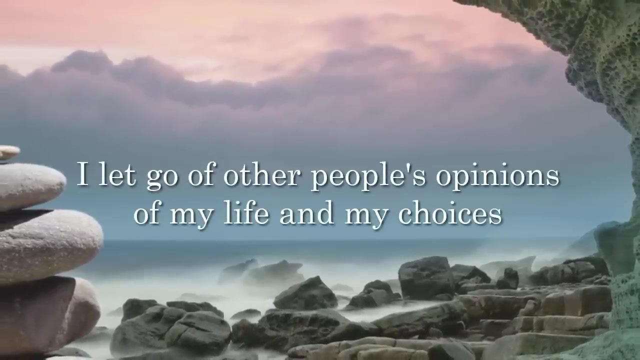 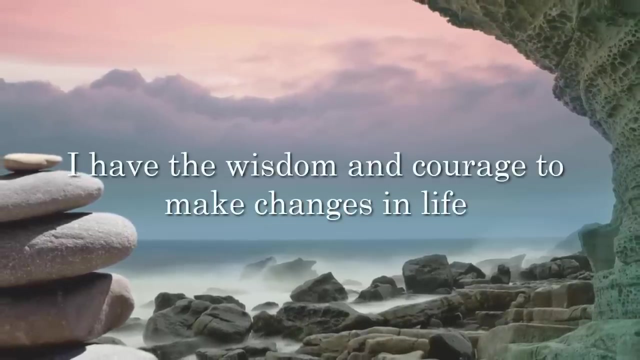 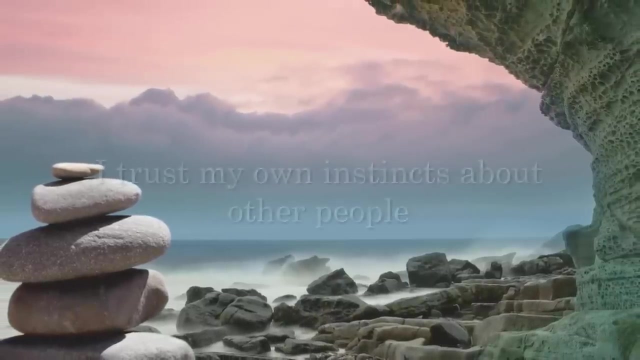 I make each moment count. when I'm with my loved ones, I check in with myself to balance my emotions. I let go of other people's opinions of my life And my choices. I have the wisdom and courage to make changes in life. 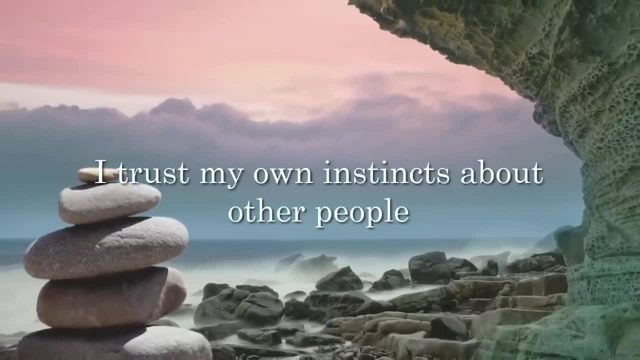 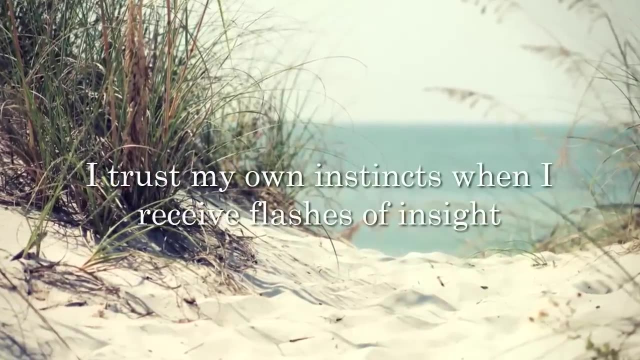 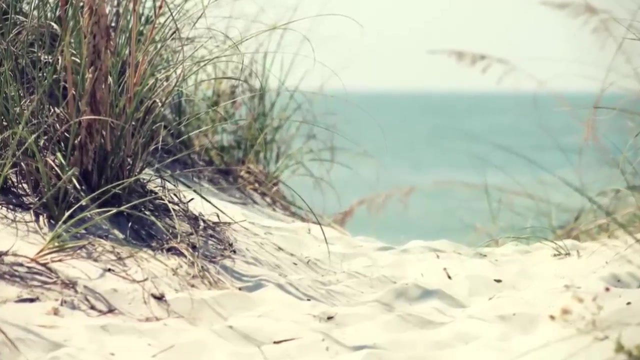 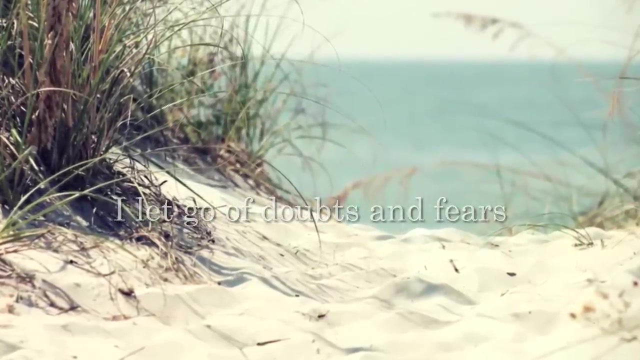 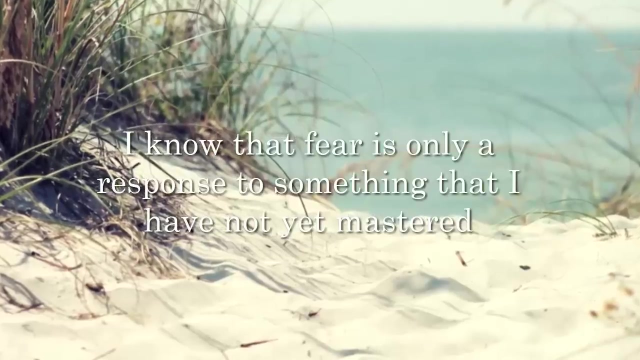 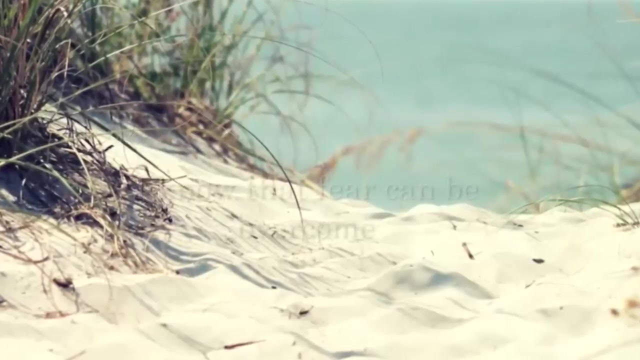 I trust my own instincts about other people. I trust my own instincts when I receive flashes of insight. I let go of doubts and fears. I know that fear is only a response to something I have not yet mastered. I know that fear can be overcome. 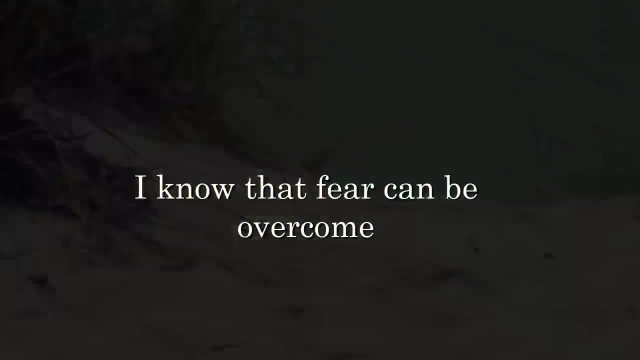 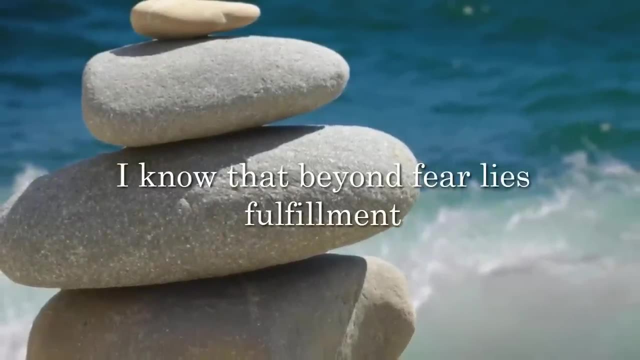 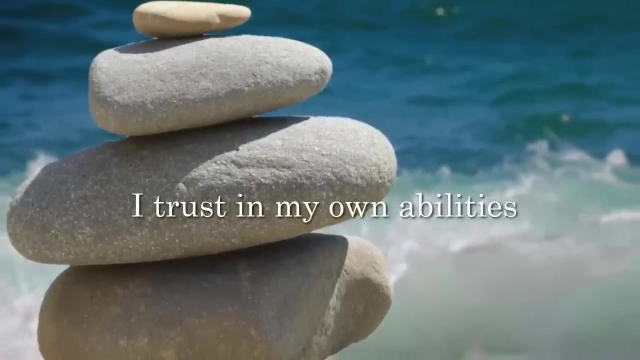 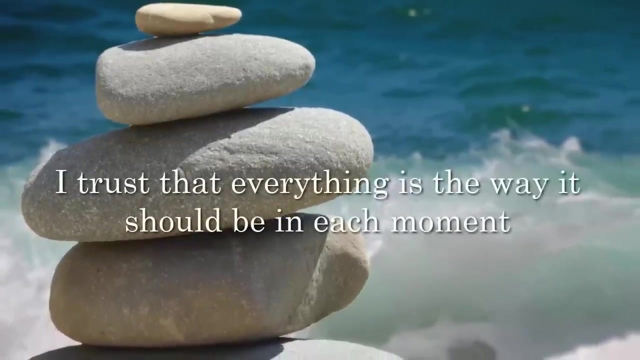 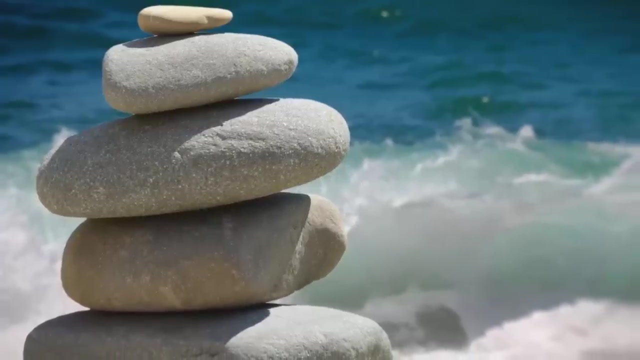 I know that fear can be overcome. I know that beyond fear lies fulfilment. I trust in my own abilities. I trust that everything is the way it should be in each moment. I trust that everything is the way it should be in each moment. 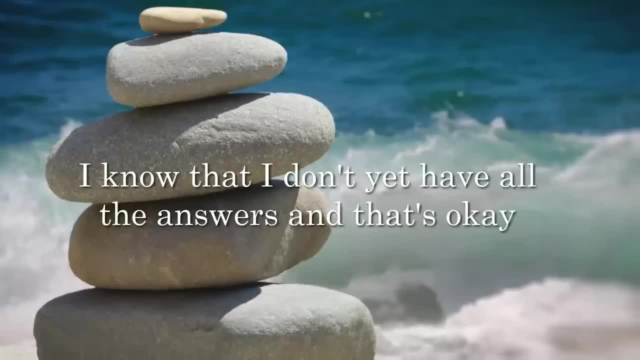 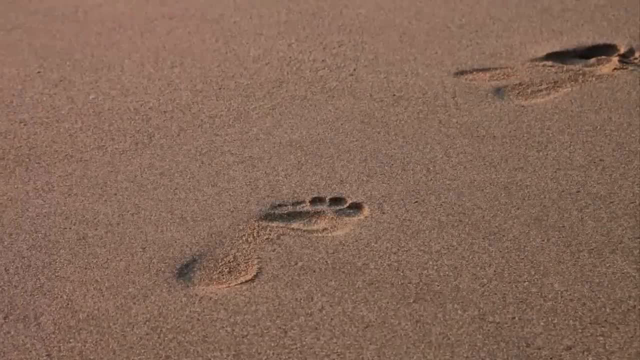 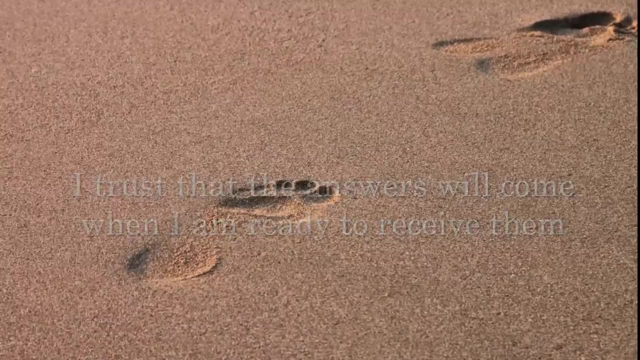 I know that my break-out is to be believed, but it is not fake. I know that I don't yet have all the answers and that it's ok. I trust that the answers will come when I am ready to receive them. I am growing into the person I want to become. 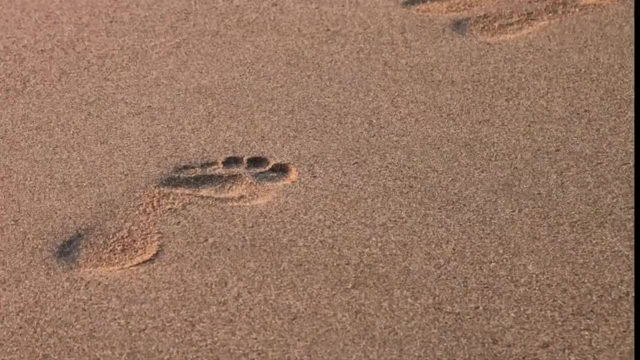 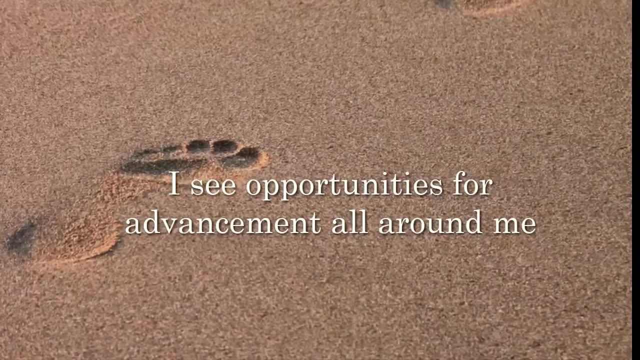 I am positive. I gather all the keys, I theCUBE my choices. I glory myself. I believe in me. I believe in me. I do the choices. I believe in me. I believe in me. opportunities for advancement all around me. I act on opportunities as soon as. 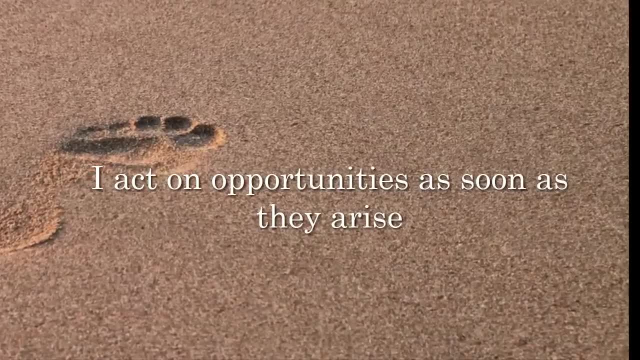 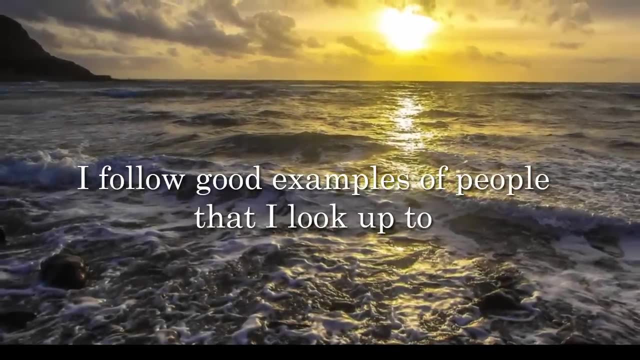 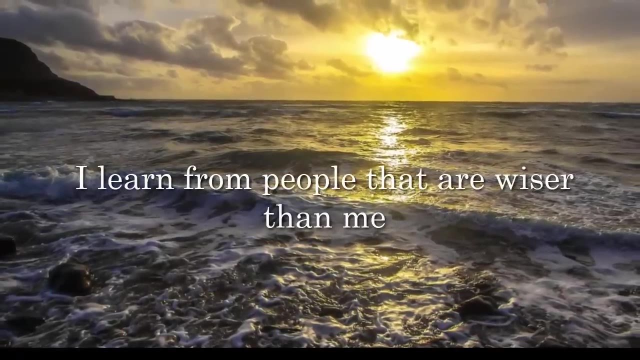 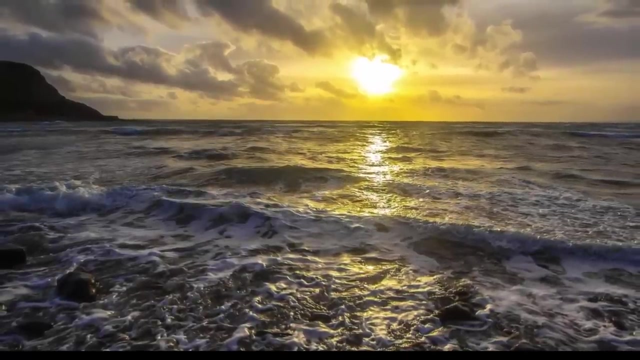 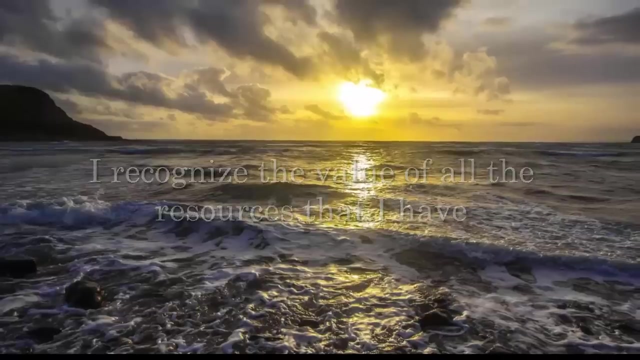 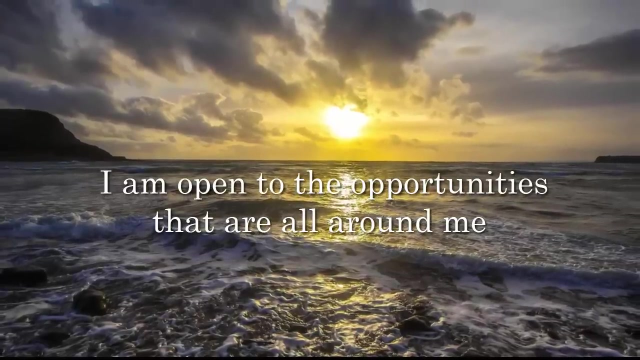 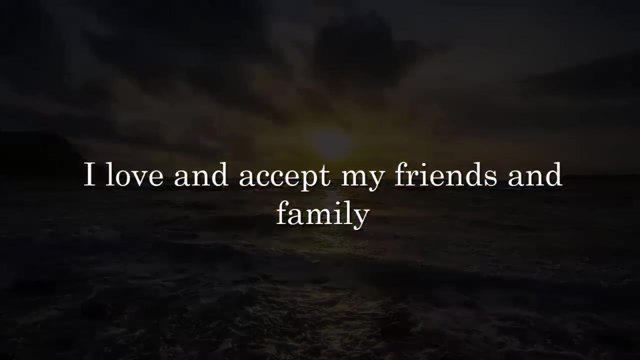 they arise. I follow good examples of people that I look up to. I learn from people that are wiser than me. I recognize the value of all the resources that I have. I am open to the opportunities that are all around me. I love and accept my friends and family. 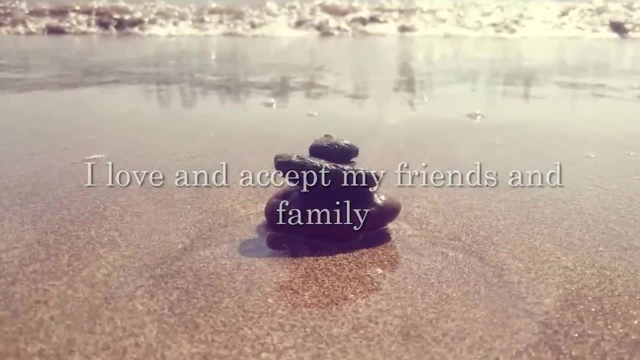 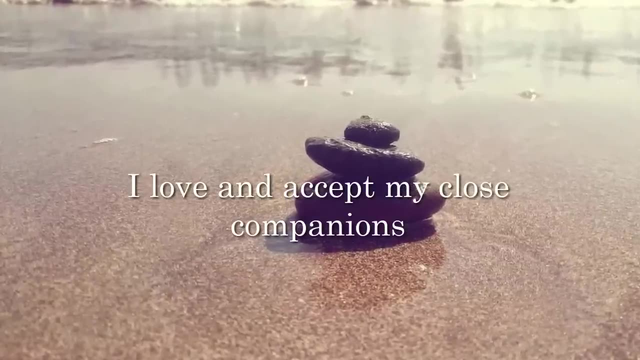 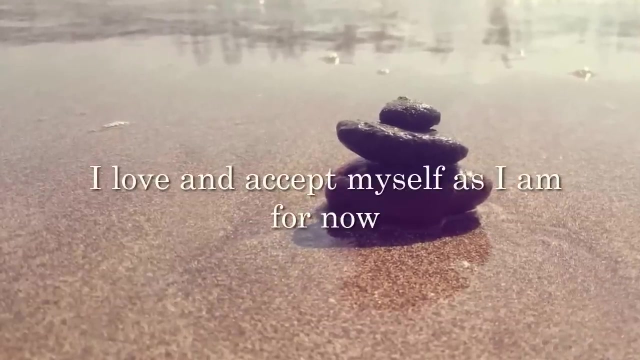 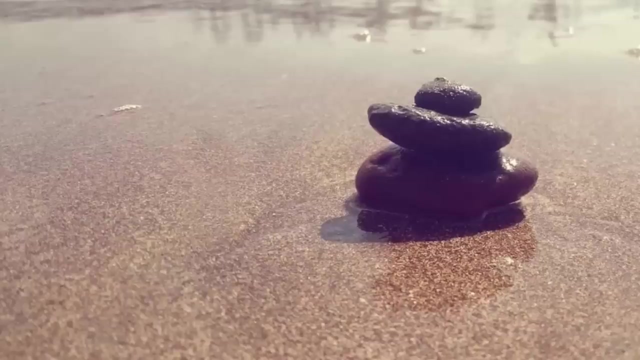 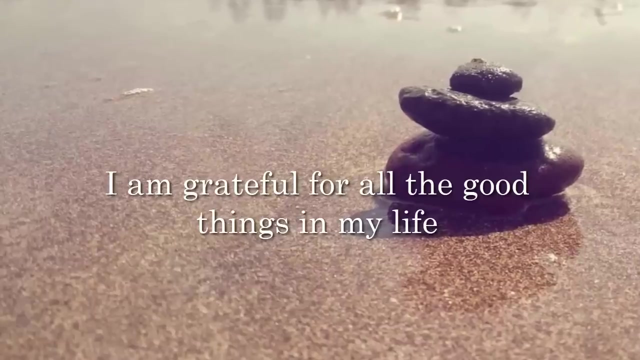 I love and accept my close companions. I love and accept myself as I am. for now, I am grateful for all the good things in my life. I believe I have'll be able to change the world around me somewhere soon. I trust that I can change that which no longer serves me. 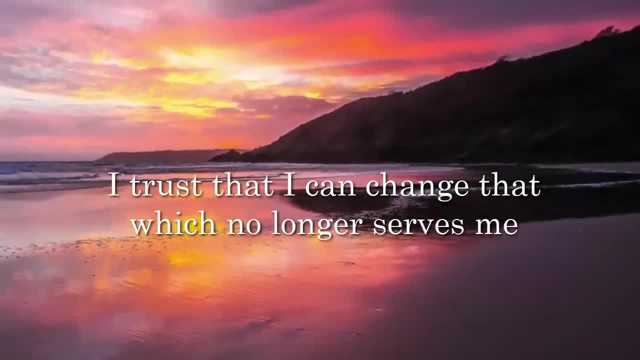 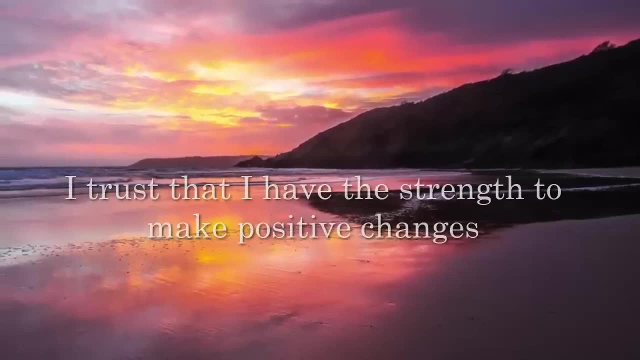 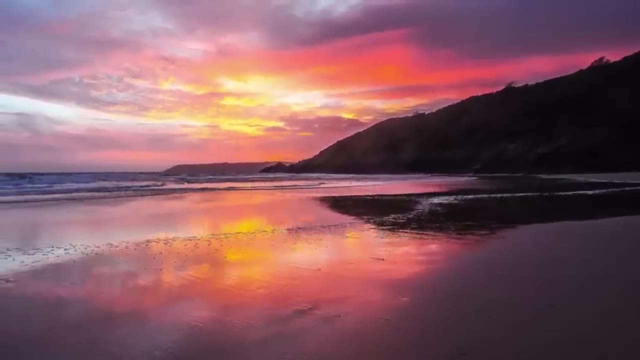 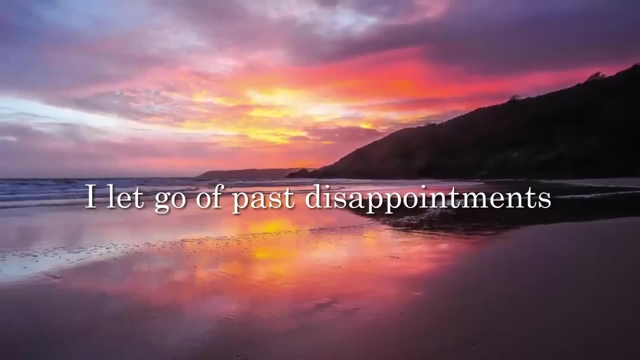 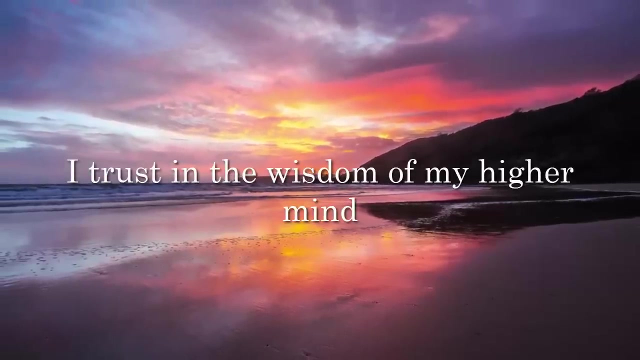 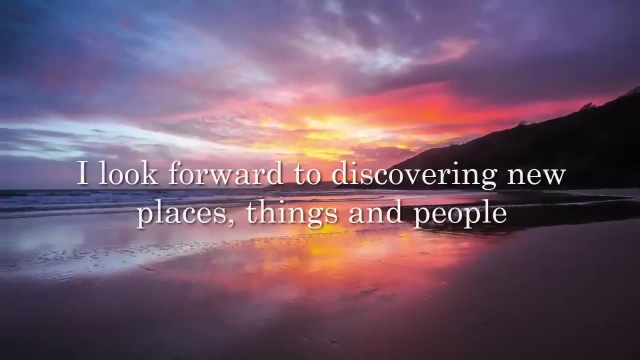 I can change what I am and what I am no longer needs me. I trust that I have the strength to make positive changes. I let go of past disappointments. I trust in the wisdom of my higher mind. I look forward to discovering new places, things and people. 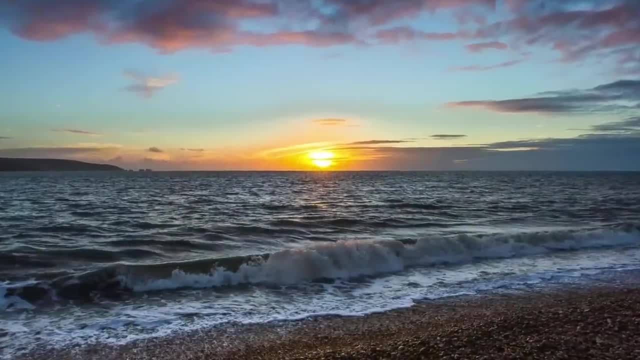 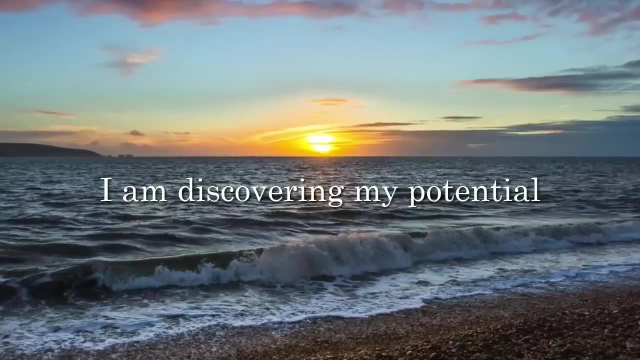 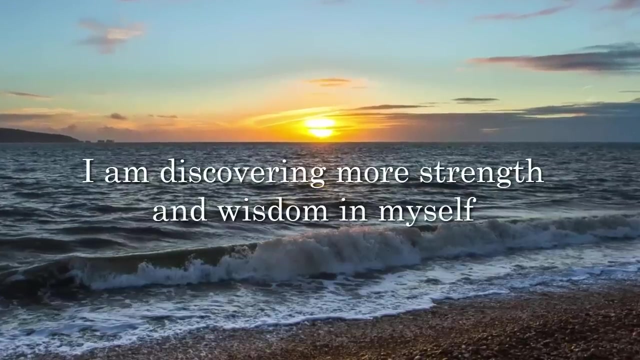 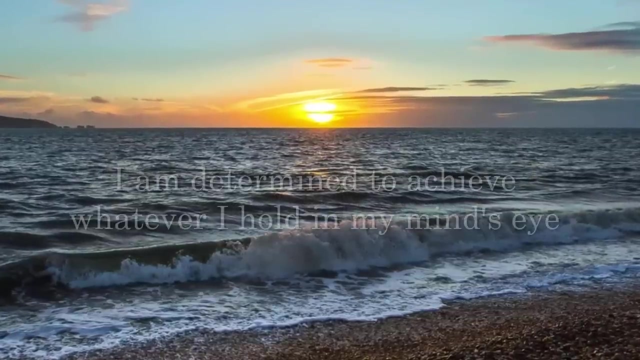 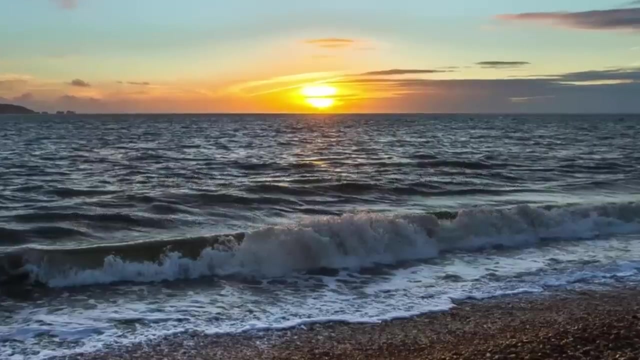 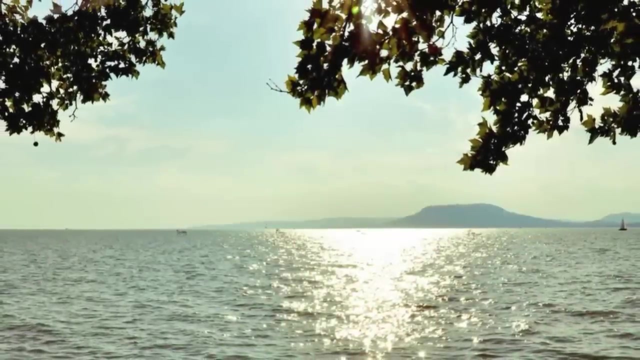 I am discovering my potential. I am discovering more strength and wisdom in myself. I am determined to achieve whatever I hold in my mind's eye, And so it is. my words become the truth. I am discovering more. I am discovering more. 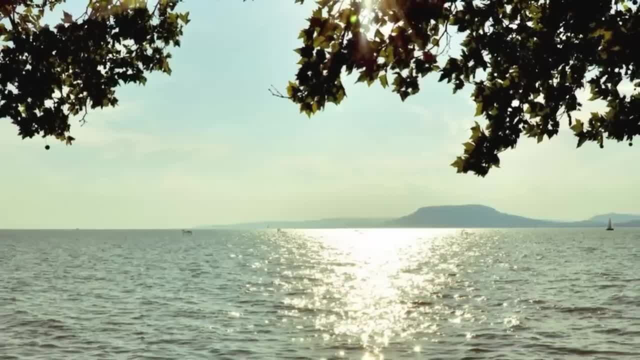 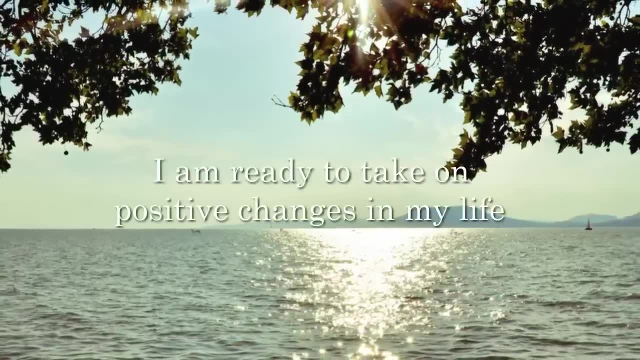 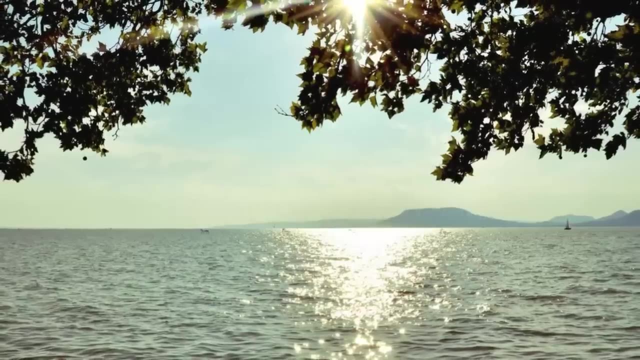 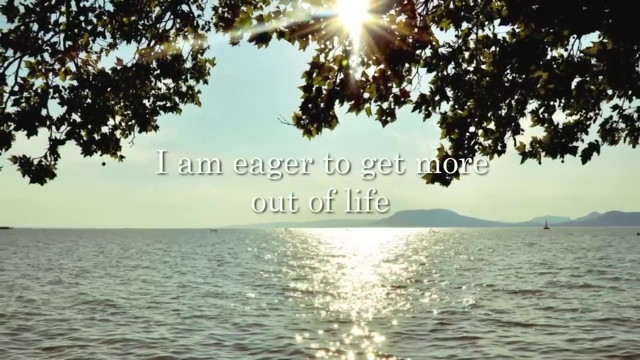 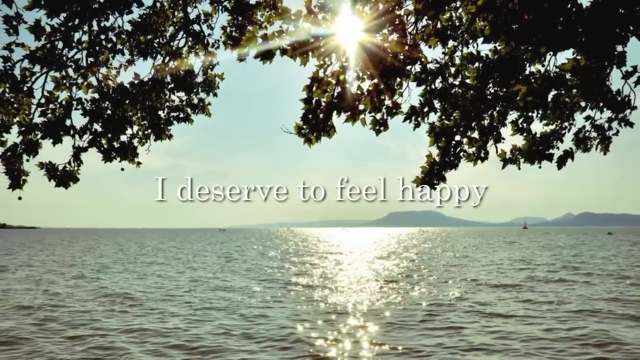 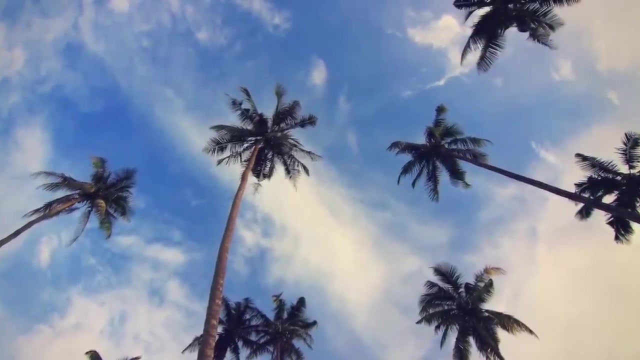 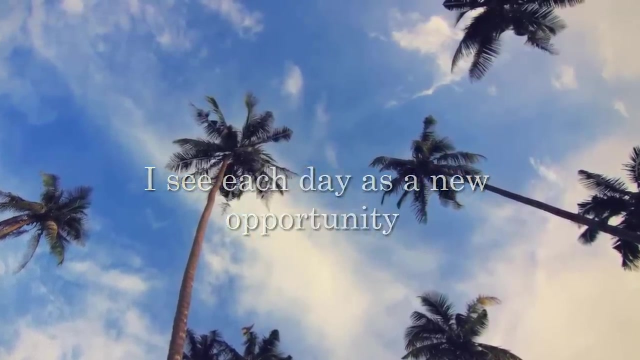 I am ready to take on positive changes in my life. I am eager to get more out of life. I am ready to take on positive changes in my life. I deserve to feel happy. I see each day as a new opportunity. I take good care of myself. 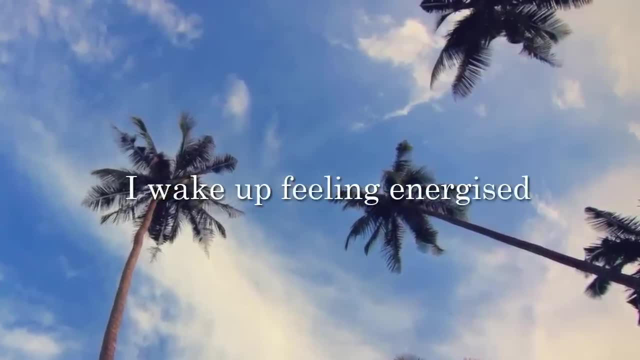 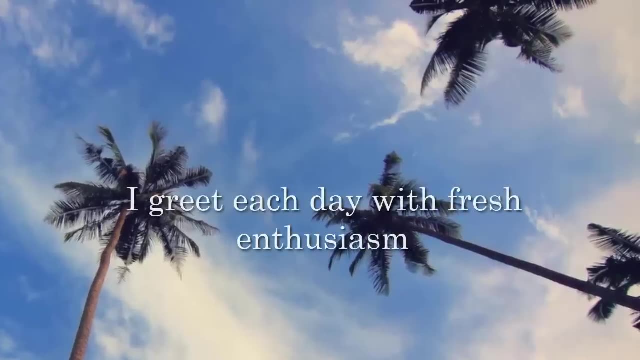 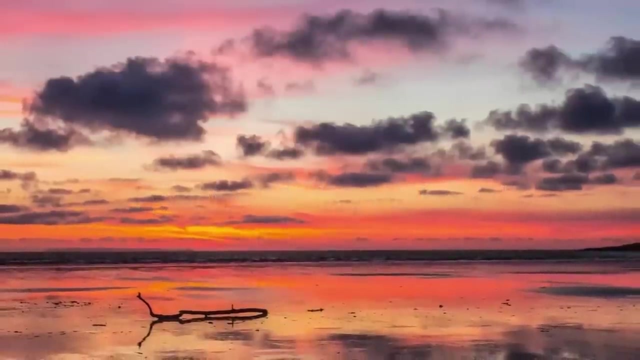 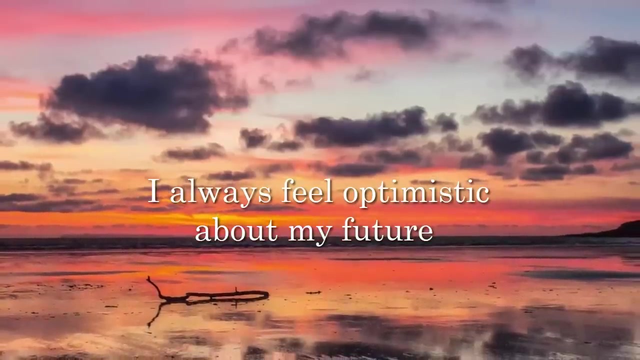 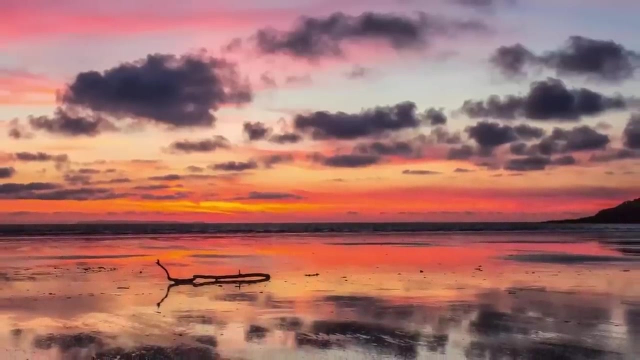 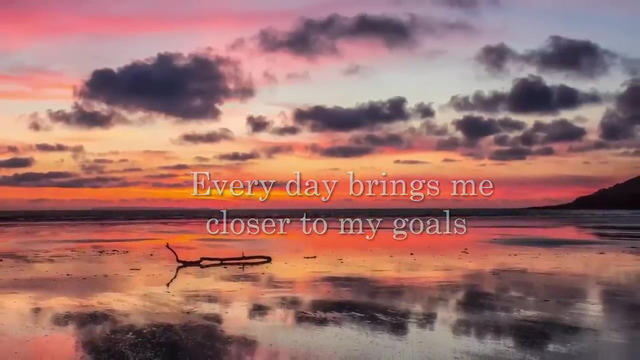 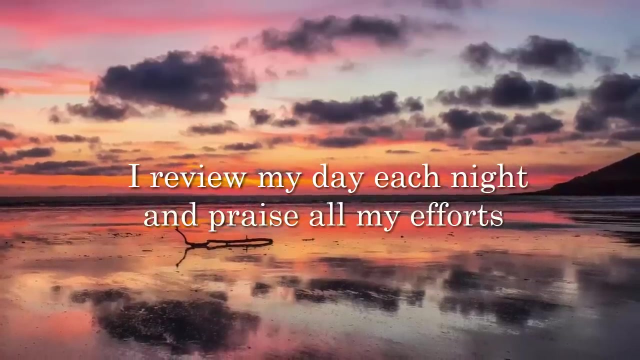 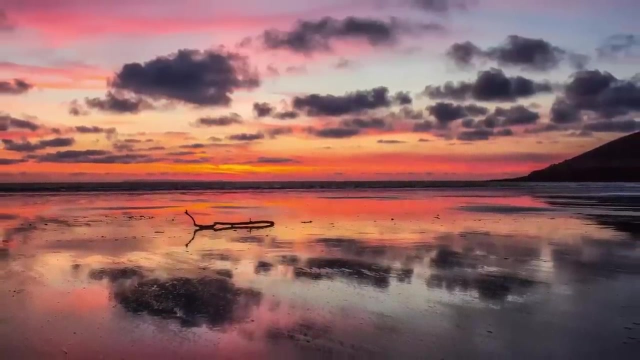 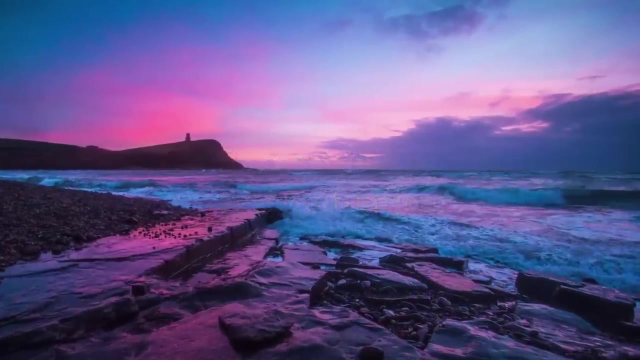 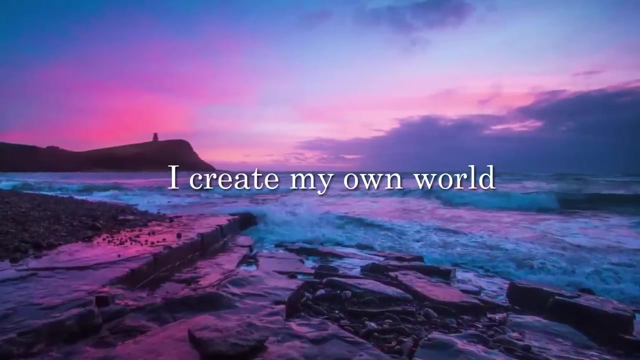 I wake up feeling energized. I greet each day with fresh enthusiasm. I always feel optimistic about my future. Every day brings me closer to my goals. I review my day each night and praise all my efforts. I see the positive aspect of every situation. I create my own world. I am learning to love everything about who. 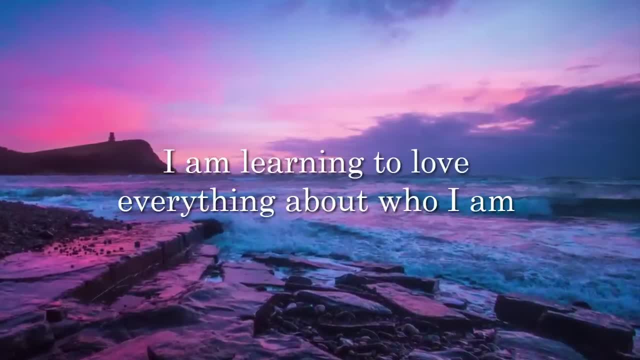 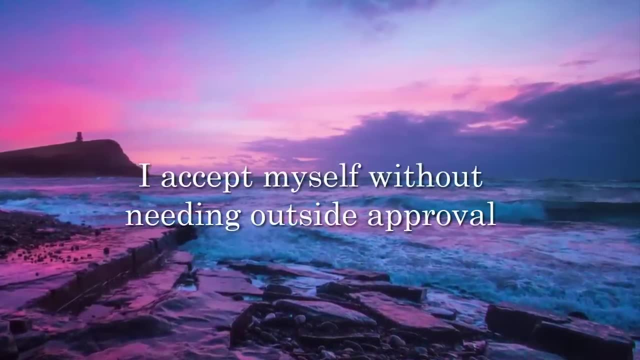 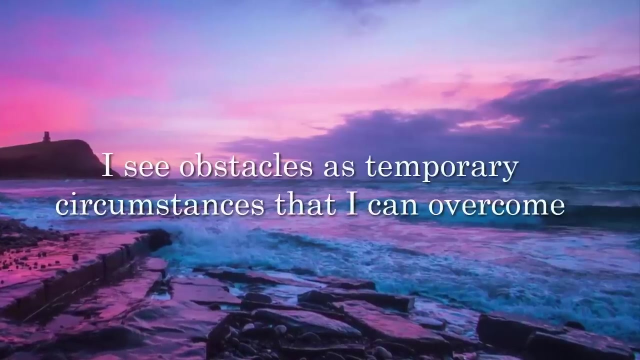 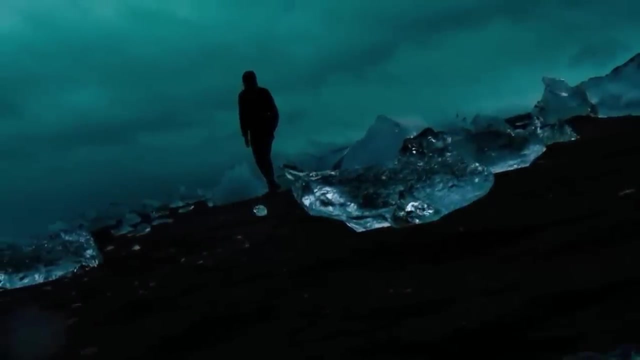 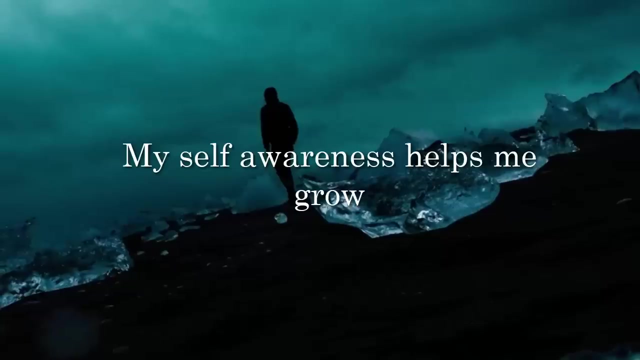 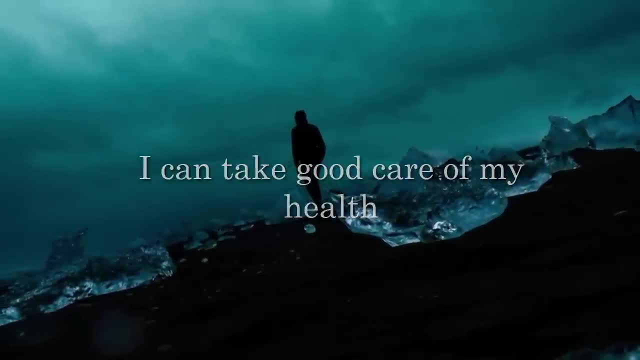 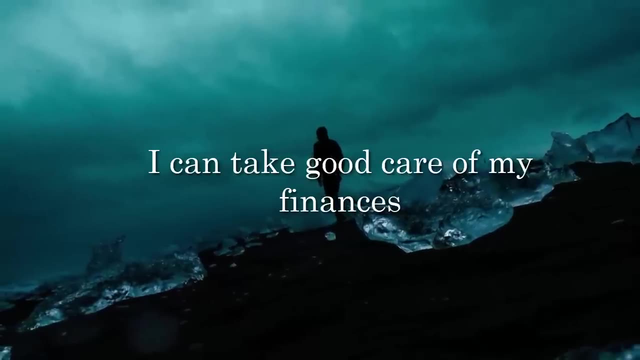 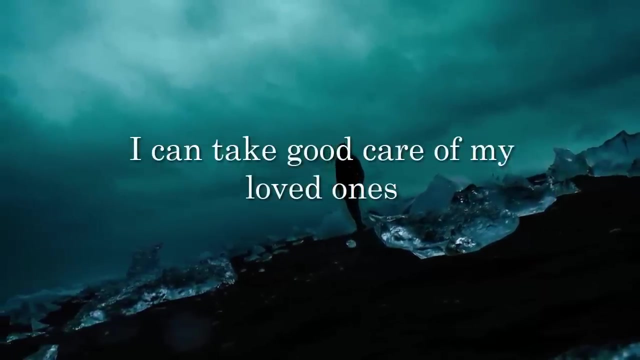 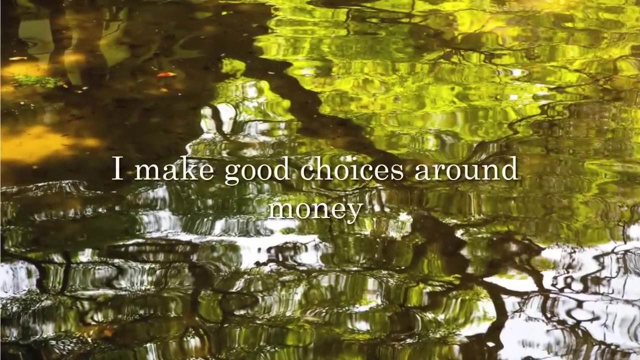 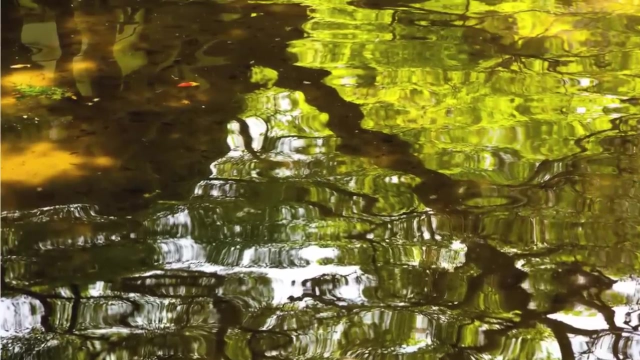 I can take good care of my finances. I can take good care of my loved ones. I can take good care of my loved ones. I make good choices around money. I make good choices around money. Each day I get better at recognizing my true friends. Each day I get better at recognizing my true friends. 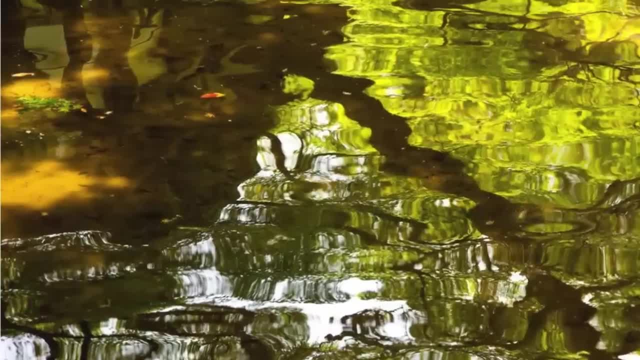 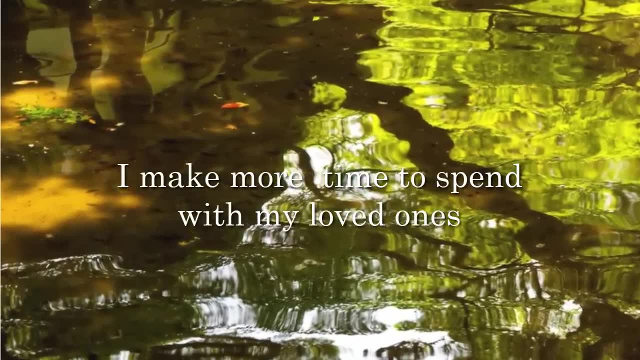 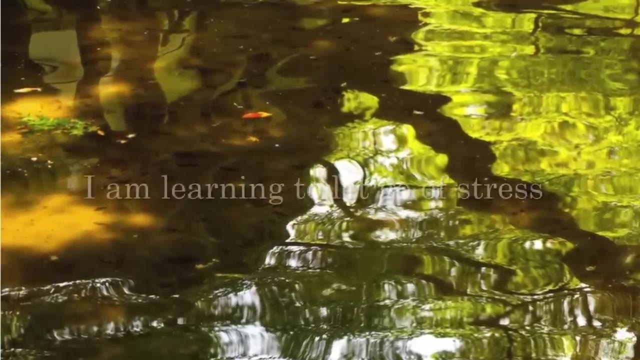 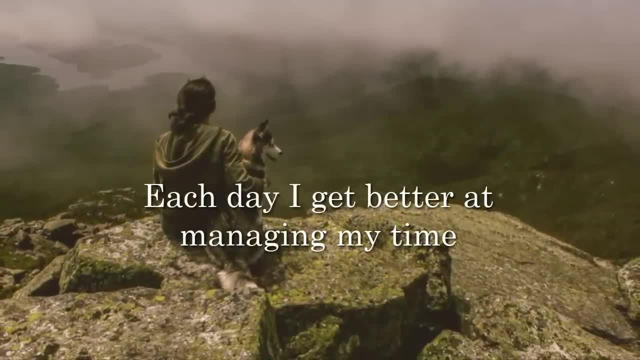 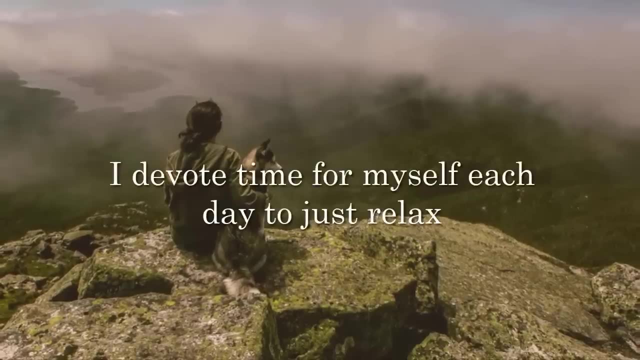 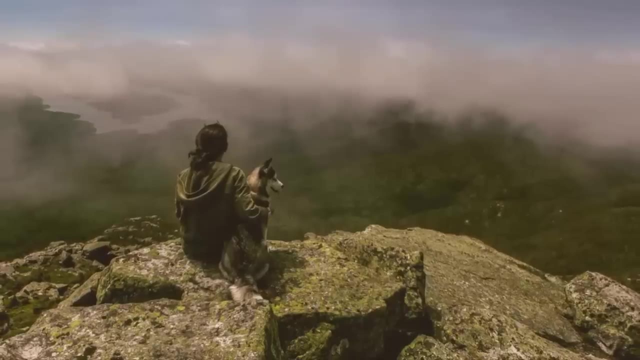 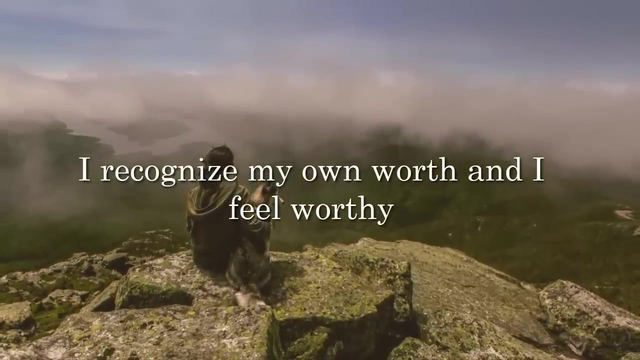 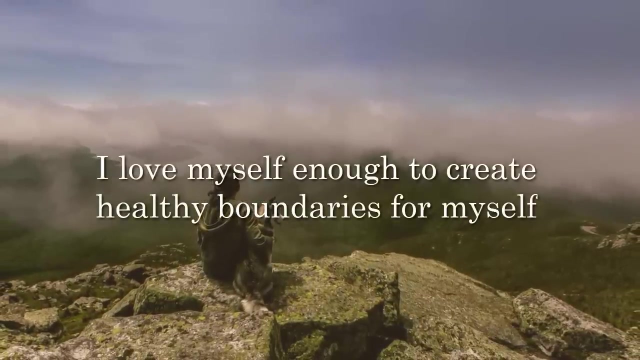 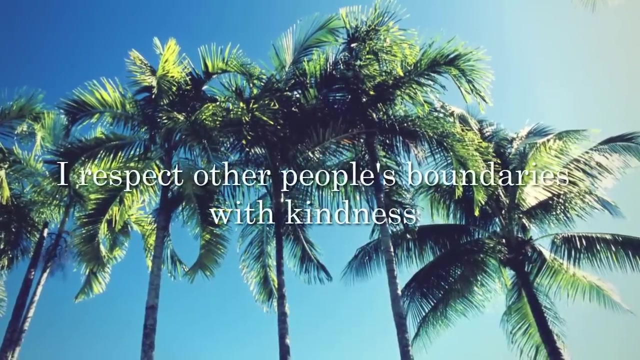 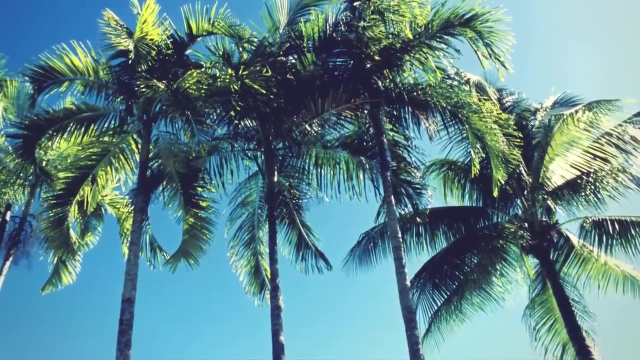 each day I get better at managing my time. I devote time for myself each day to just relax. I recognize my own worth and I feel worthy. I love myself enough to create healthy boundaries for myself. I respect other people's boundaries with kindness. I am becoming more loving towards others. 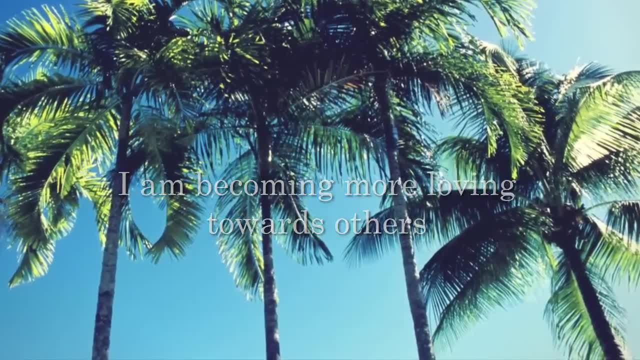 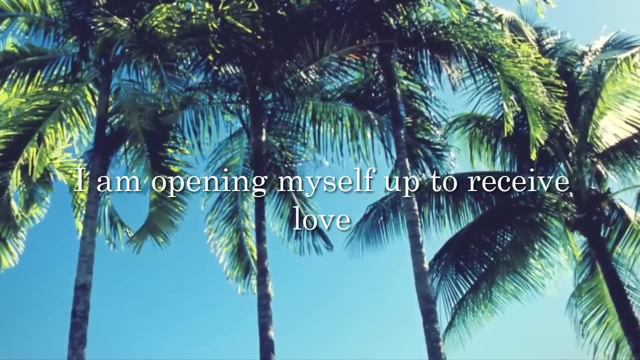 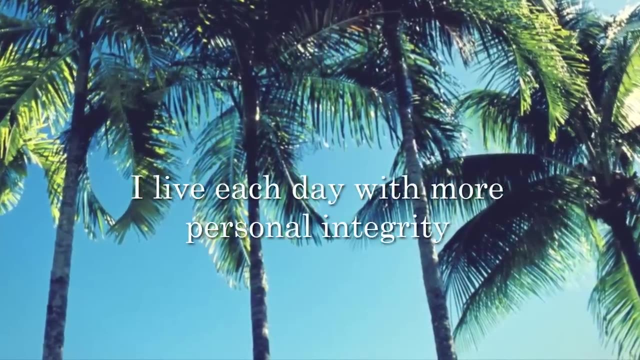 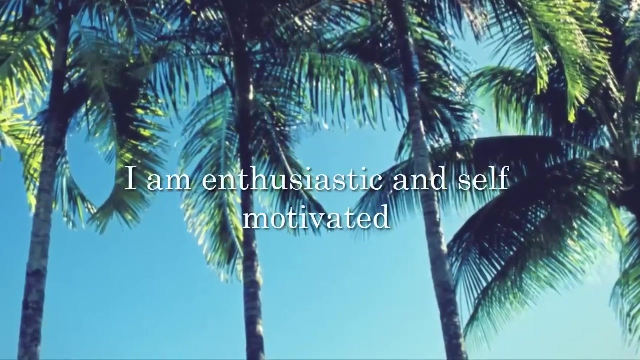 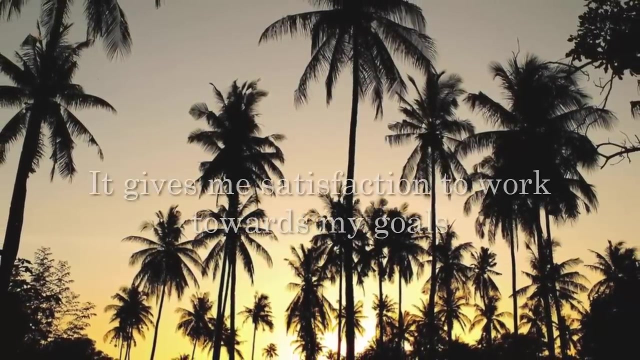 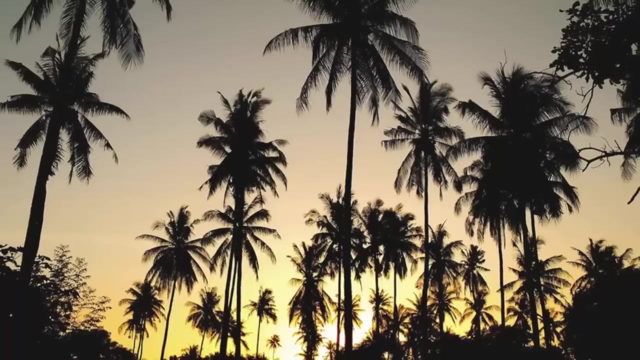 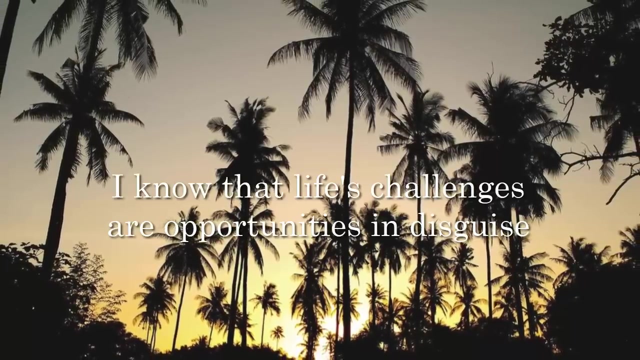 I am opening myself up to receive love. I live each day with more personal integrity. I am enthusiastic and self-motivated. it gives me great satisfaction to work towards my goals. I know that life's challenges are opportunities in disguise. I know that challenges bring me happiness. 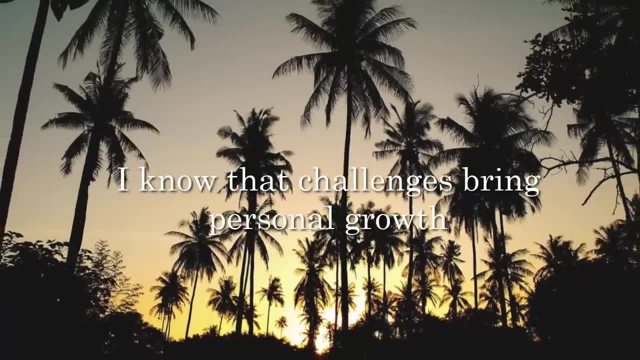 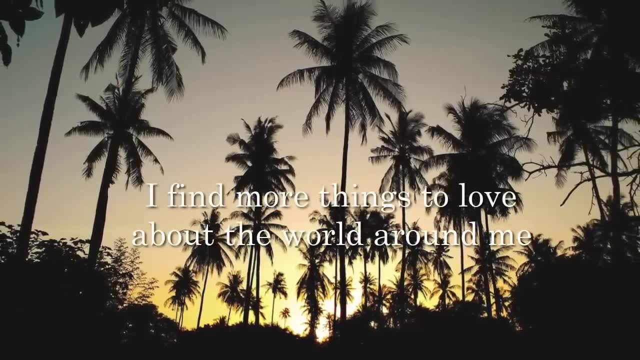 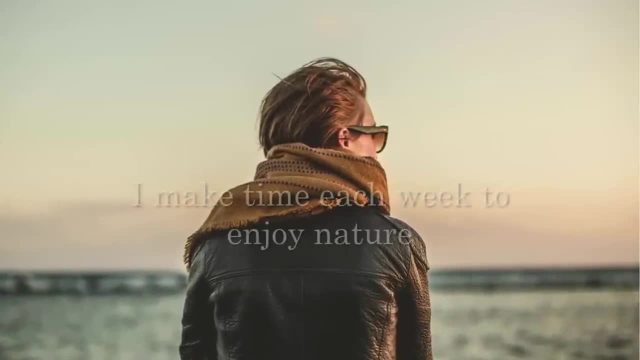 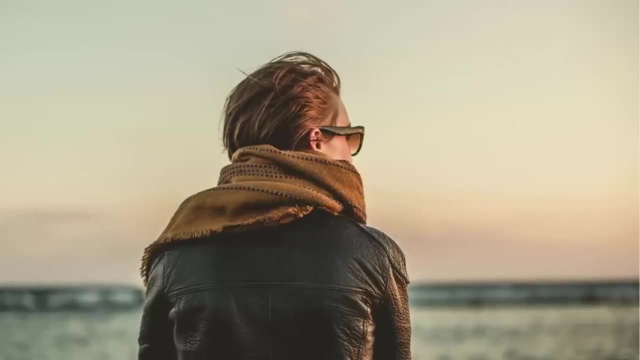 I know that life's challenges bring me happiness. I know that love does not bring personal growth. Love gives my feet and body aku. I find more things to love about the world around me. I make time each week to enjoy nature. Nature praises me. I feel at one with nature and everything around me. 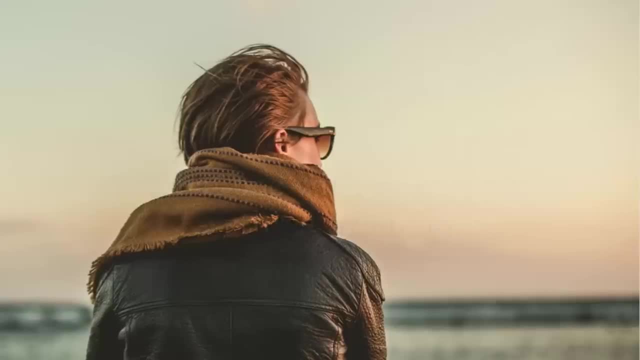 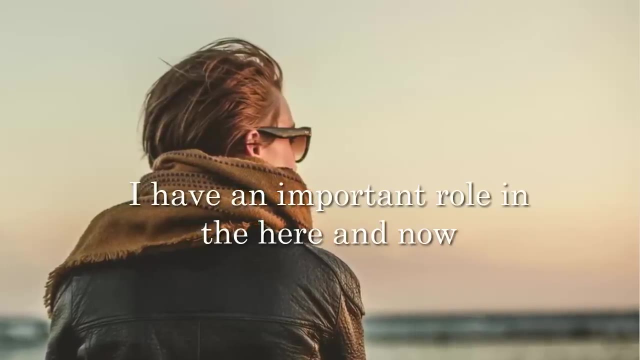 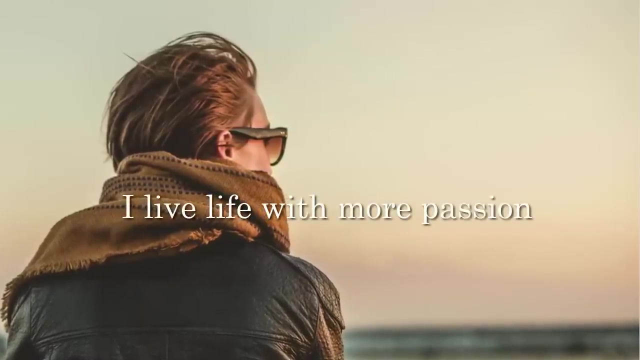 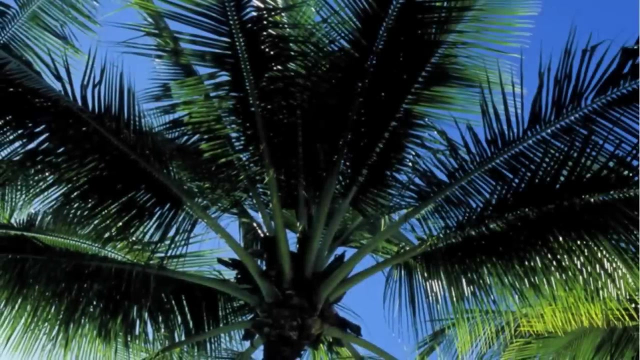 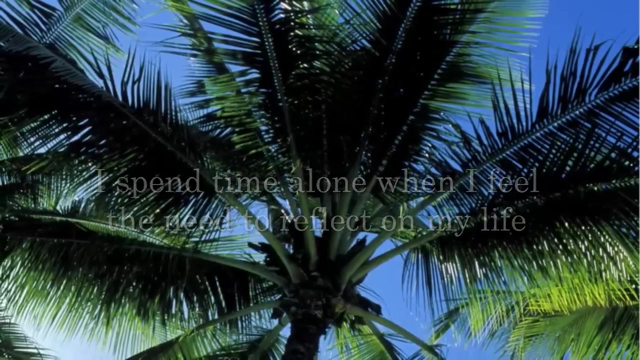 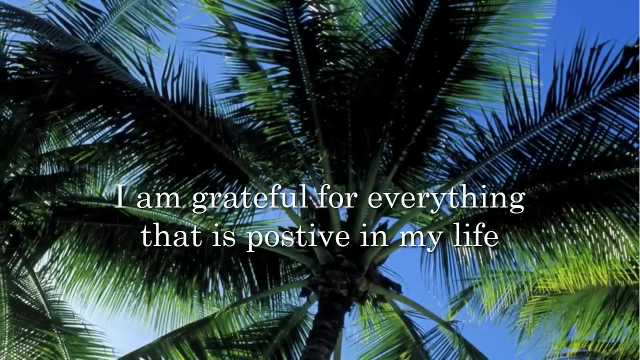 Nature delves into creative levels based on her ability and boundaries. I have an important role in the here and now. I live life with more passion. I spend time alone when I feel the need to reflect on my life. I am grateful for everything that is positive about my life. 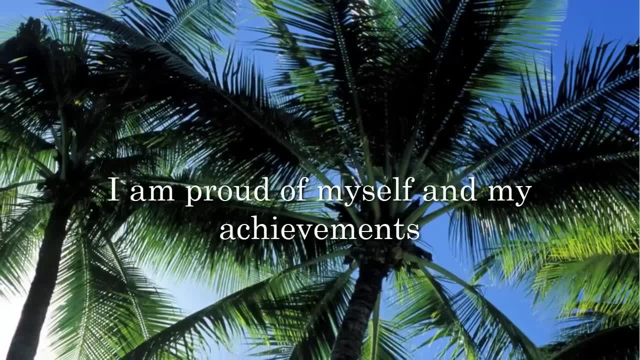 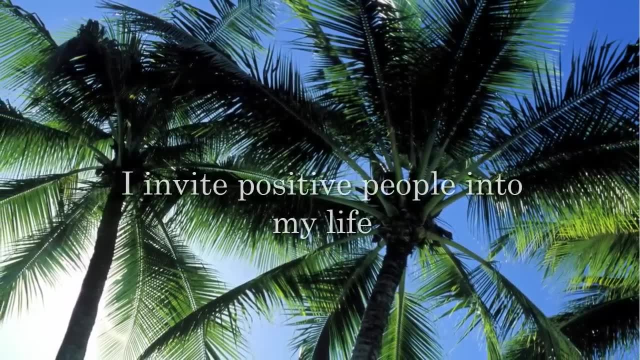 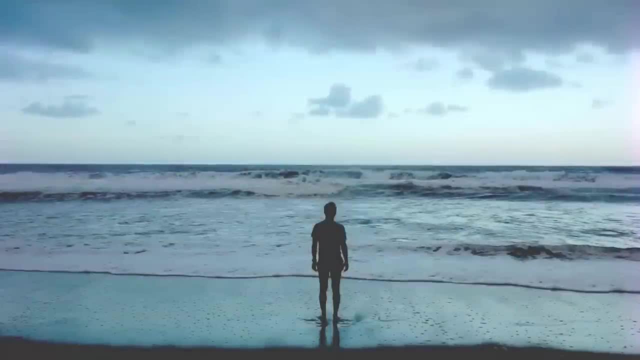 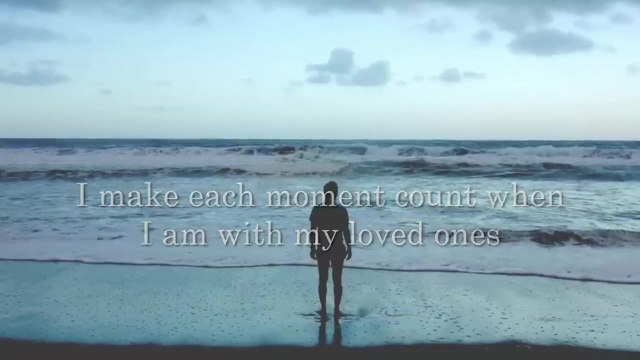 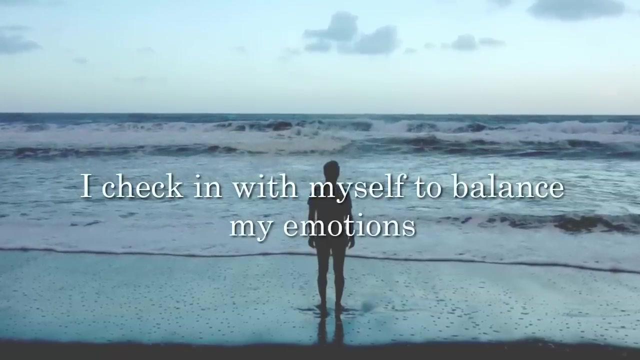 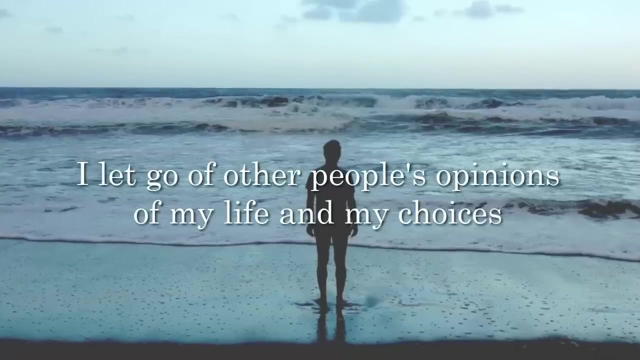 I am proud of myself and my achievements. I invite positive people into my life. I make each moment count. when I'm with my loved ones, I check in with myself to balance my emotions. I let go of other people's opinions of my life and my choices. 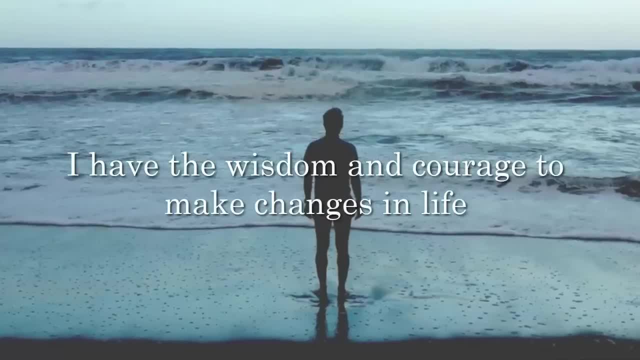 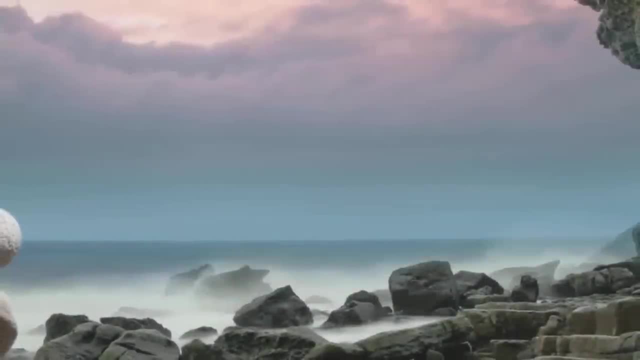 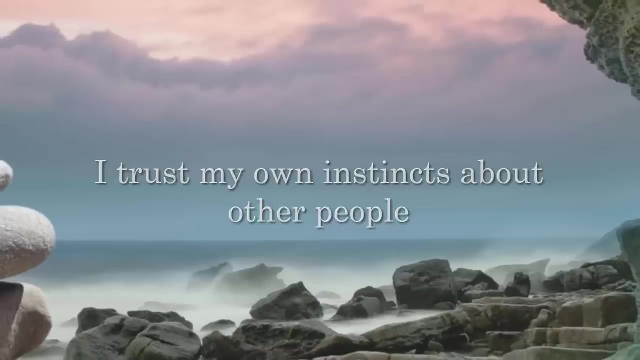 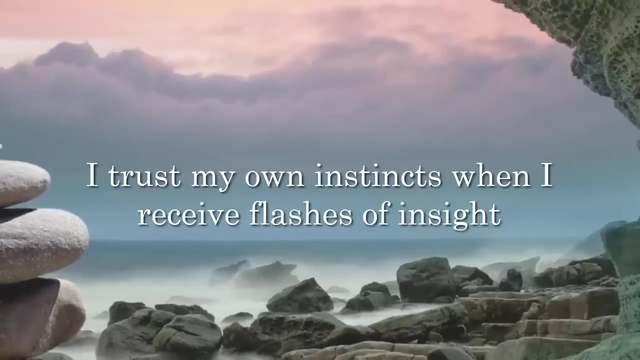 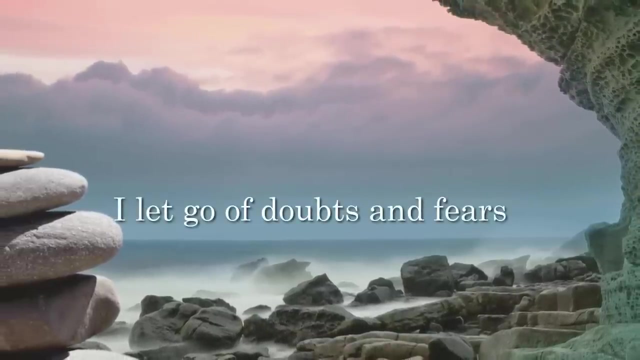 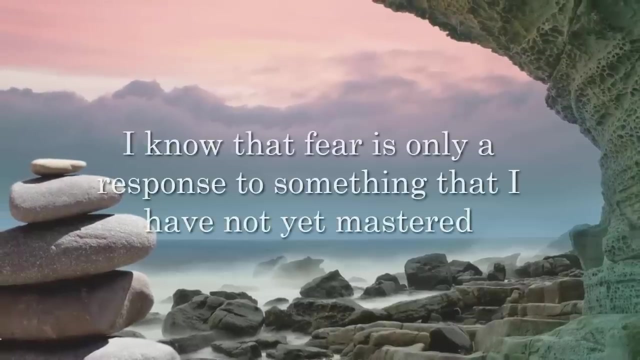 I have the wisdom and courage to make changes in life. I trust my own instincts about other people. I trust my own instincts when I receive flashes of insight. I let go of doubts and fears. I know that fear is only a response to something I have not yet mastered. 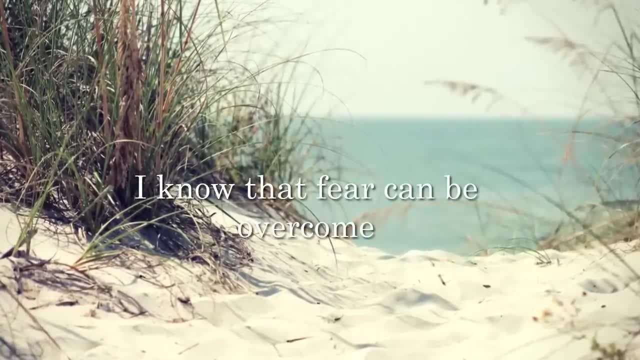 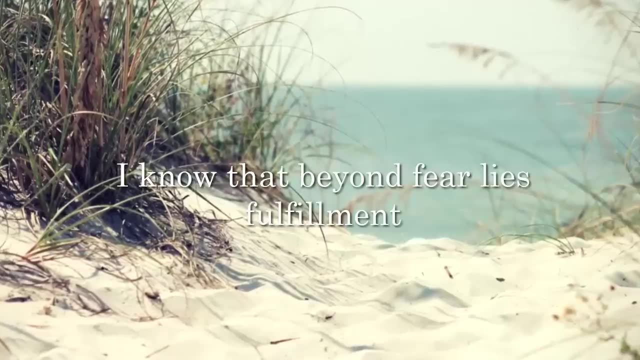 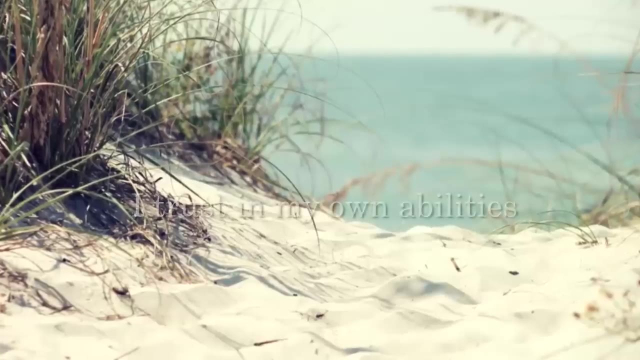 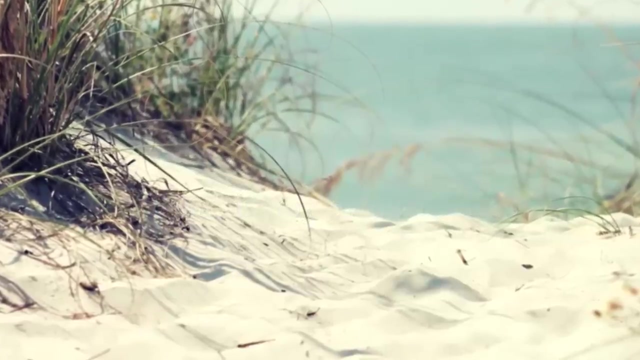 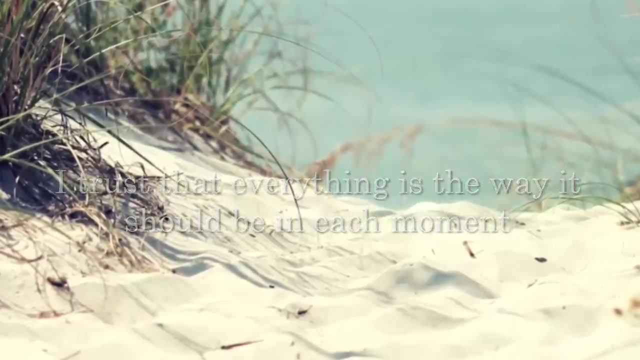 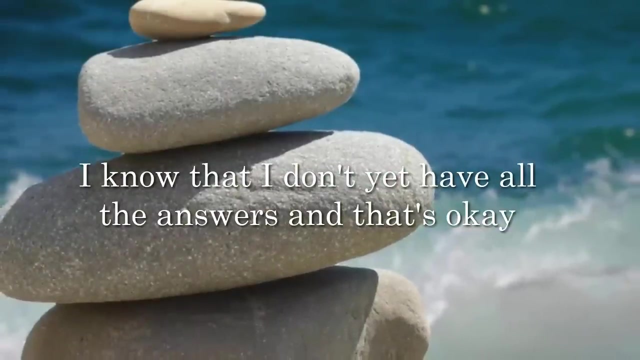 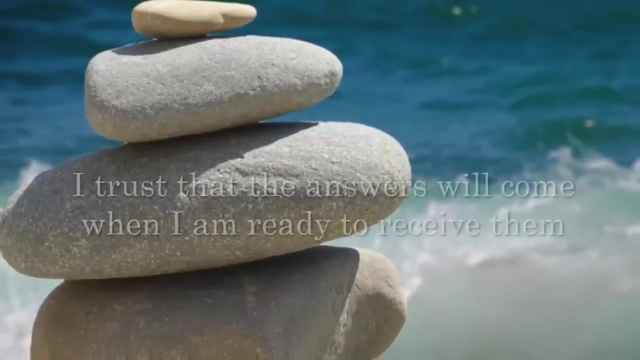 I know that fear can be overcome. I know that beyond fear lies fulfilment. I trust in my own abilities. I trust that everything is the way it should be in each moment. I know that I don't yet have all the answers and that it's okay. 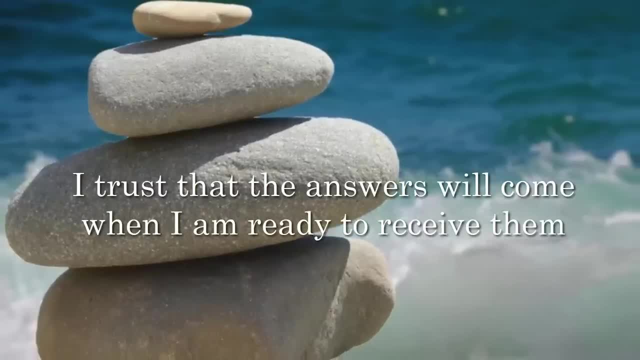 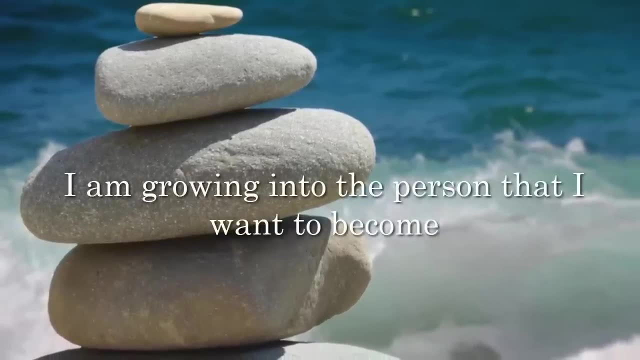 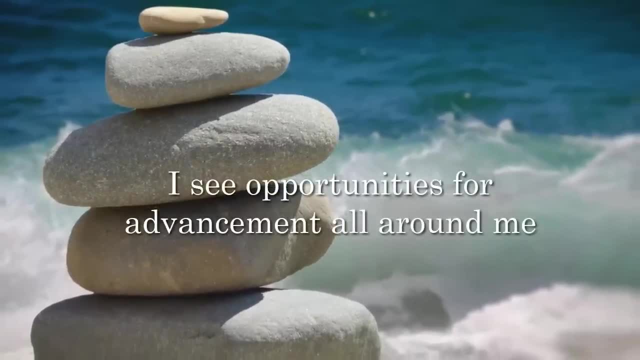 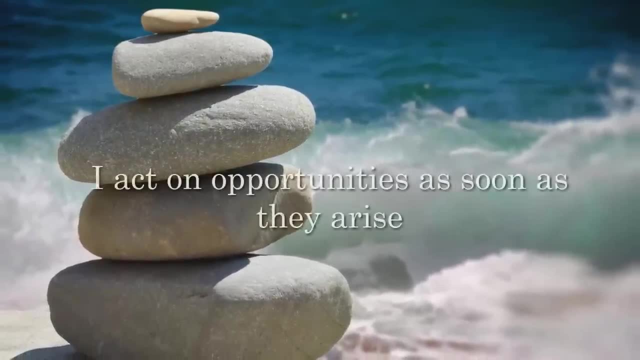 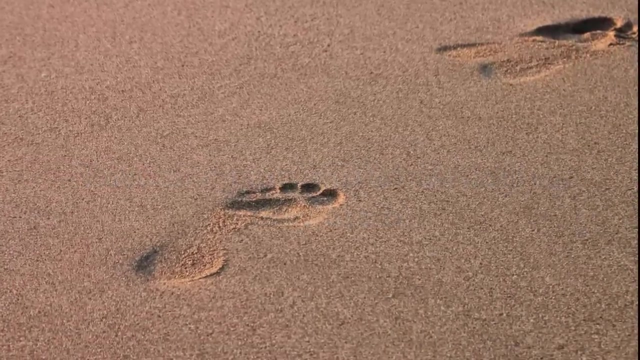 I see opportunities for advancement all around me. I act on opportunities as soon as they arise. I follow good examples of people that I look up to. I look up to people that I love. I look up to people that I look up to. 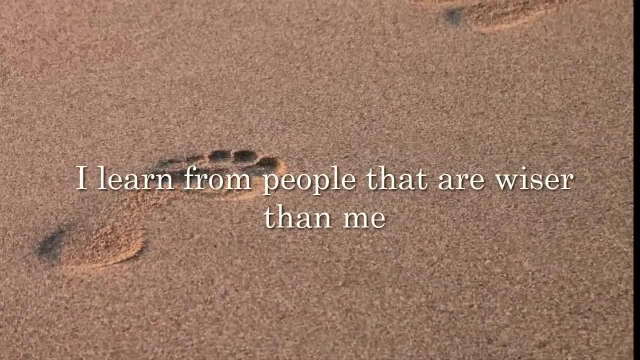 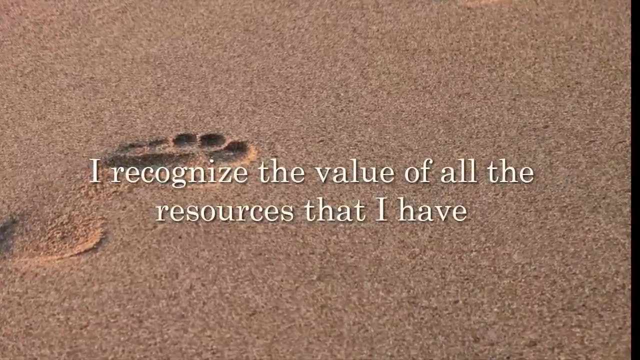 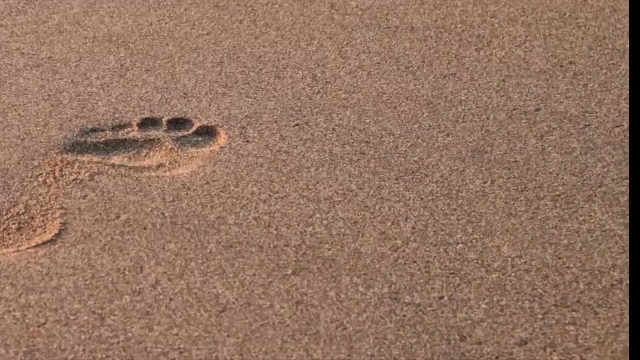 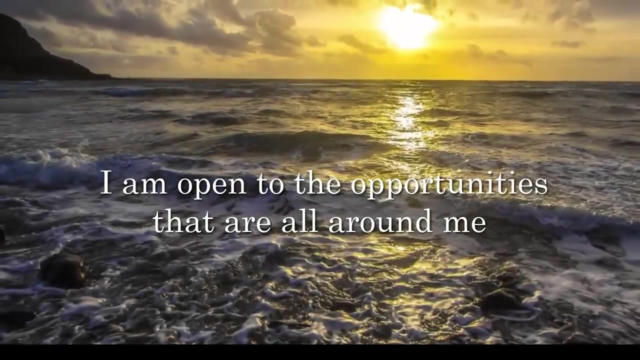 I learn from people that are wiser than me. I recognise the value of all the resources that I have. I am open to the opportunities that are all around me. I am open to the opportunities that are in front of me. I don't have to think about how I can bring people in. 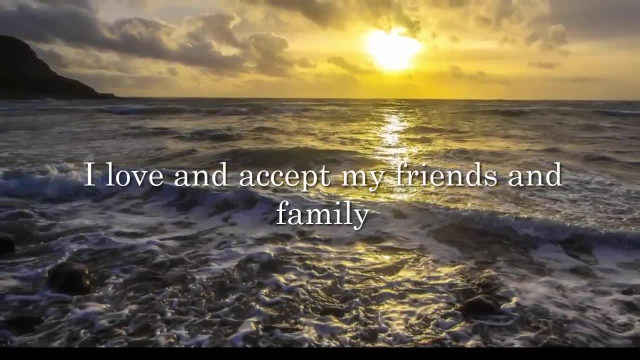 I'm like me. I am equal to me in every way, regardless of who I spend the time with, I don'tике when I help them. I am open to the opportunities that you give. I love and accept my friends and family. 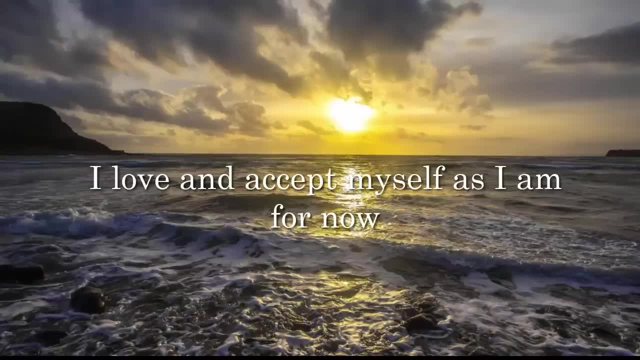 I love and accept myself as I am. now that I am who I am. I love and accept myself as I am, for now I am who I am. My time at home has been precious with each time, But I know that we need to be something different every day and every single day. 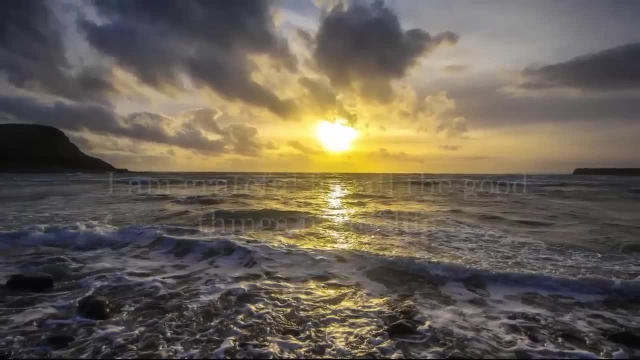 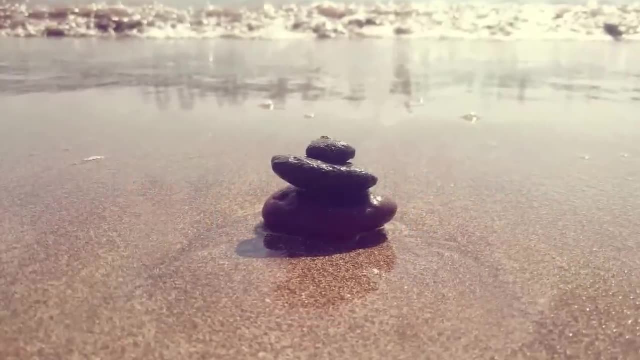 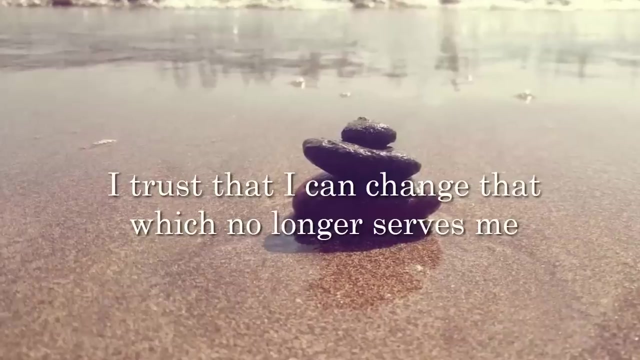 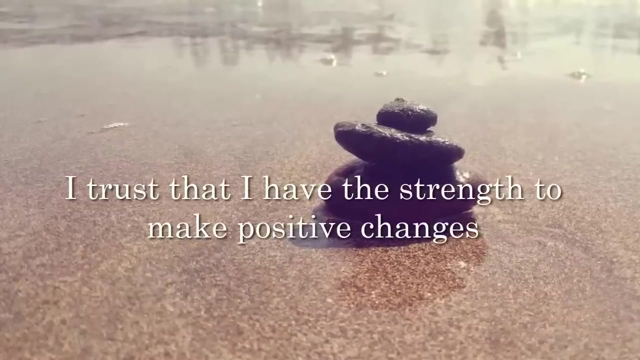 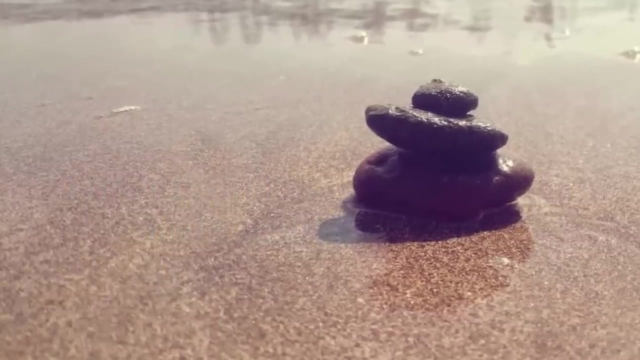 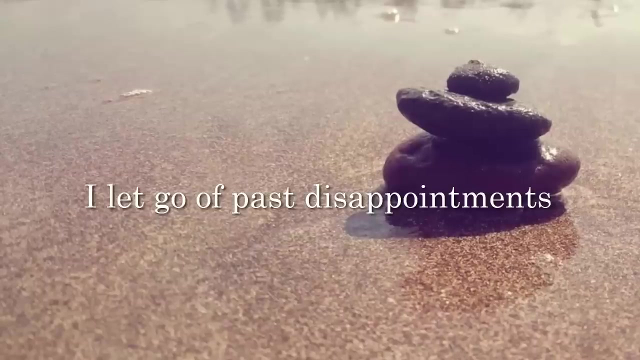 I am grateful for all the good things in my life. I trust that I can change that which no longer serves me. I trust that I have the strength to make positive changes. I let go of past disappointments. I trust in the wisdom of my higher mind. 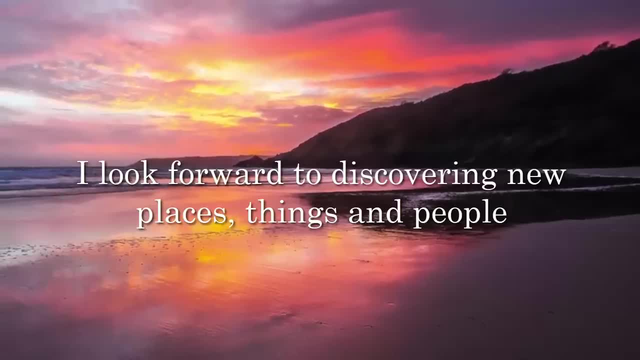 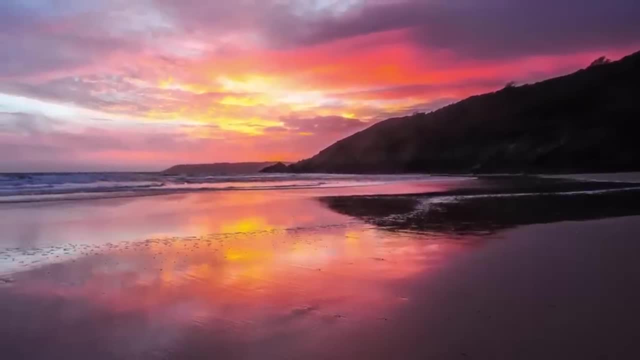 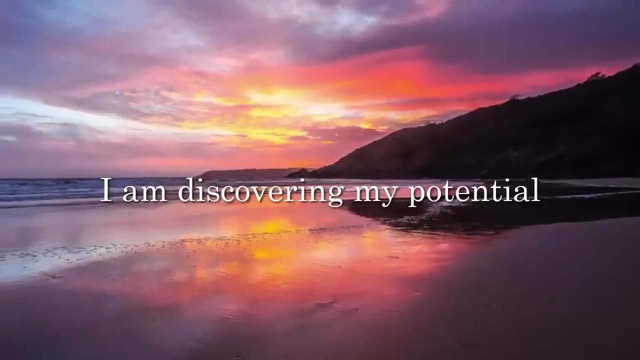 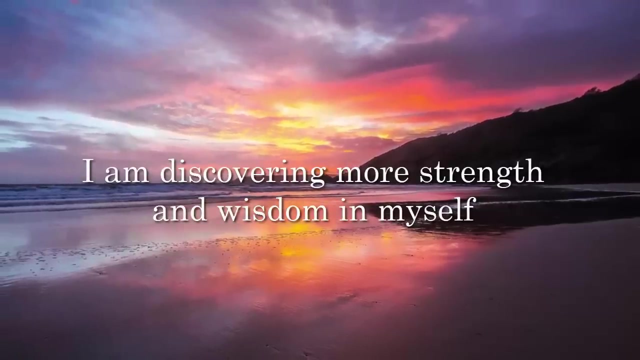 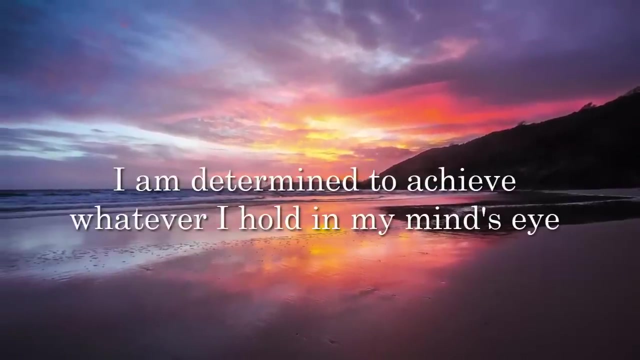 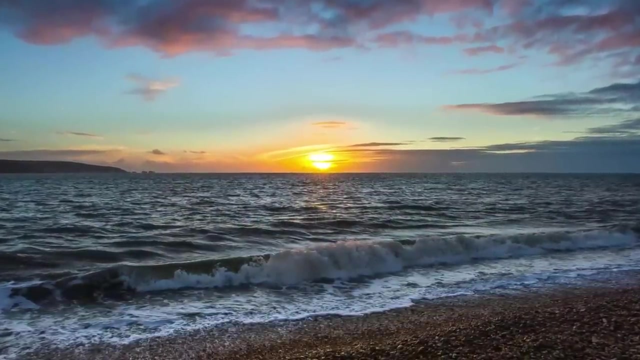 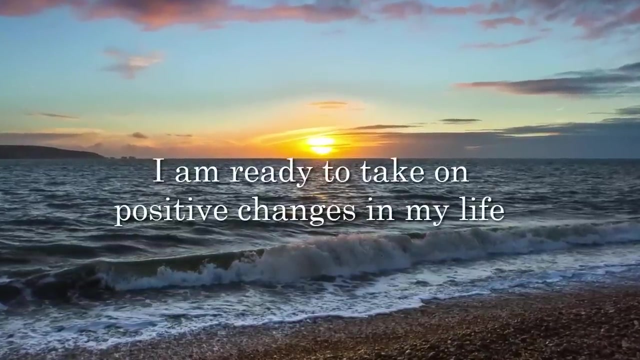 I look forward to discovering new places, things and people. I am discovering my potential. I am discovering more strength and wisdom in myself. I am determined to achieve whatever I hold in my mind's eye. I am ready to take on positive changes in my life. 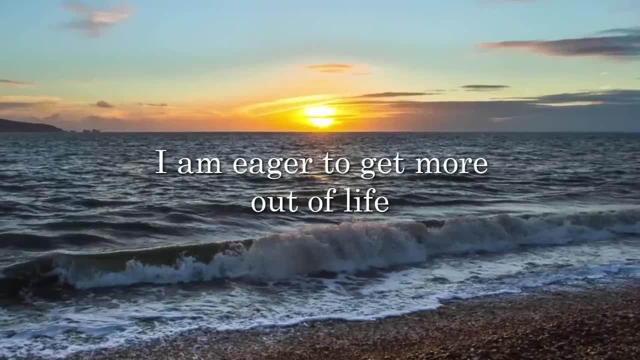 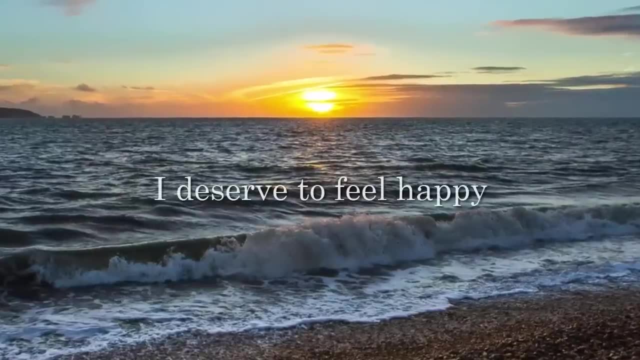 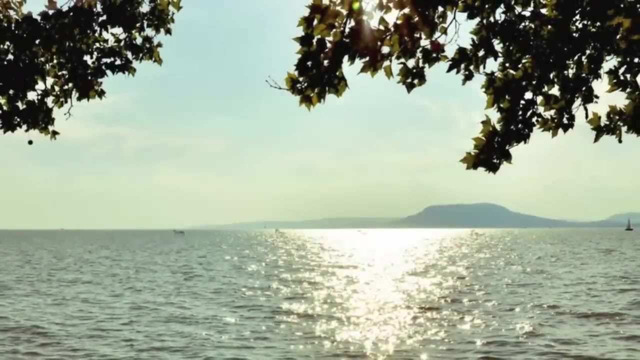 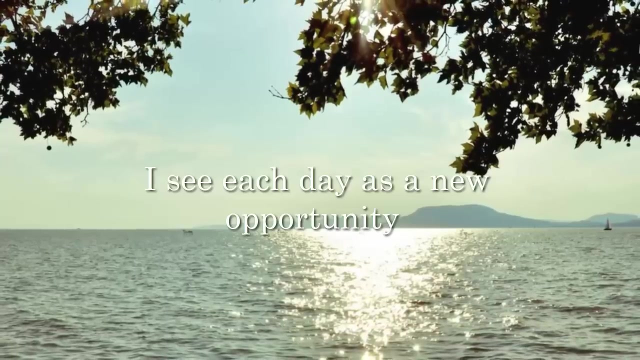 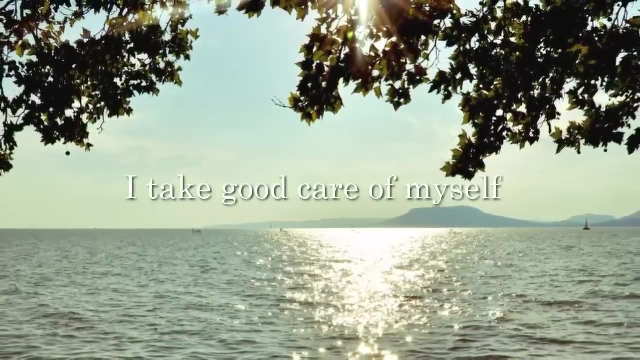 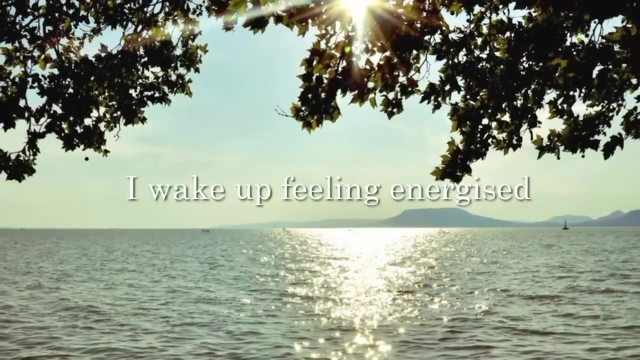 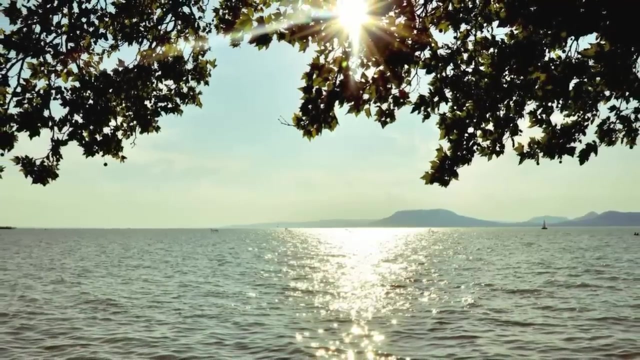 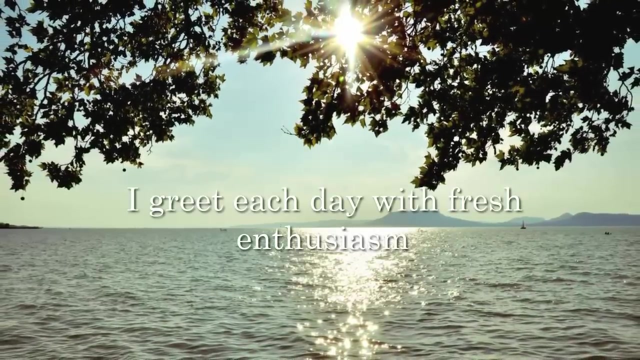 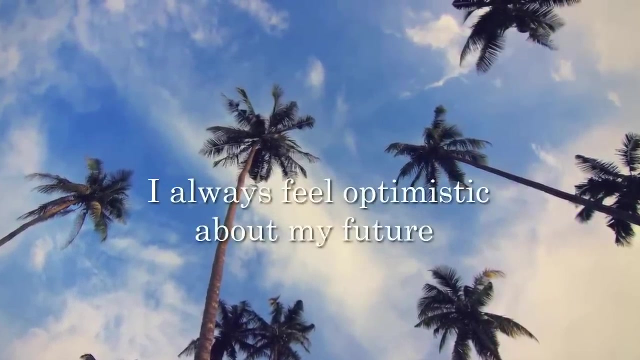 I am eager to get more out of life. I deserve to feel happy. I see each day as a new opportunity. I take good care of myself. I wake up feeling energized. I greet each day with fresh enthusiasm. I always feel optimistic about my future. 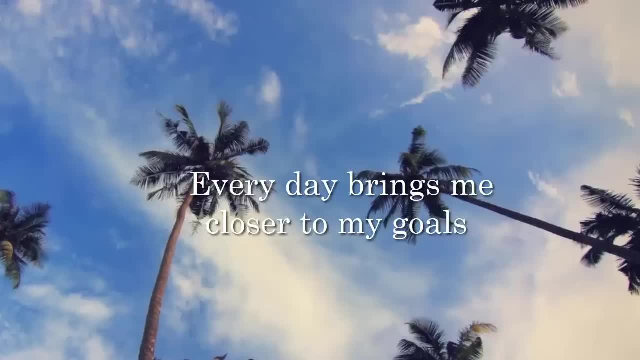 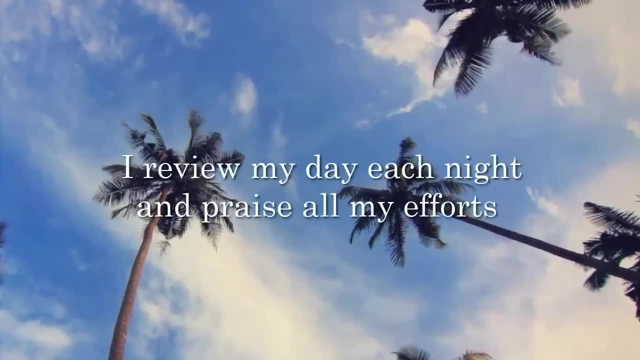 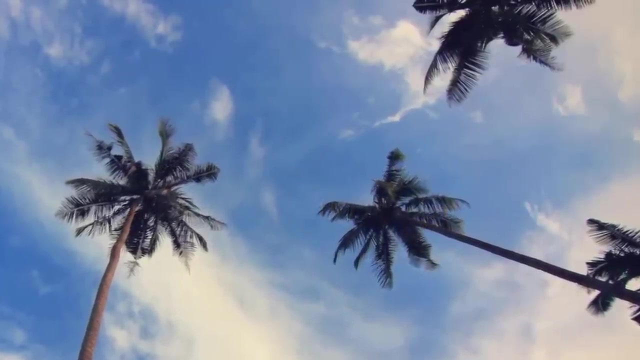 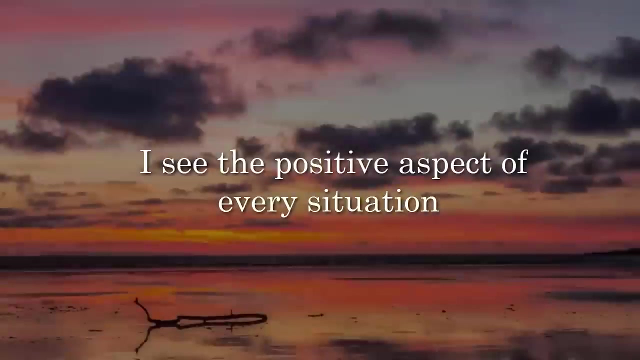 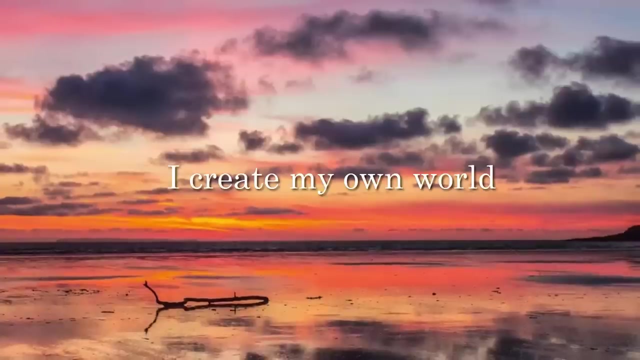 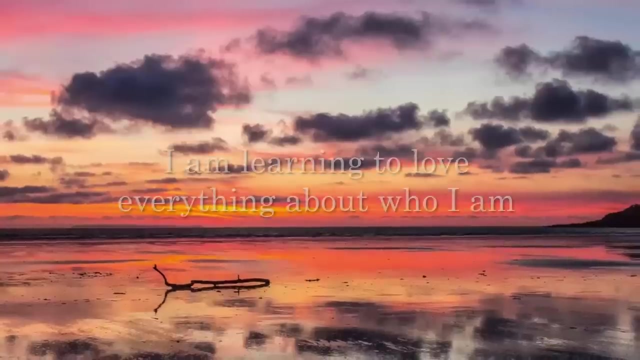 Every day brings me closer to my goals. I review my day each night and praise all my efforts. I see the positive aspect of every situation. I create my own world. I am now learning to learn my education. I can be independent. I'm part of my community. 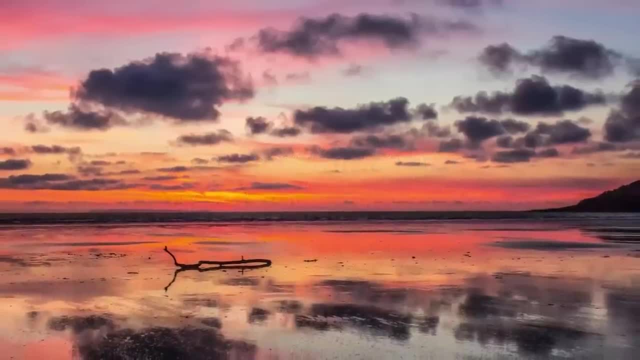 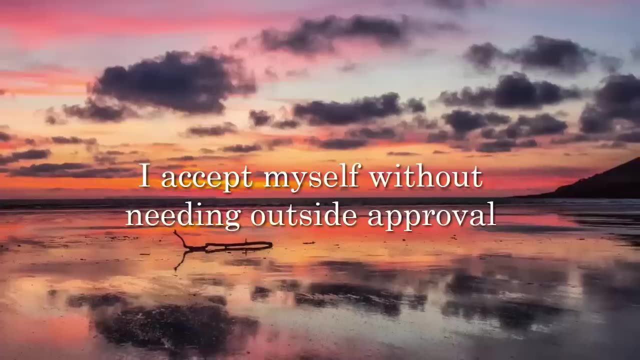 I can serve my community. I love not only myself, but my other self and I as one. If I want to be more understanding, I need to. I am ready to love. I'm learning to love everything about who I am. I accept myself without needing outside approval. 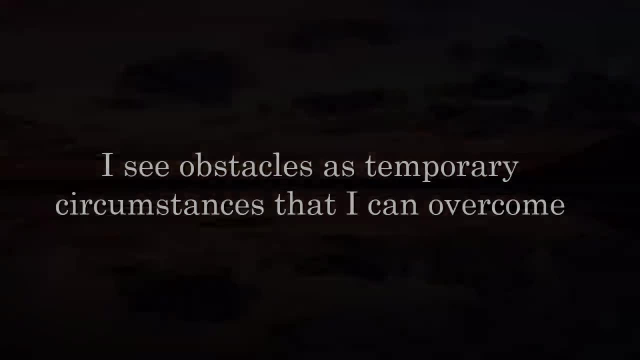 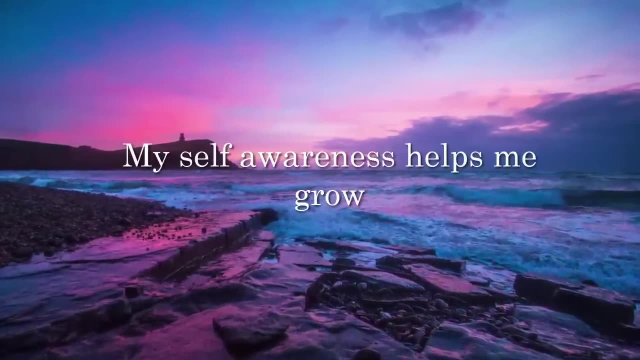 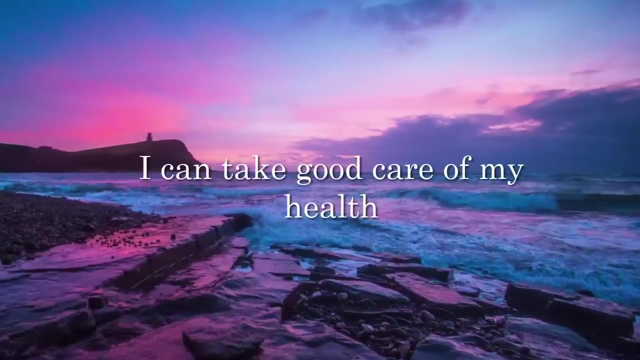 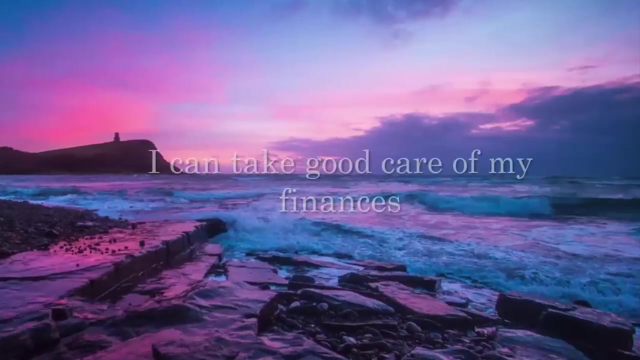 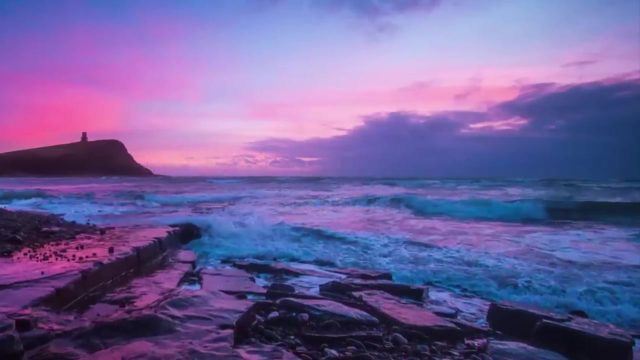 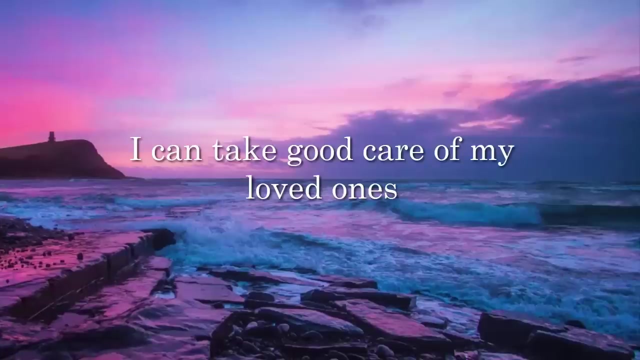 I love myself. I see obstacles as temporary circumstances that I can overcome. I learn to love. My self-awareness helps me grow. I can take good care of my health. I can take good care of my finances. I can take good care of my loved ones. 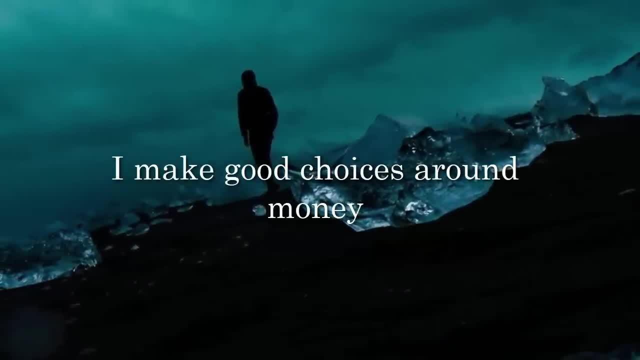 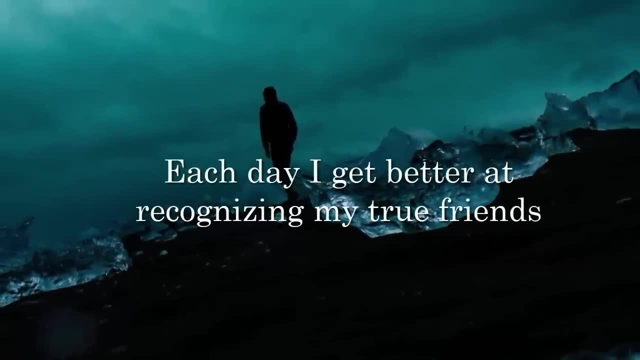 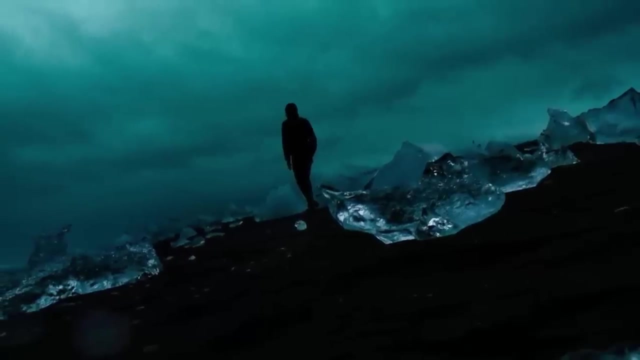 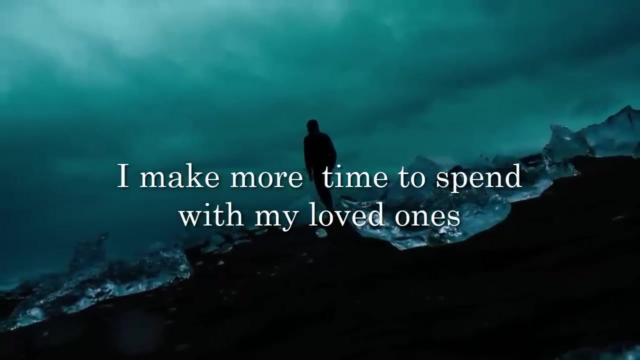 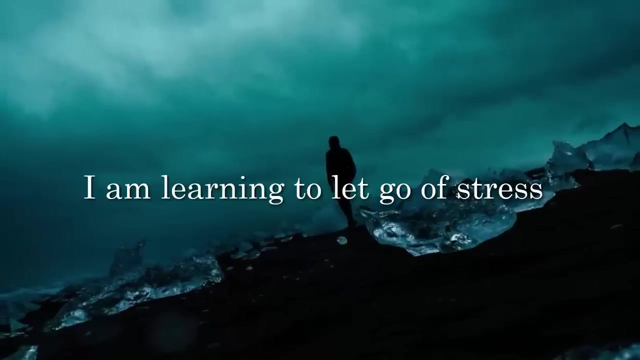 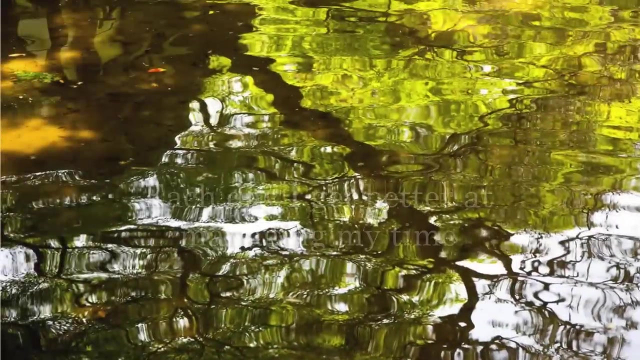 I make good choices around money. Each day, I get better at recognising my true friends. I make more choices around money. I have more time to spend with my loved ones. I am learning to let go of stress. Each day I get better at managing my time. 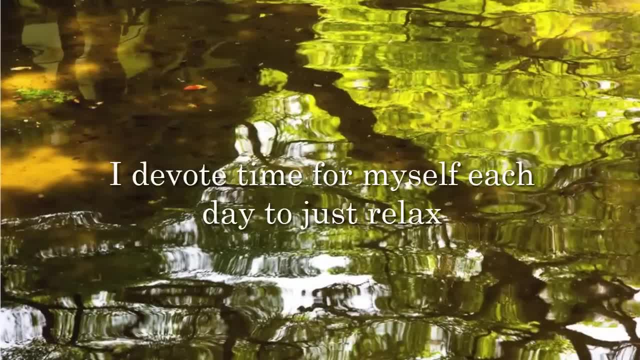 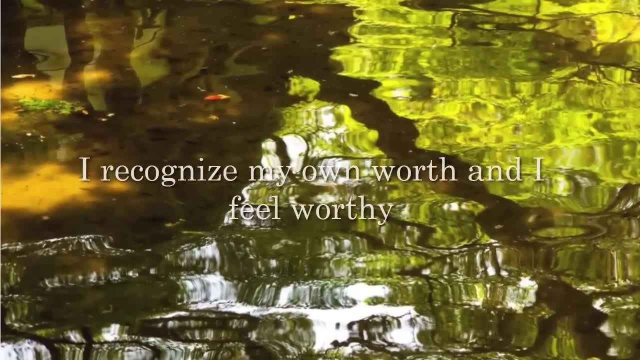 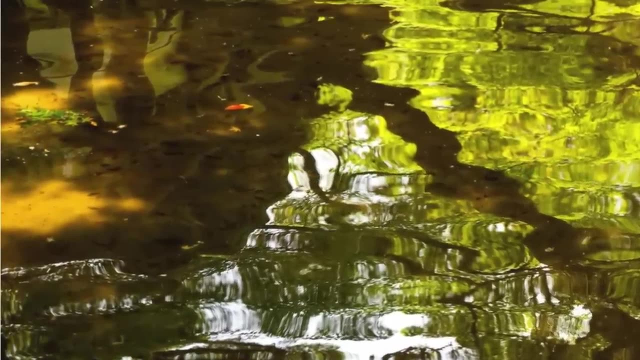 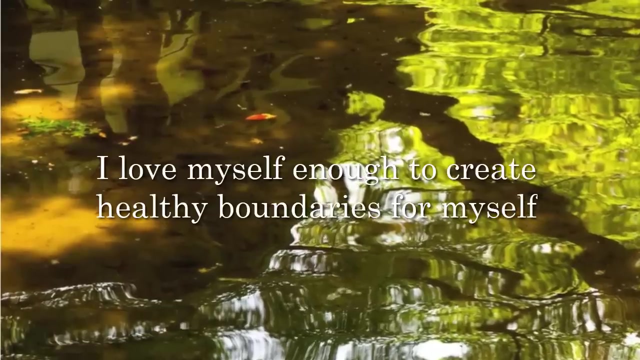 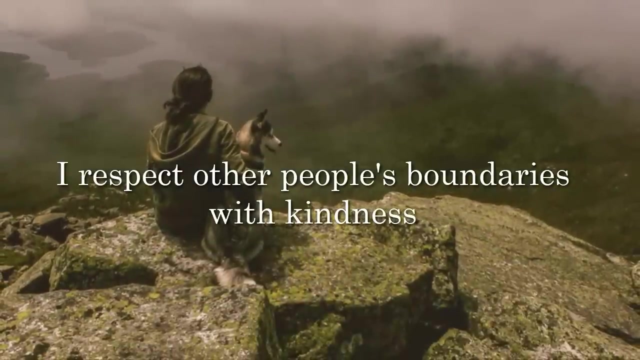 I devote time for myself each day. My self-awareness helps me out. in Australia, I look for different ways in which to just relax. I recognise my own worth and feel worthy. I love myself enough to create healthy boundaries for myself. I respect other people's boundaries with kindness. 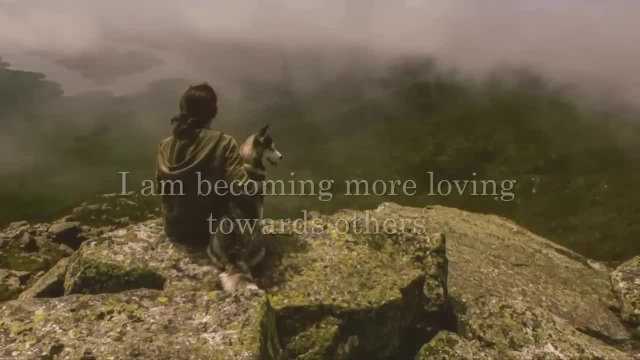 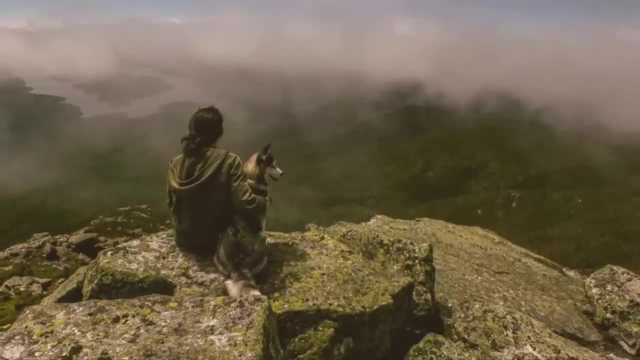 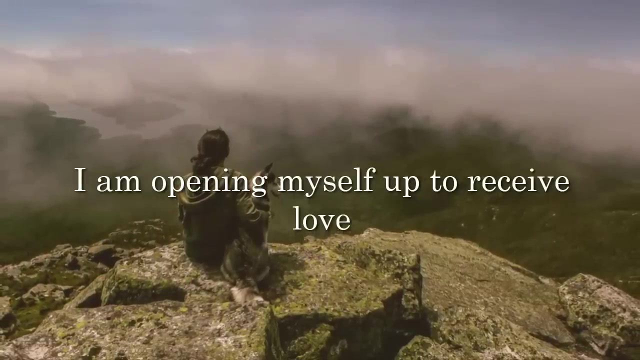 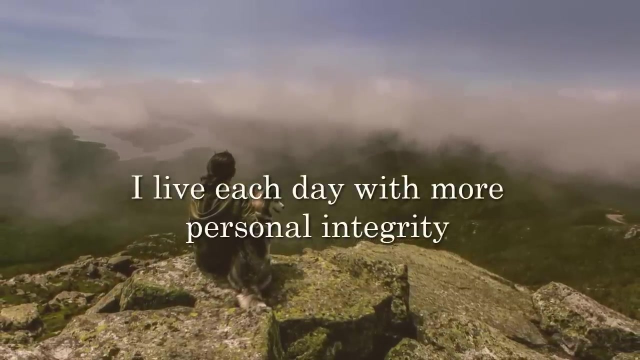 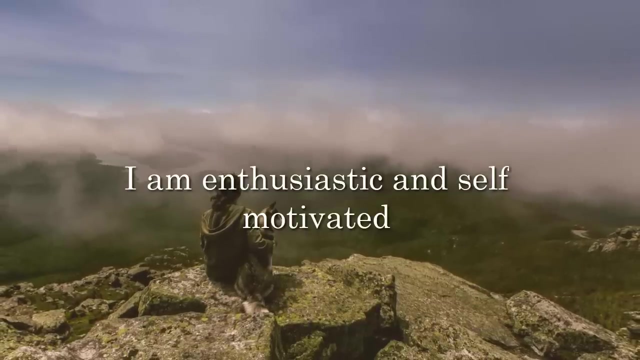 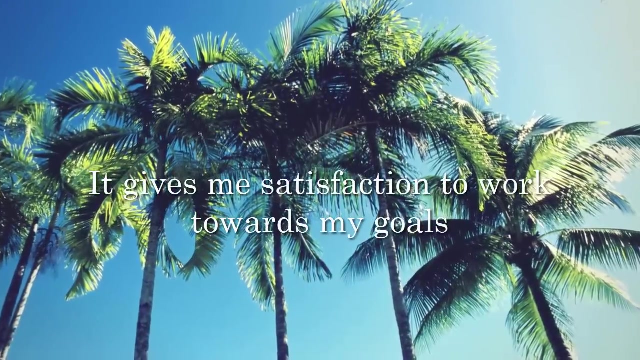 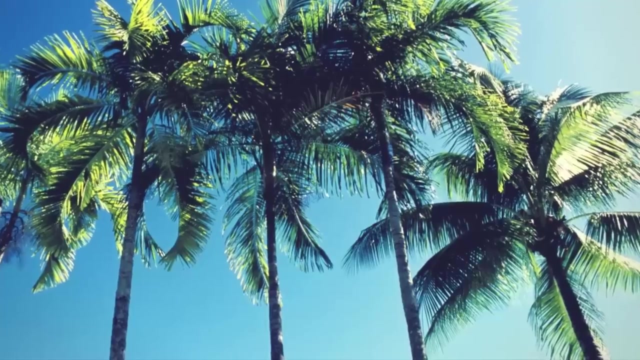 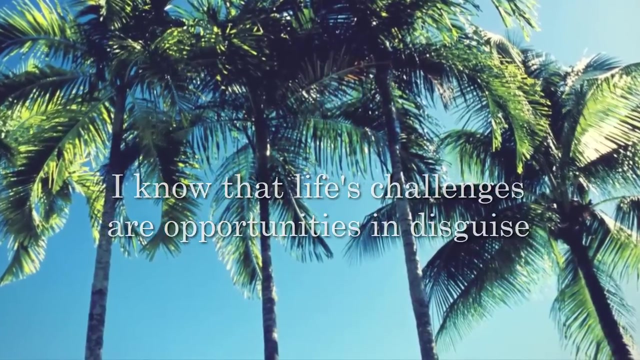 I am becoming more loving towards others. I am opening myself up to receive love. I live each day with more personal integrity. I am enthusiastic and self-motivated. It gives me great satisfaction to work towards my goals. I know that life's challenges are opportunities in disguise. 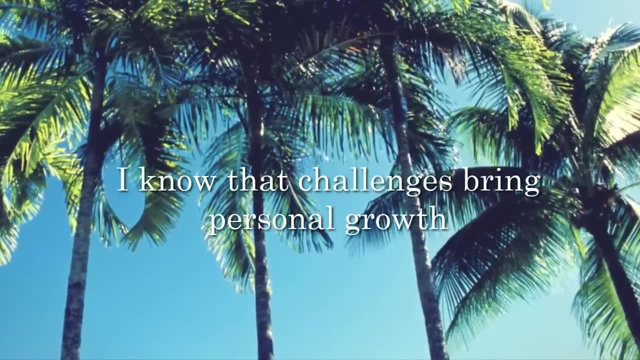 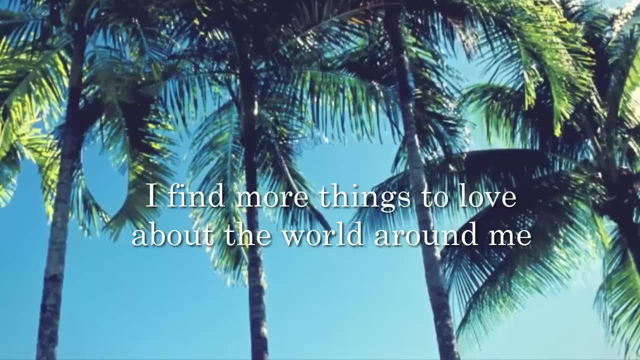 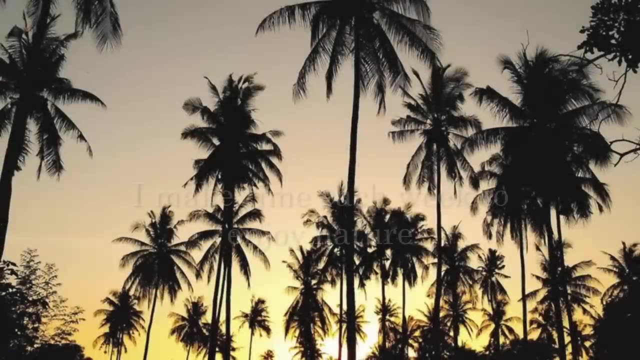 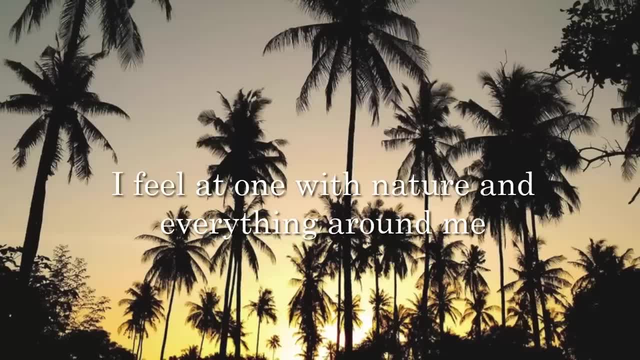 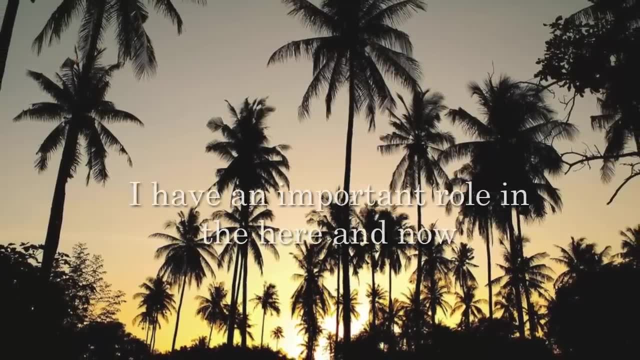 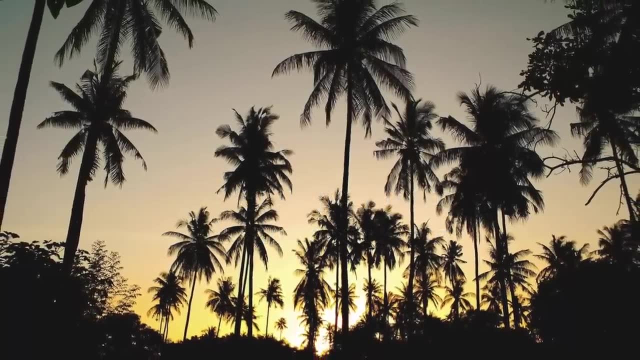 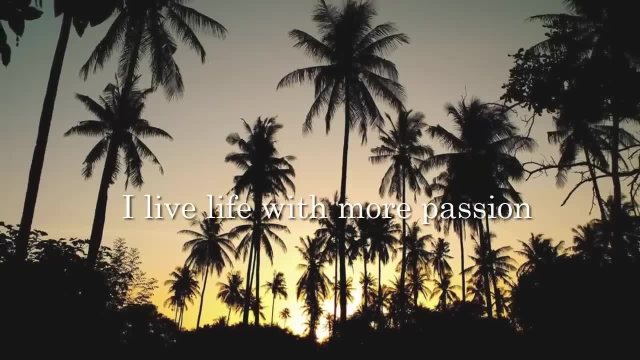 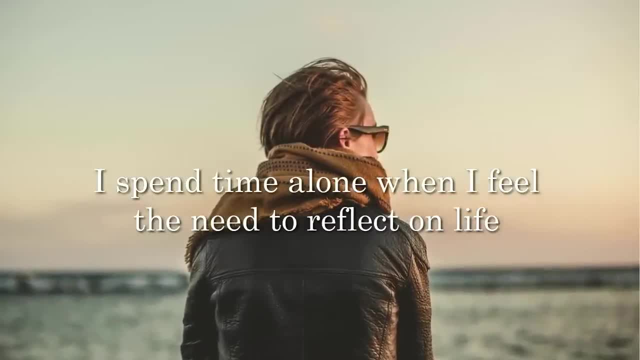 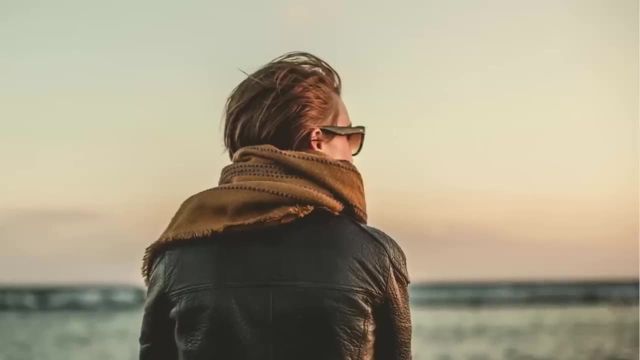 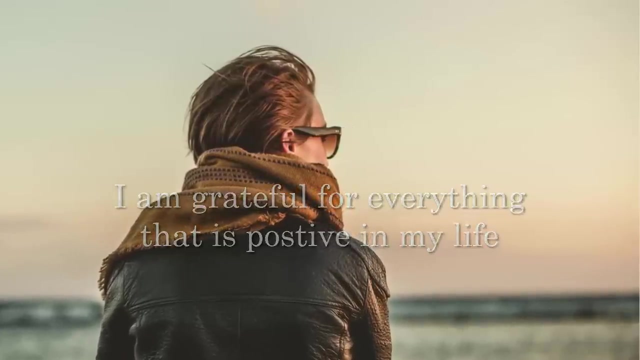 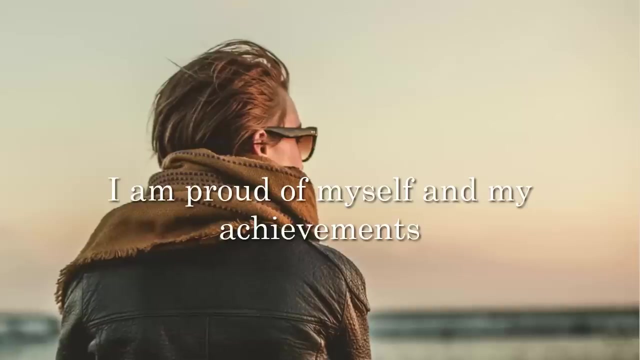 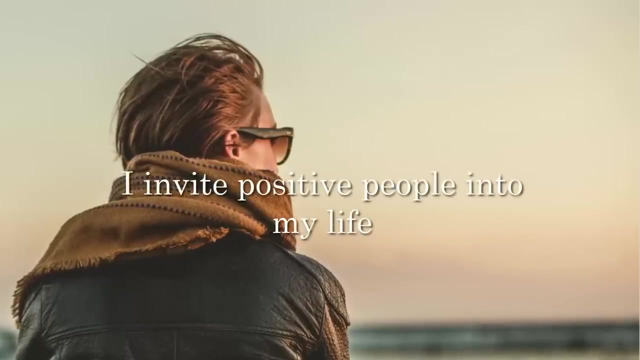 I spend time alone when I feel the need to reflect on my life. I spend time alone when I feel the need to reflect on my life. I am grateful for everything that is positive about my life. I am proud of myself and my achievements. I invite positive people into my life. 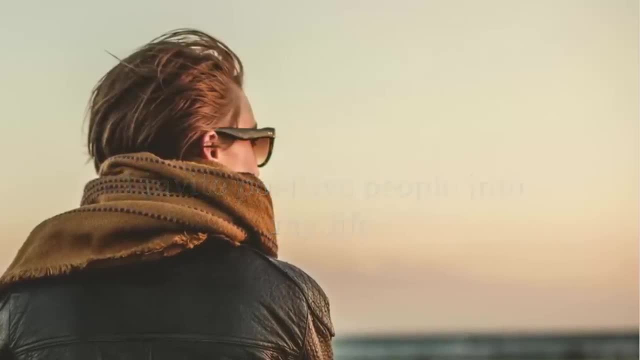 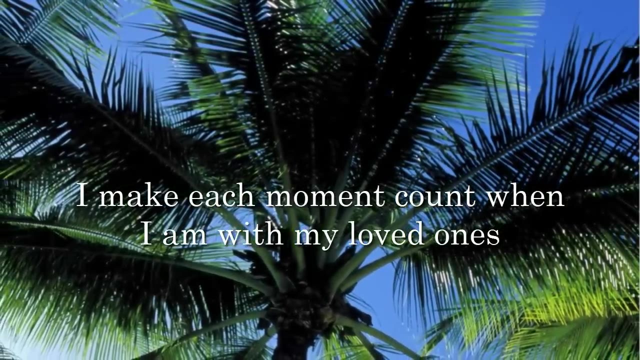 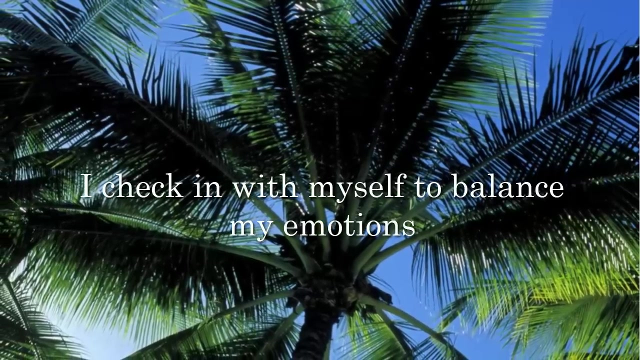 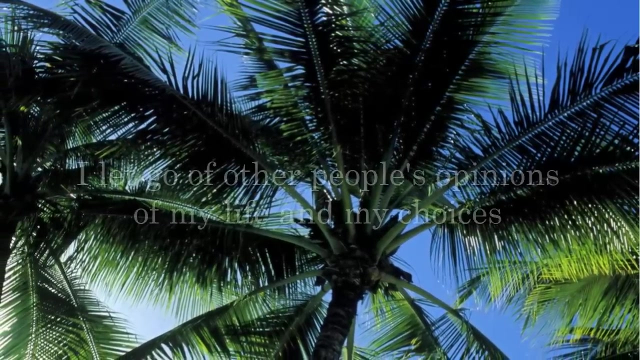 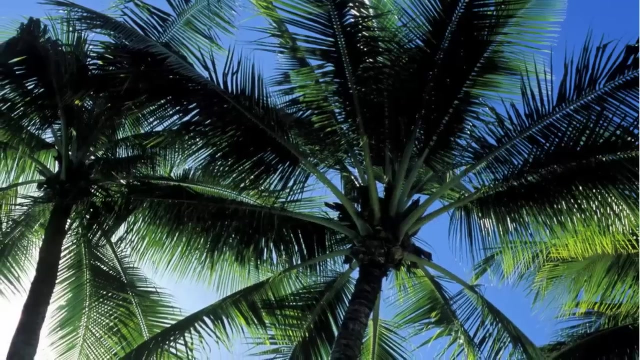 I make each moment count. when I'm with my loved ones. I am grateful for everything that is positive about my life. I check in with myself to balance my emotions. I let go of other people's opinions of my life and my choices. I have the wisdom and courage. 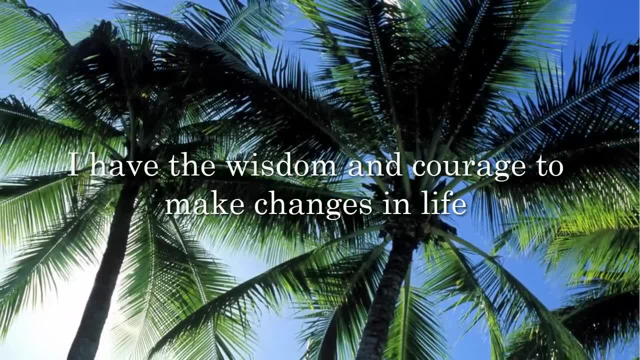 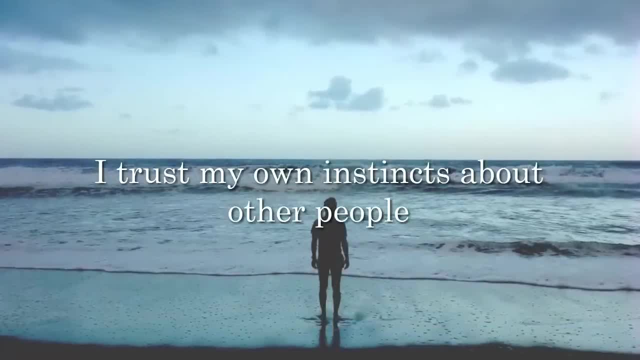 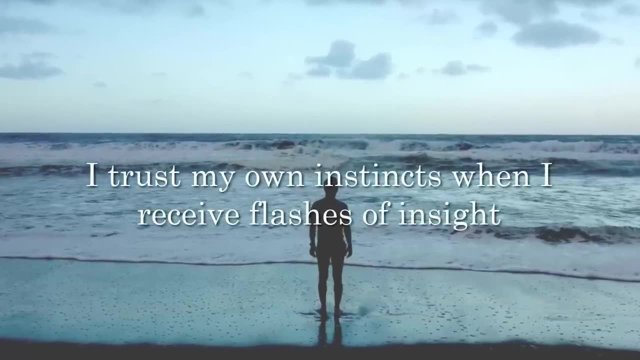 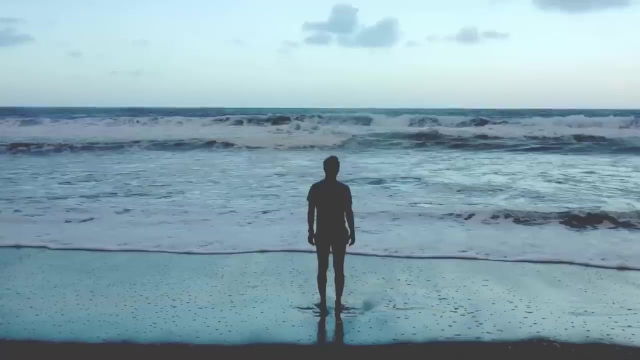 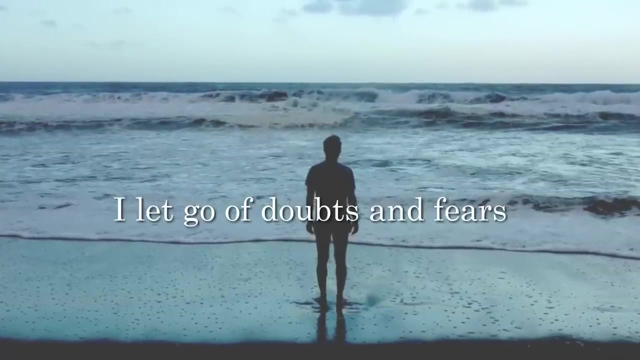 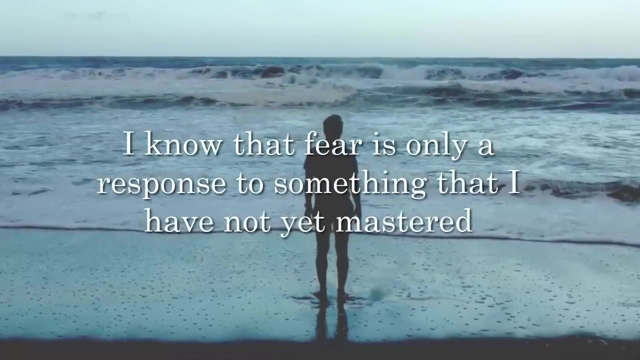 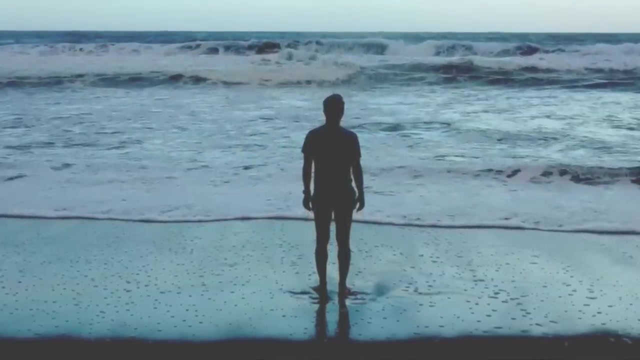 to make changes in life. I trust my own instincts about other people. I trust my own instincts when I receive flashes of insight. I let go of doubts and fears. I trust my own instincts about other people. I know that fear is only a response to something I have not yet mastered. 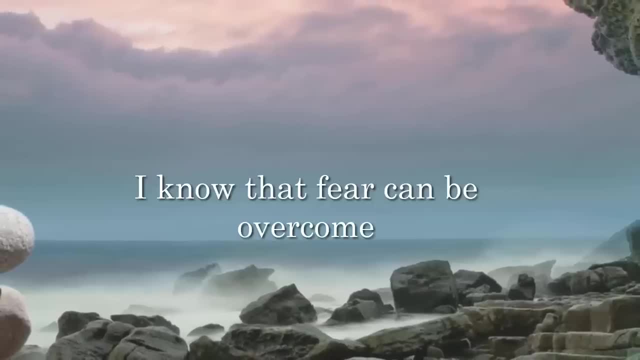 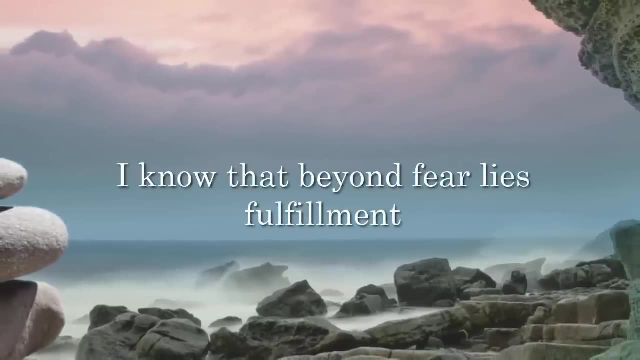 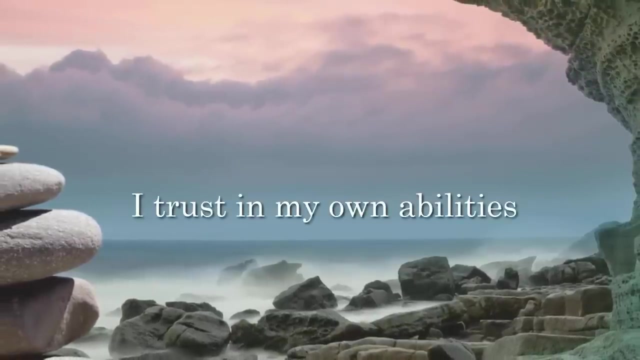 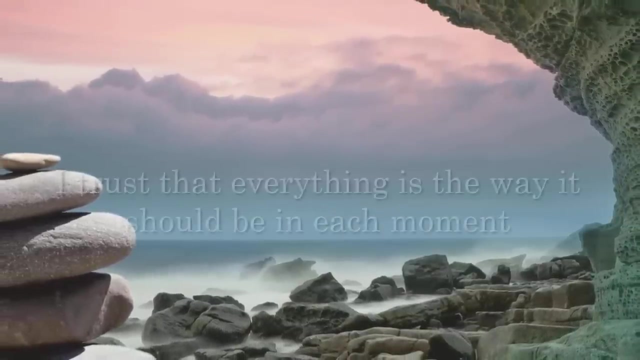 I know that fear can be overcome. I trust my own instincts about other people. I trust mine instincts about others. I trust my own instincts about other people by responding to forgotten questions, by correcting suffrage. I trust in my own investments by usingorký Creatures own abilities. 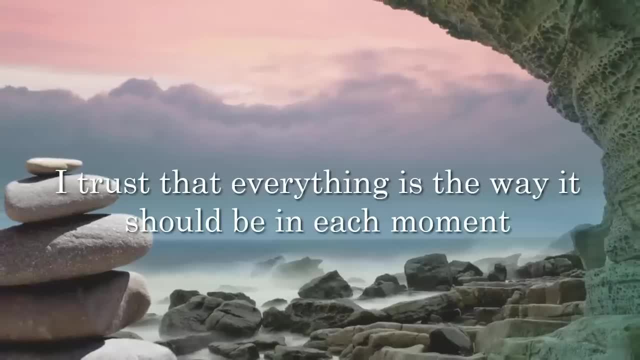 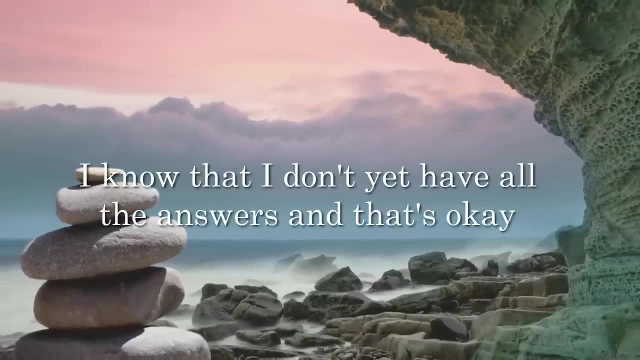 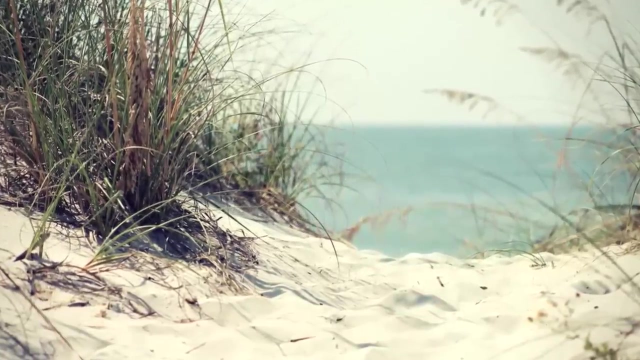 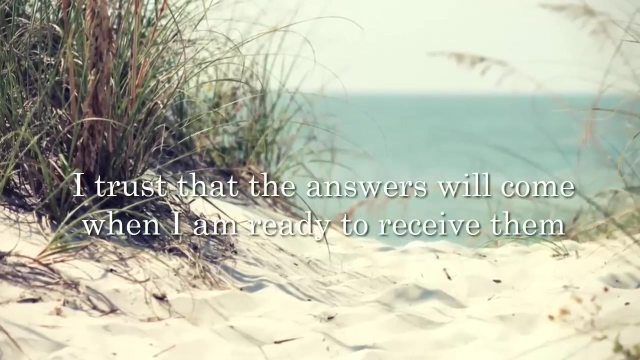 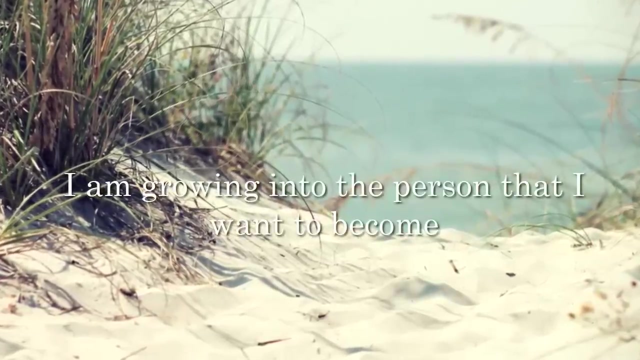 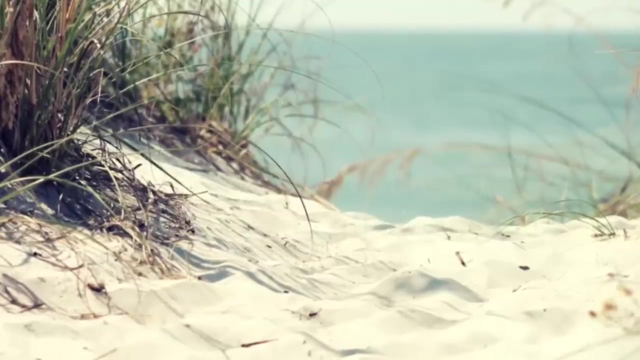 I trust that everything is the way it should be in each moment. I know that I don't yet have all the answers and that it's okay. I trust that the answers will come when I'm ready to receive them. I'm growing into the person I want to become. 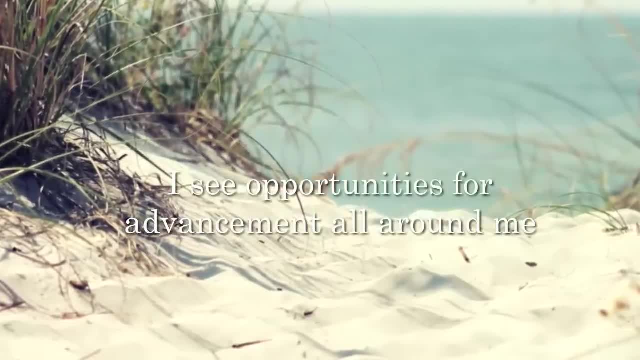 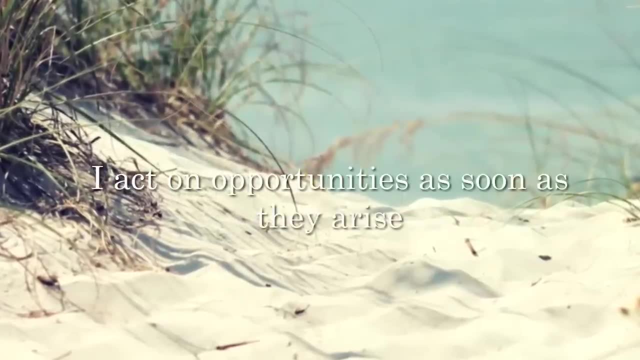 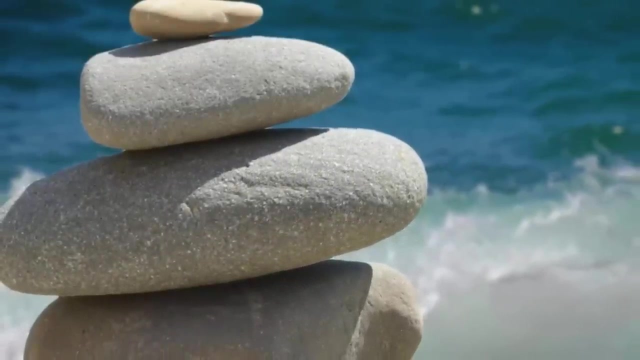 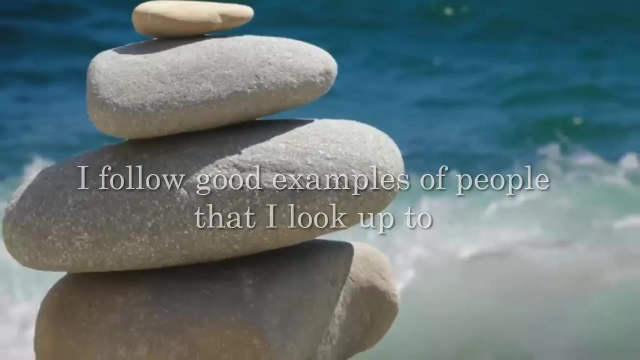 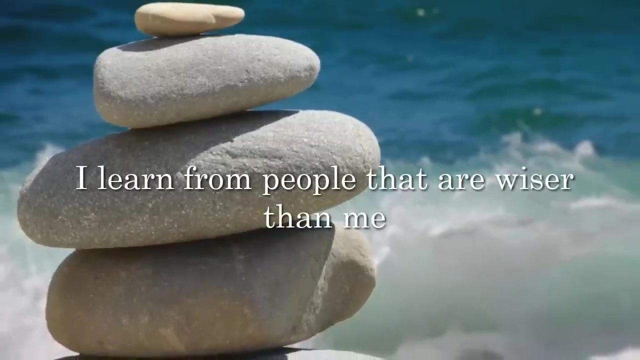 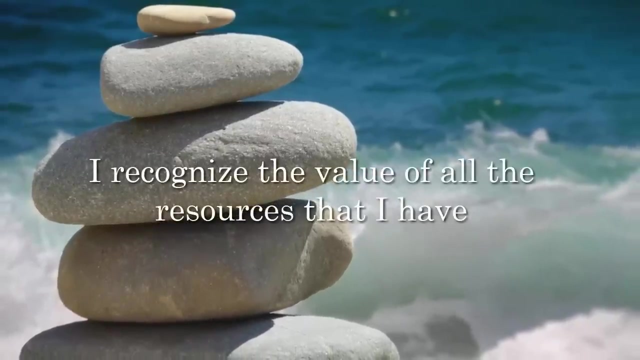 I see opportunities for advancement all around me. I act on opportunities as soon as I can. I follow good examples of people that I look up to. I learn from people that are wiser than me. I recognize the value of all the resources that I have. 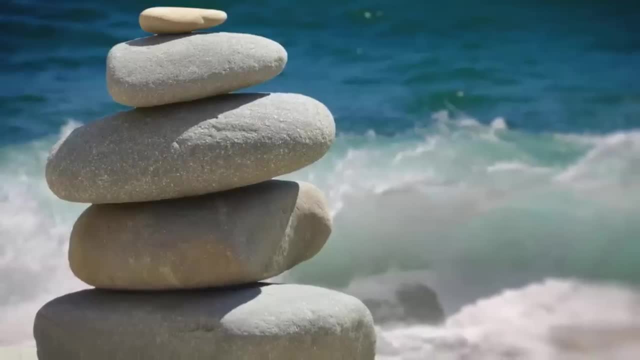 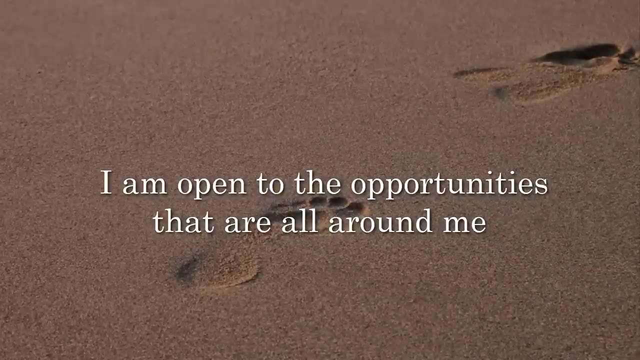 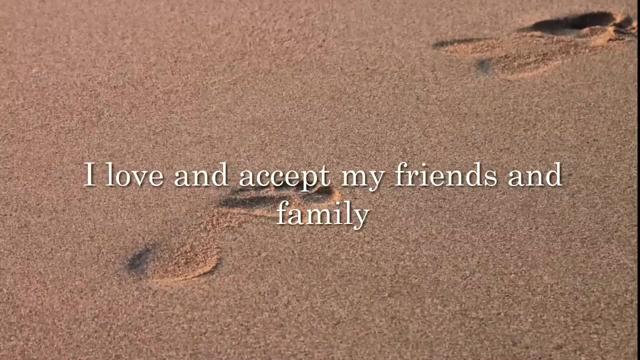 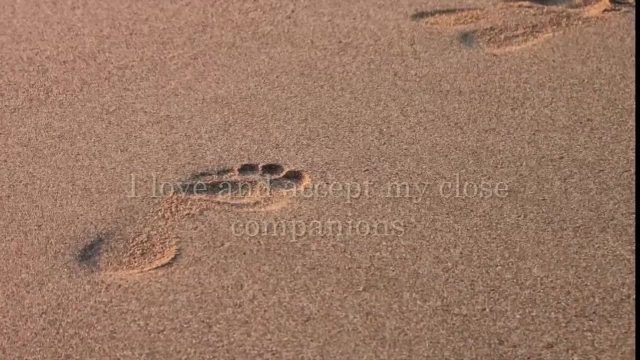 I am open to the opportunities that are all around me. I love and accept my friends and family. I love and accept my close companions. I love and accept my family. I love and accept my friends and family. I love and accept my family. 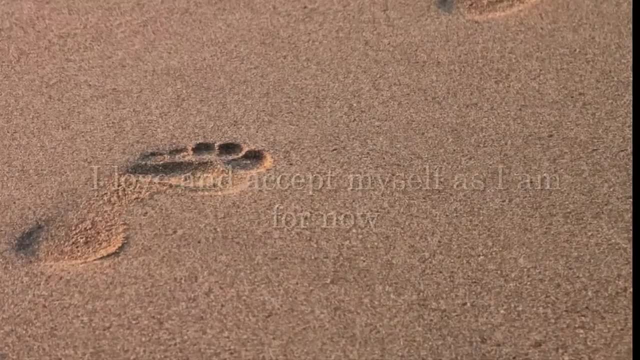 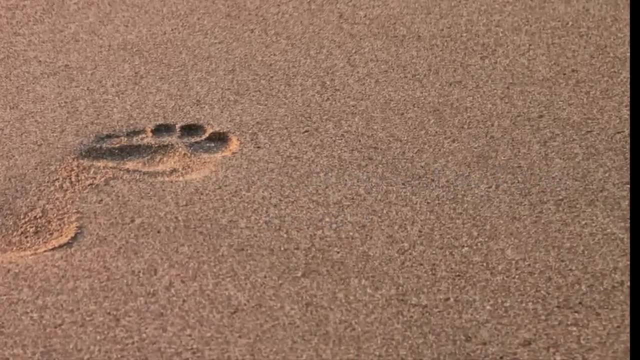 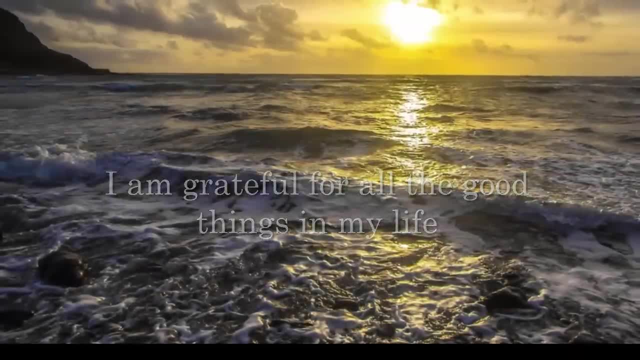 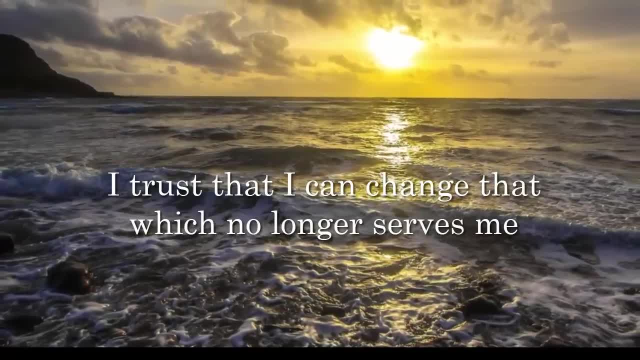 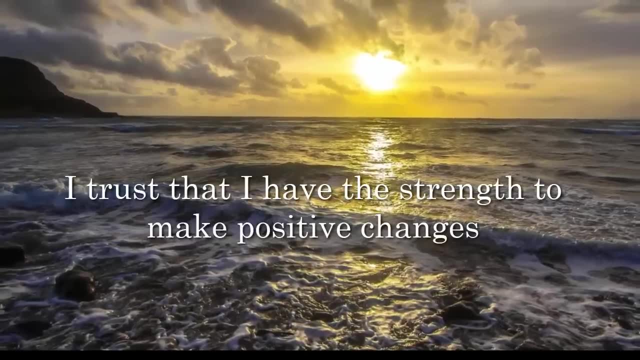 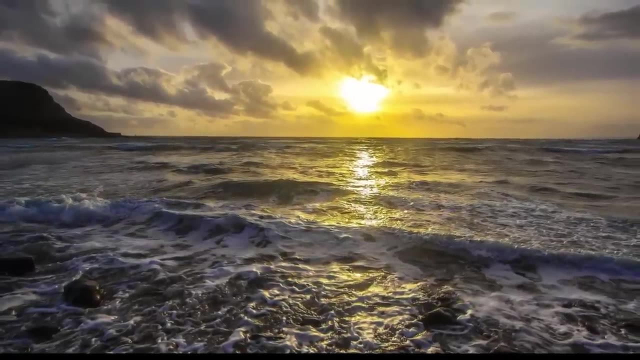 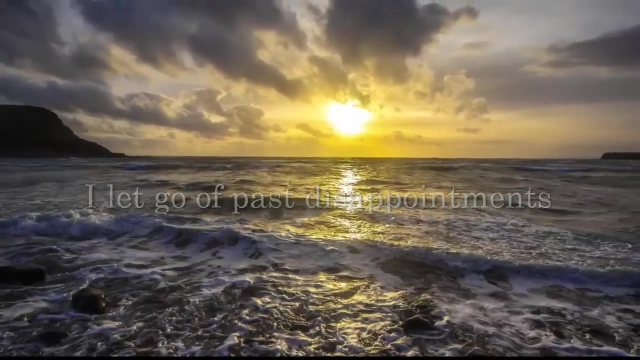 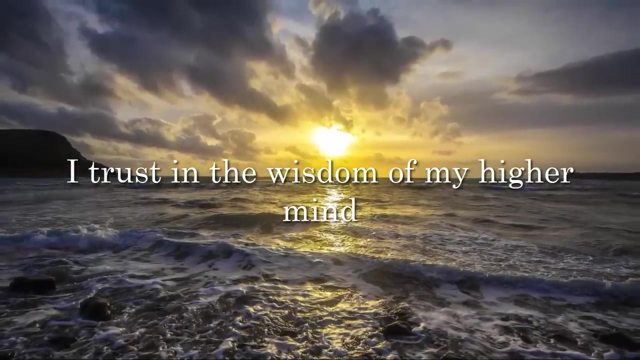 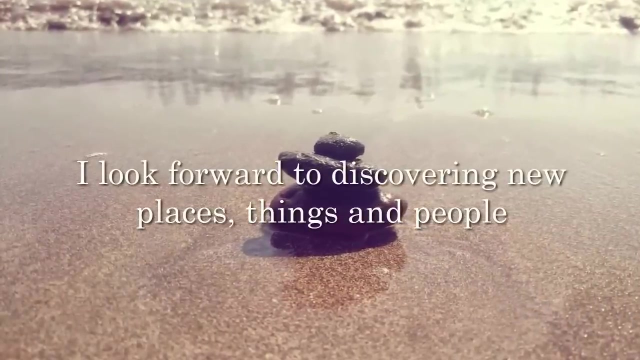 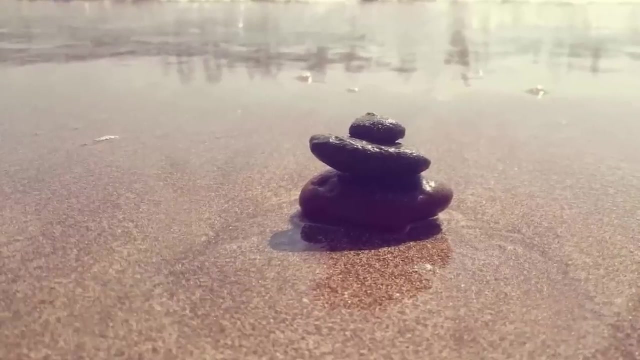 that which no longer serves me. I trust that I have the strength to make positive changes. I let go of past disappointments. I trust in the wisdom of my higher mind. I look forward to discovering new places, things and people. I am discovering my potential. 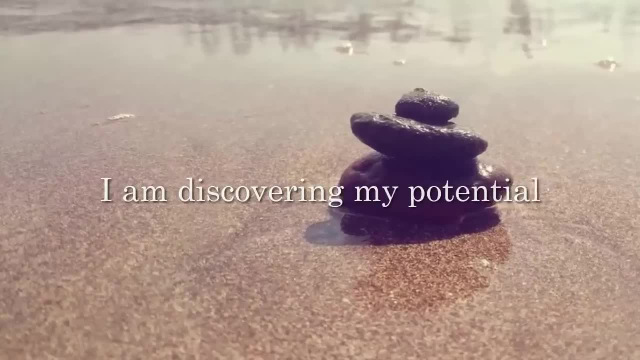 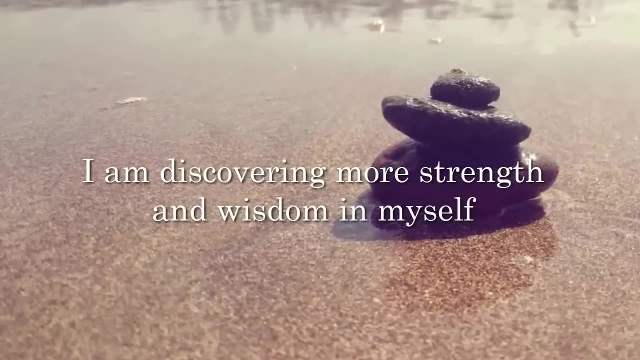 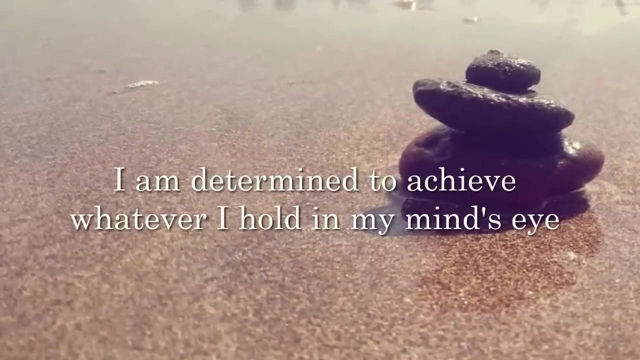 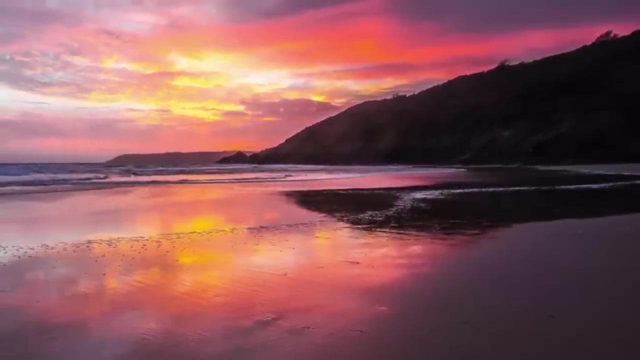 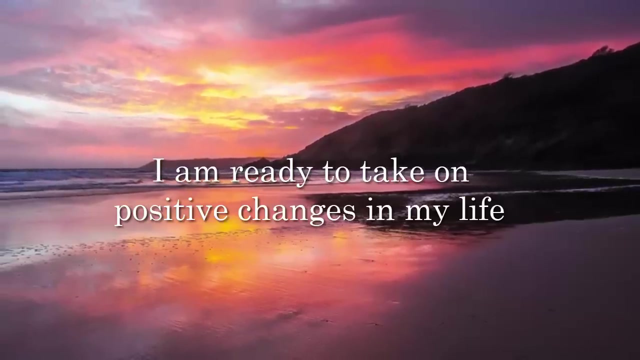 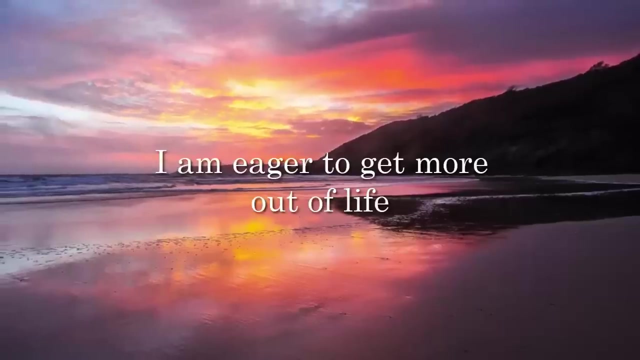 I am discovering more strength and wisdom in myself. I am determined to achieve whatever I hold in my mind's eye. I am ready to take on positive changes in my life. I am ready to take on positive changes in my life. I am eager to get more out of life. 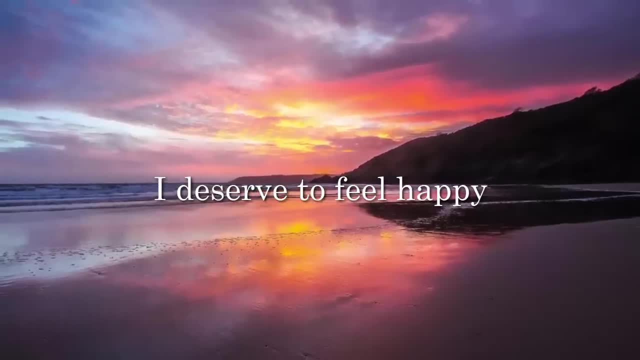 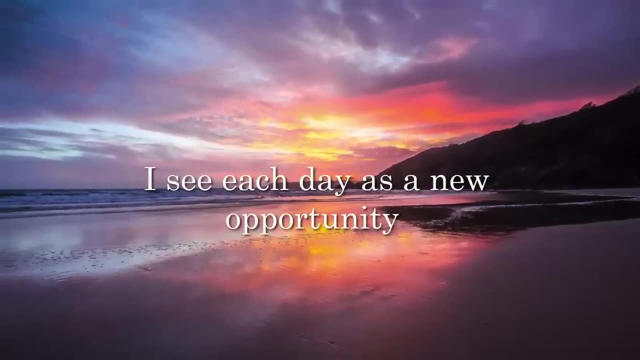 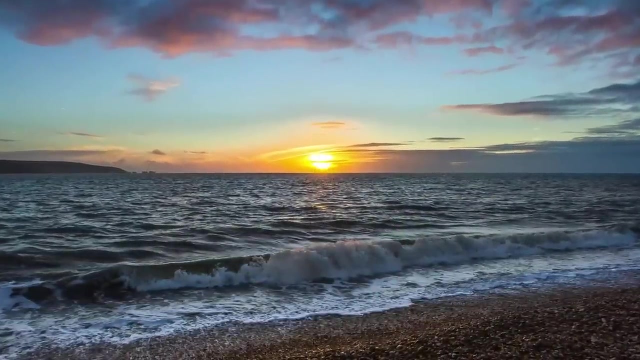 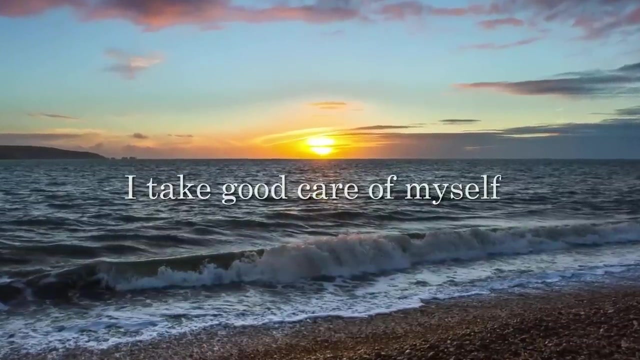 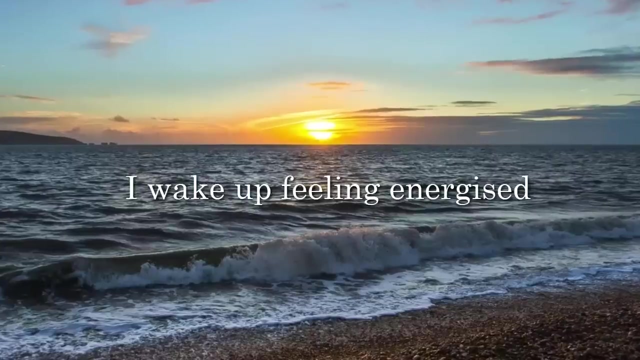 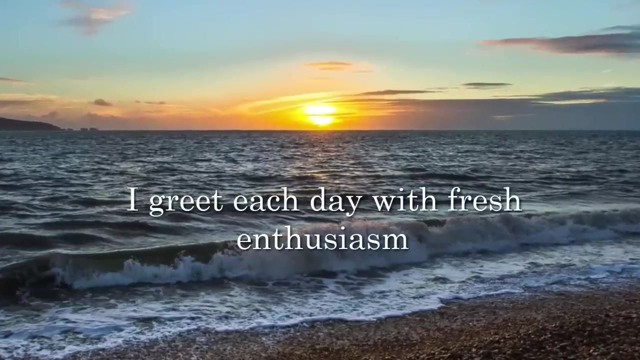 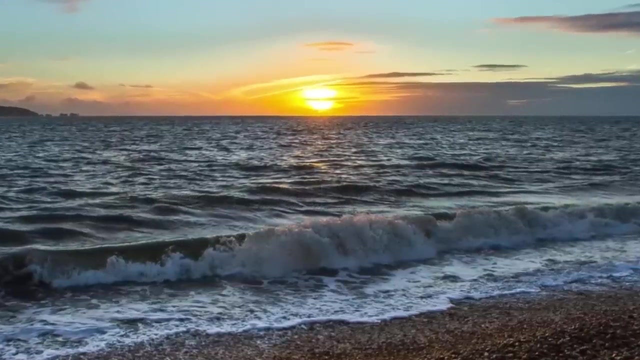 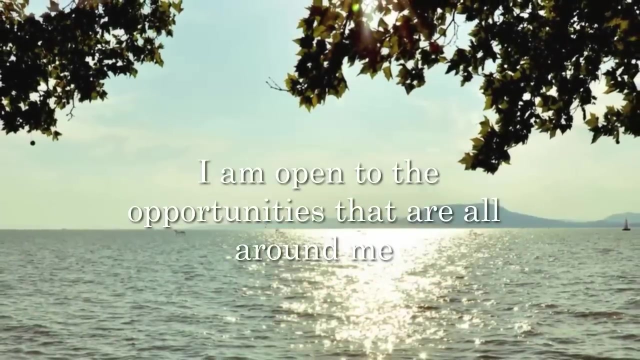 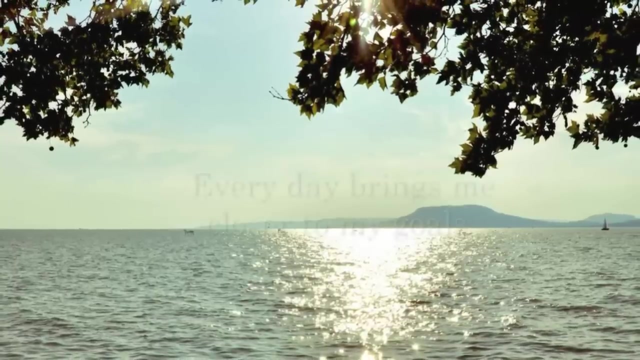 I deserve to feel happy. I see each day as a new opportunity. I take good care of myself. I wake up feeling energised. I greet each day with fresh enthusiasm. I always feel optimistic about my future. Every day brings me closer to my goals. 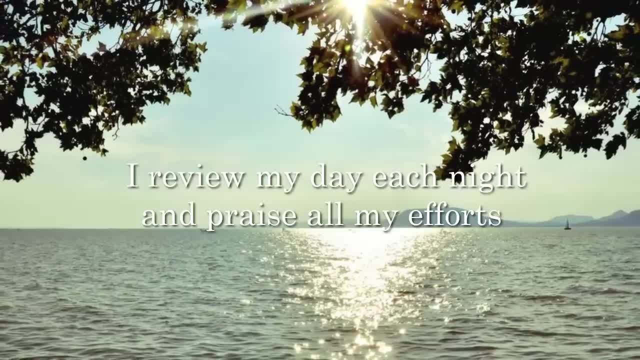 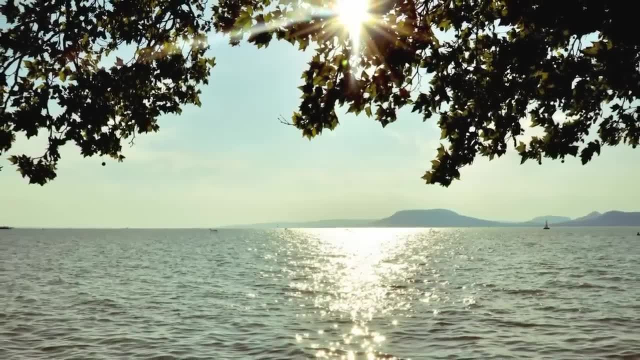 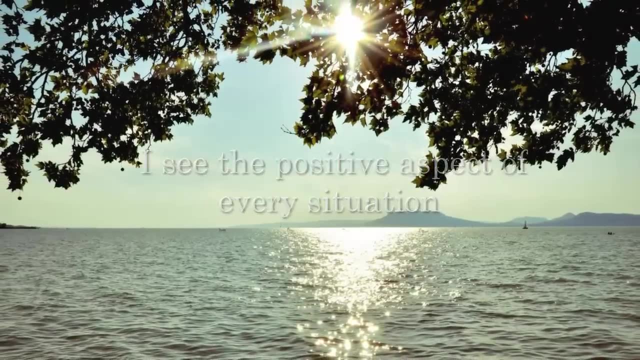 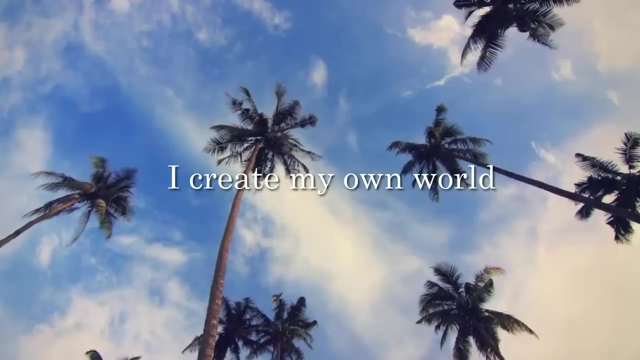 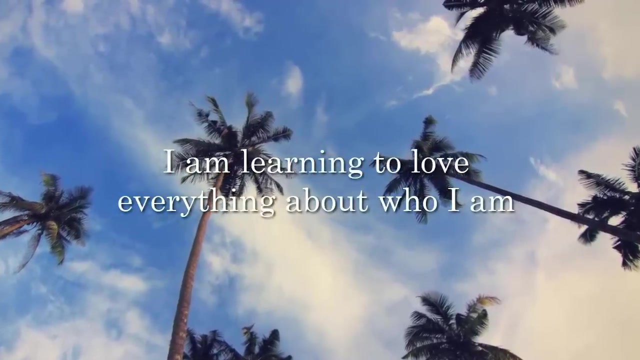 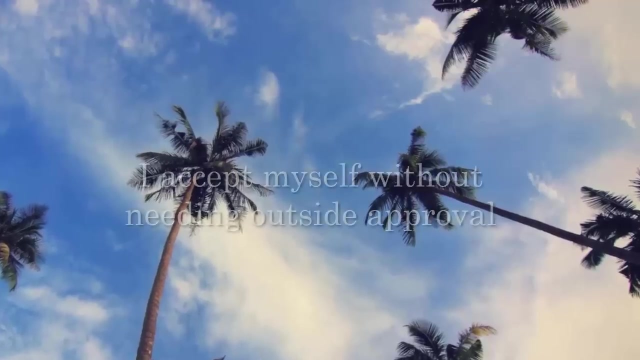 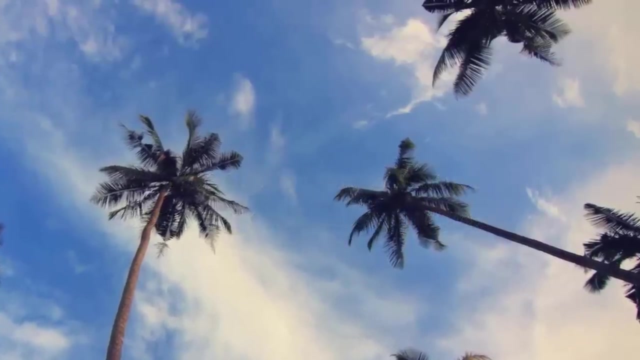 I review my day each night and praise all my efforts. I almost cannot explain what changes I have made. I see every possible situation. I see inner well-being. I love others. I do everything for their self. I accept myself without needing outside approval. I see obstacles as temporary. 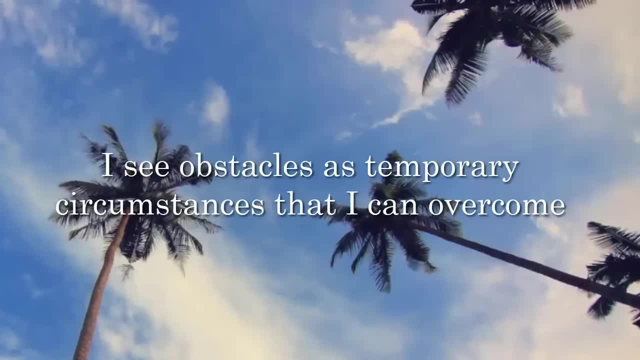 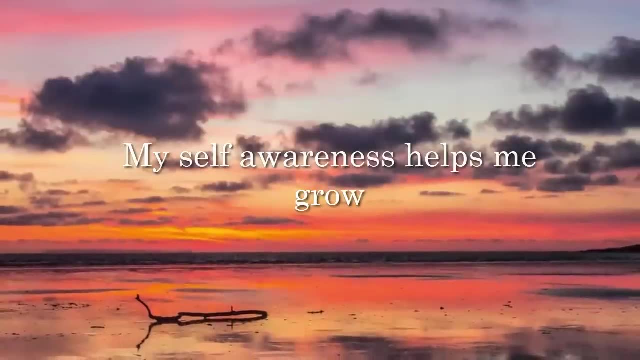 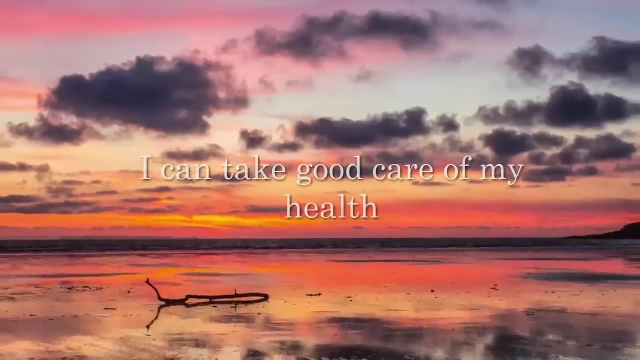 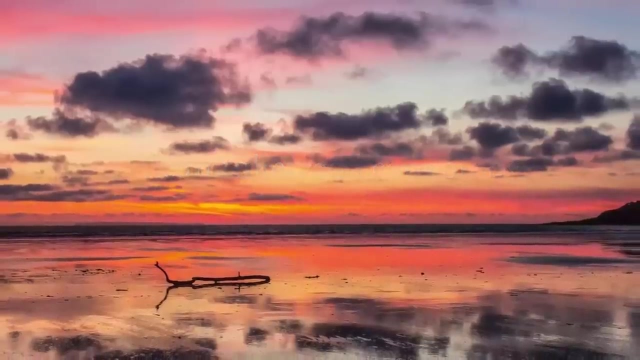 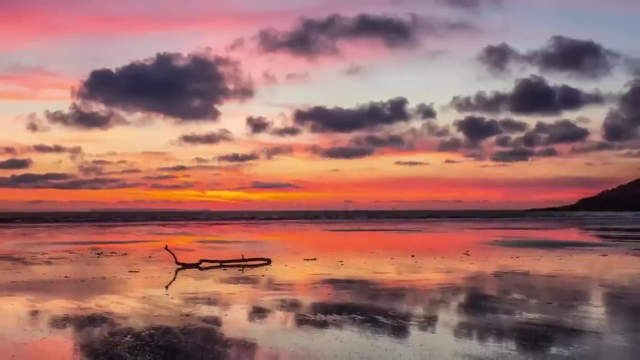 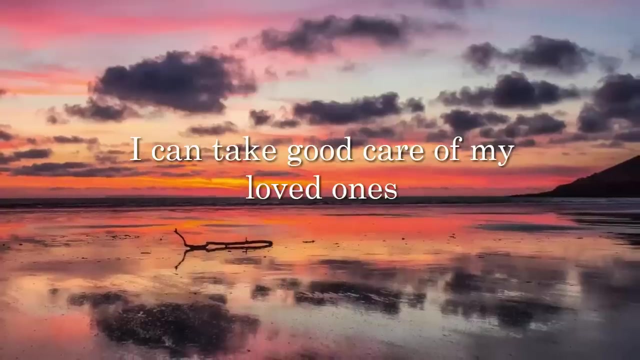 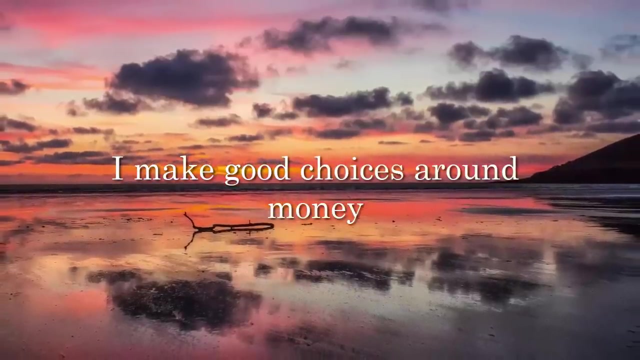 circumstances that I can overcome. my self-awareness helps me grow. I can take good care of my health. I can take good care of my finances. I can take good care of my loved ones. I make good choices. I make good choices. I make good choices around money. 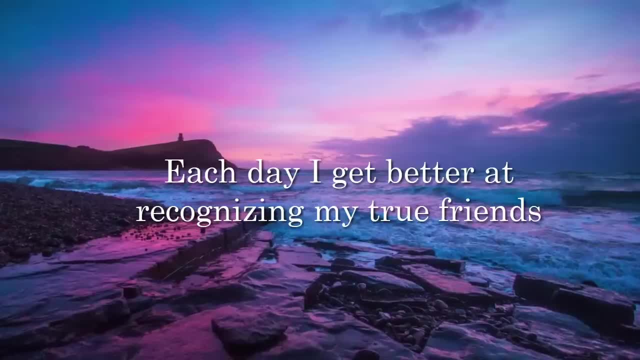 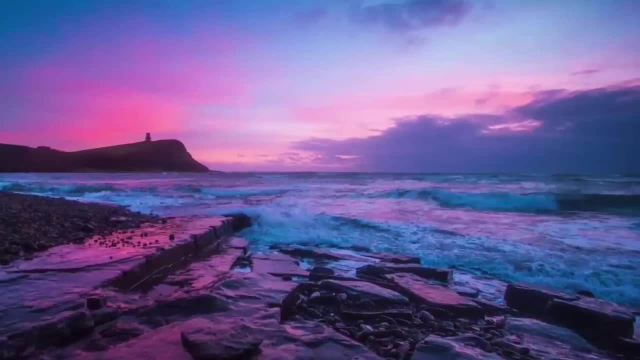 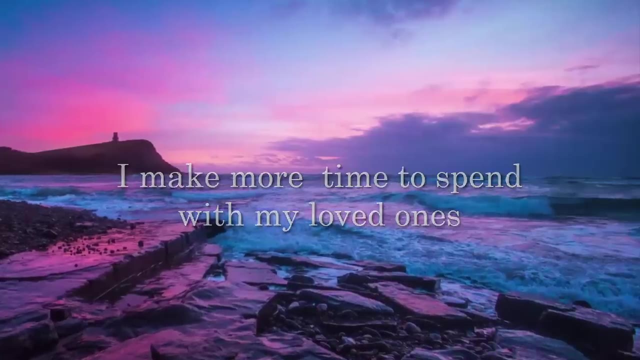 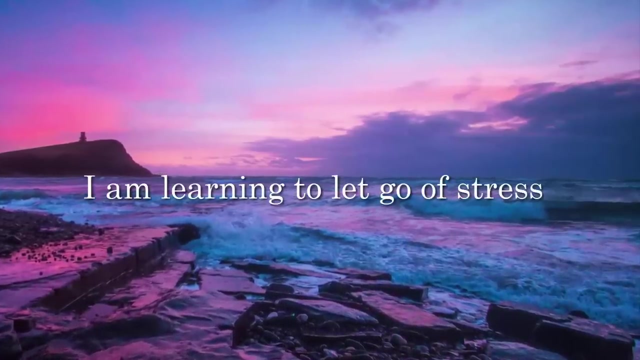 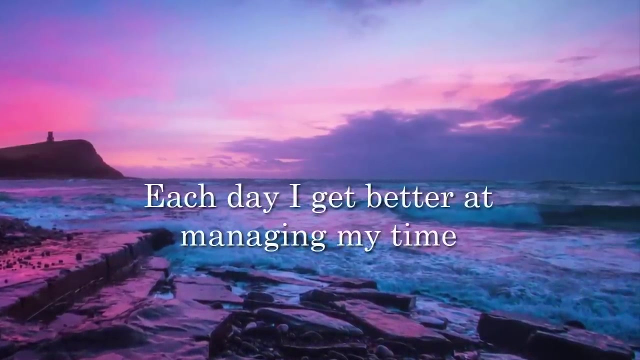 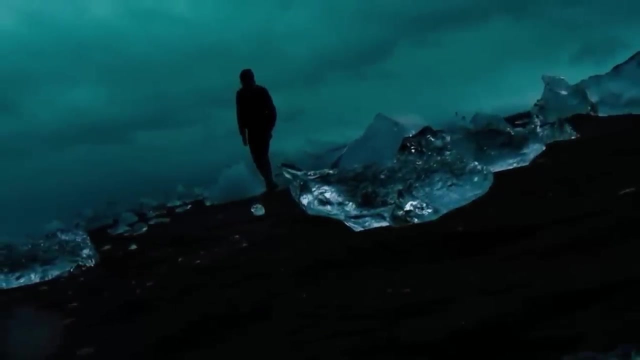 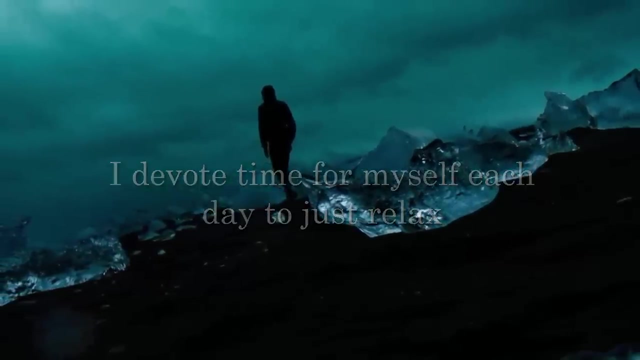 each day I get better at recognizing my true friends. I make more time to spend with my loved ones. I am learning to let go of stress. each day I get better at managing my time. I devote time for myself each day to just relax. I recognize my own worth and I feel worthy. 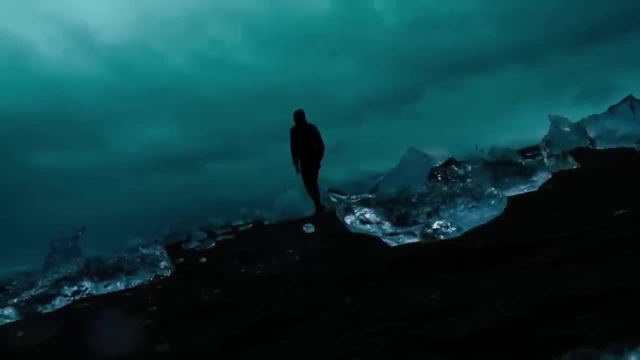 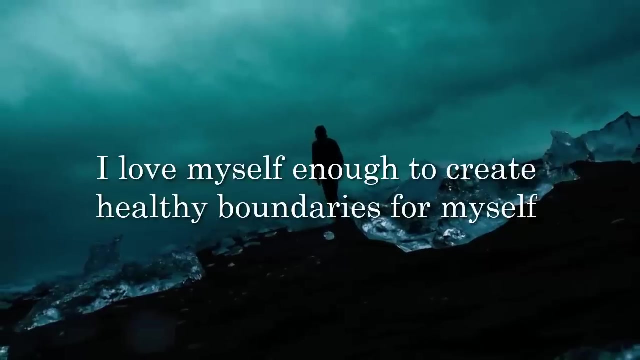 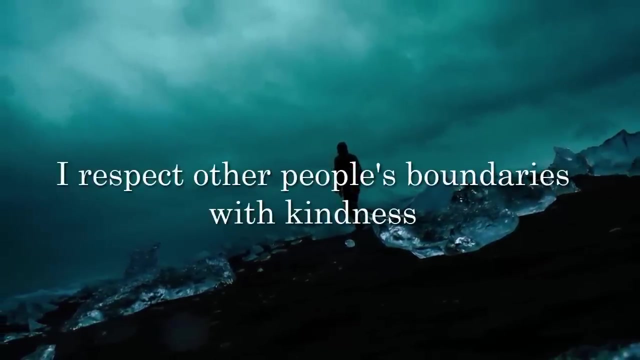 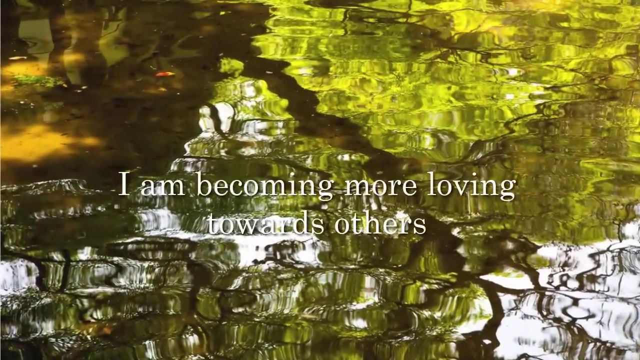 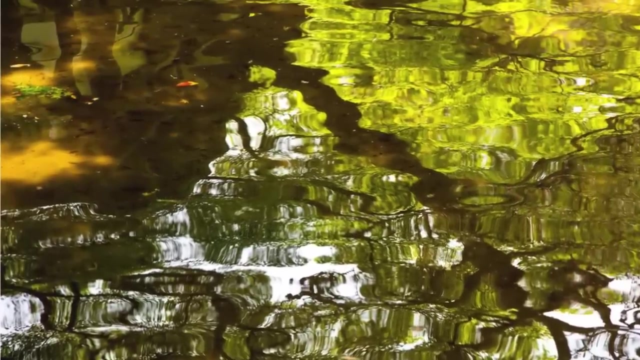 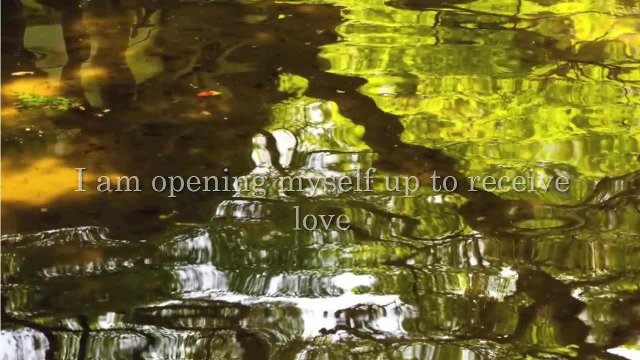 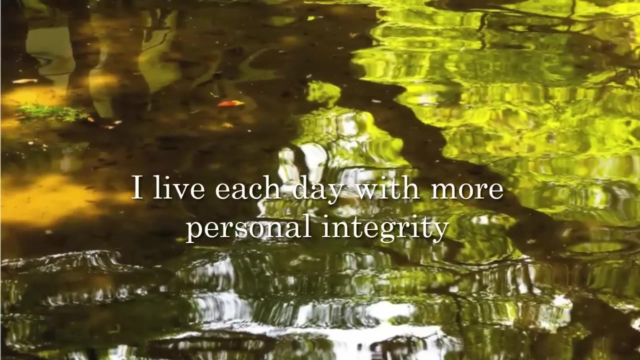 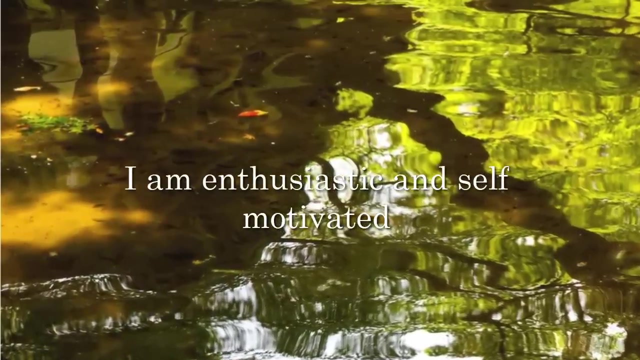 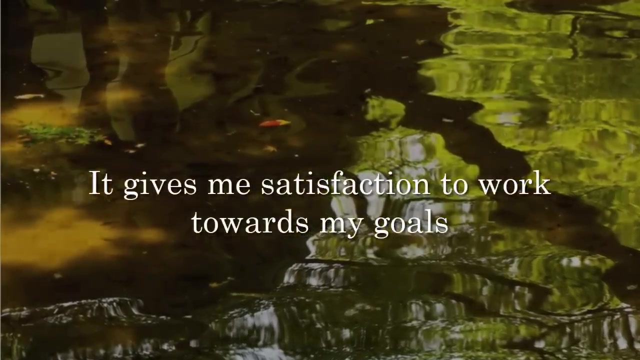 I love myself enough to create healthy boundaries for myself. I respect other people's boundaries with kindness. I am becoming more loving towards others. I am opening myself up to receive love. I live each day with more personal integrity. I am enthusiastic and self-motivated. It gives me great satisfaction to work towards my goals. 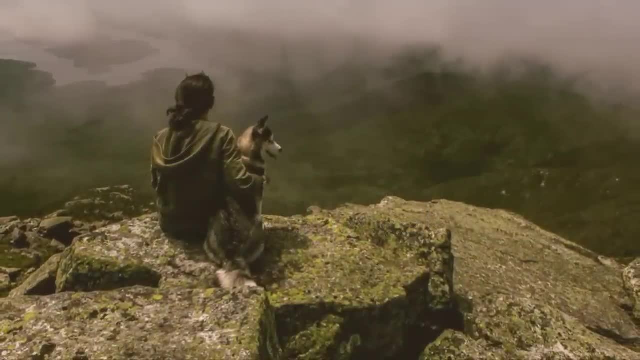 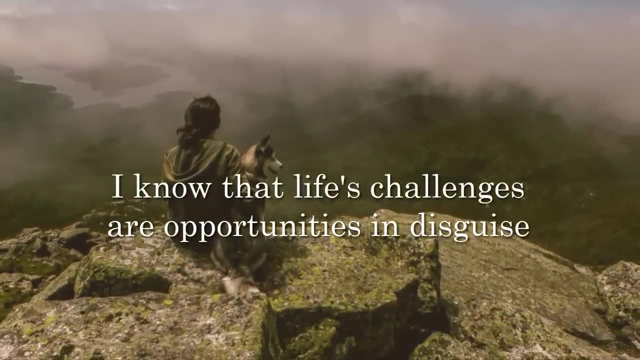 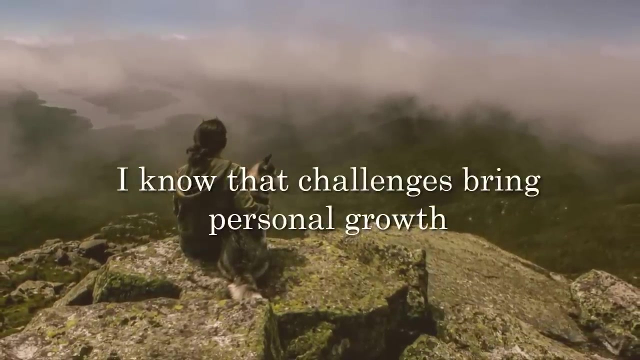 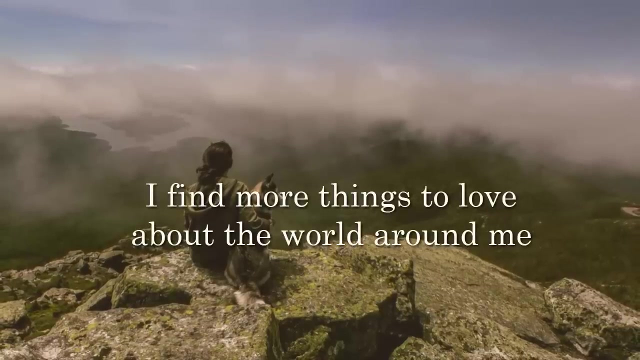 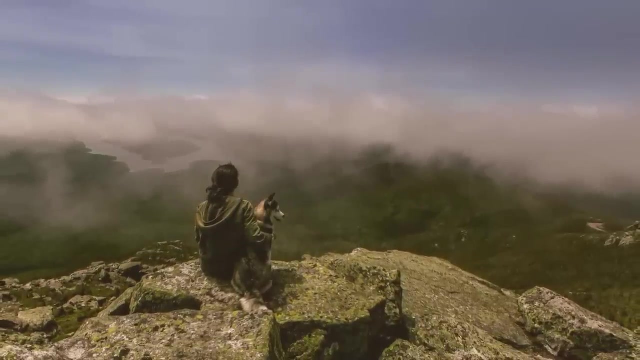 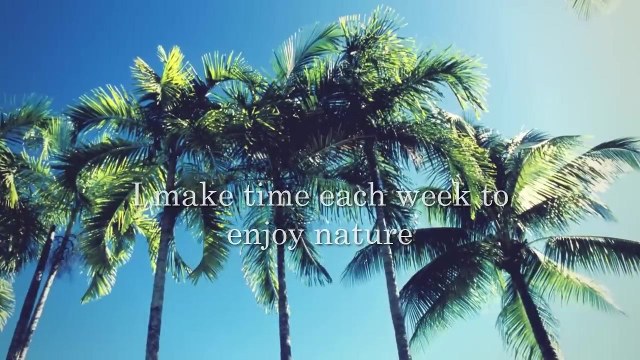 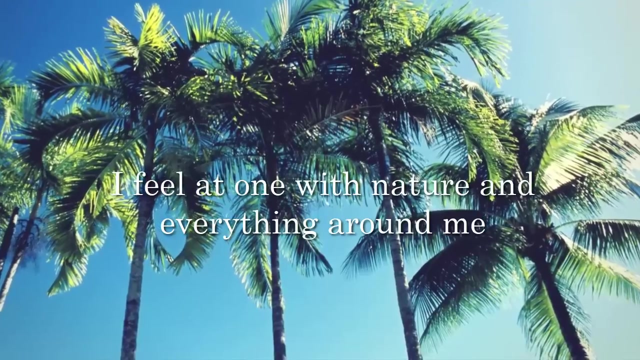 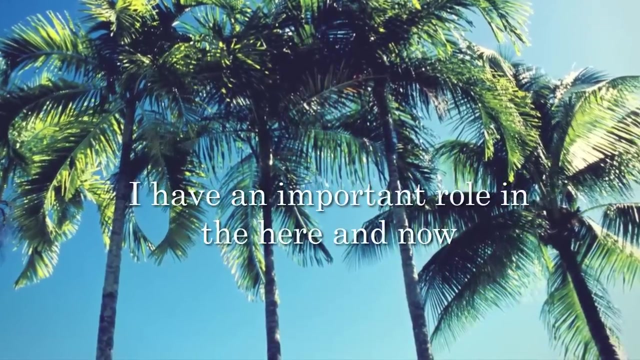 I know that life's challenges are opportunities in disguise. I know that challenges bring personal growth. I find more things to love about myself. I love the world around me. I make time each week to enjoy nature. I feel at one with nature and everything around me. I have an important role in the here and now. 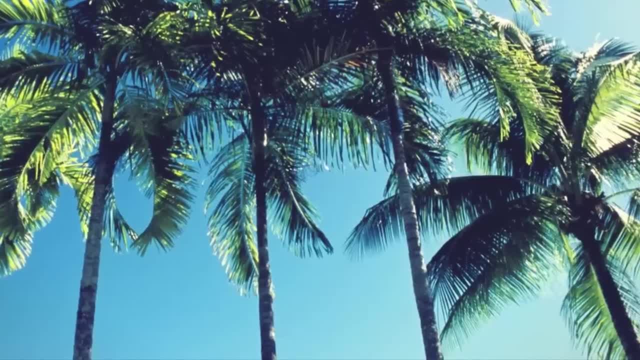 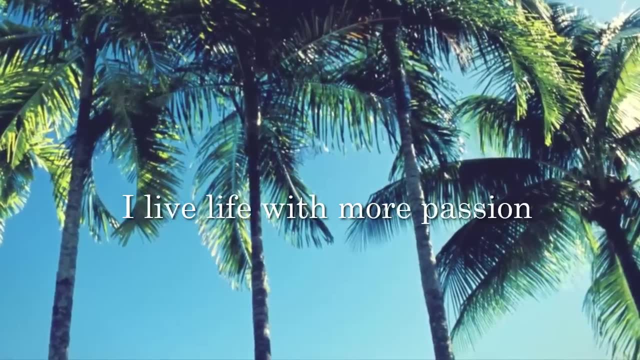 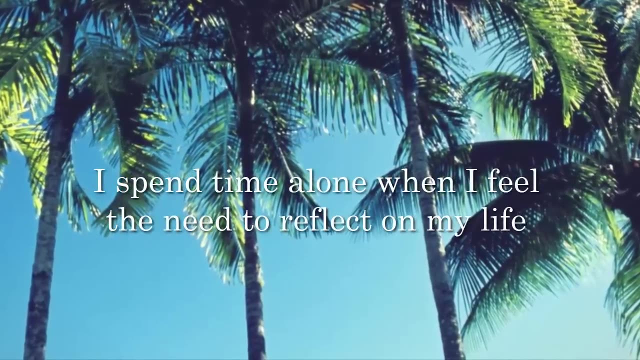 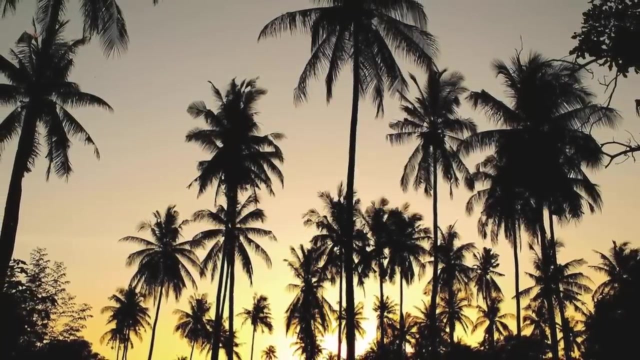 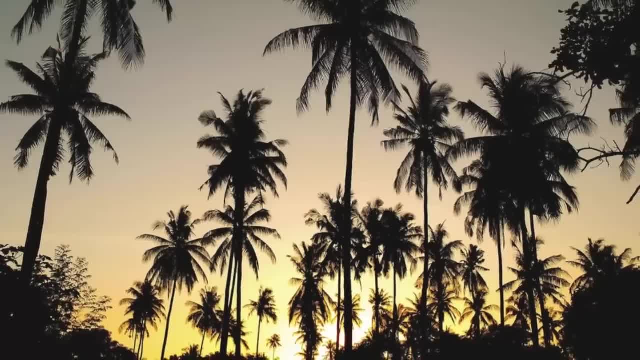 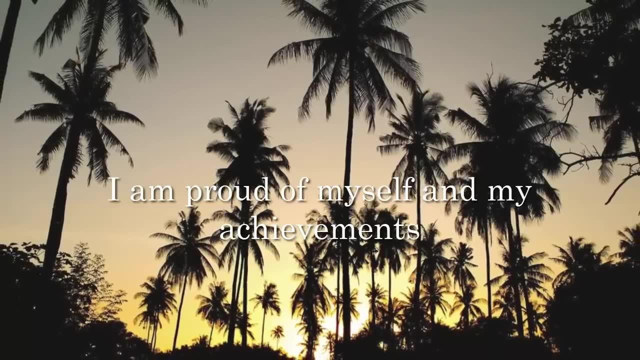 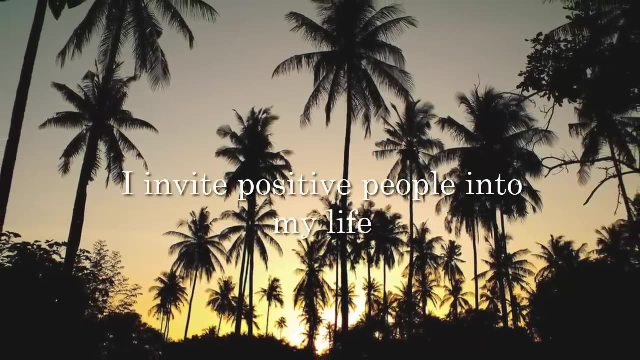 I am grateful for everything that is positive about my life. I am proud of myself and my achievements. I am proud of myself and my achievements. I invite positive people into my life. I invite positive people into my life. I can be able to do more for myself. I face challenges, live��ies and emotions. 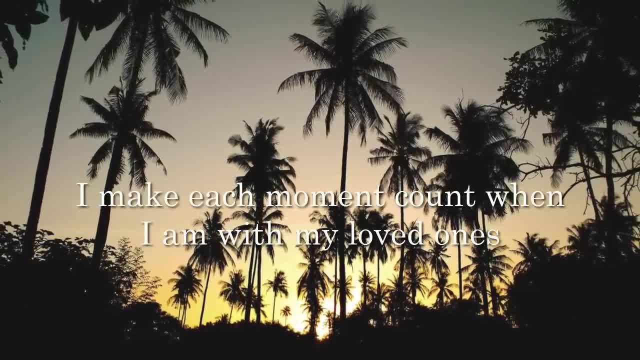 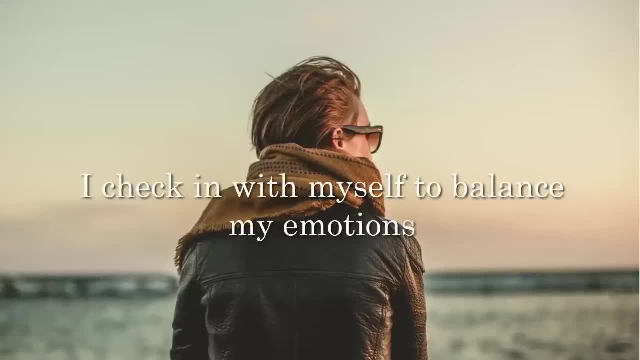 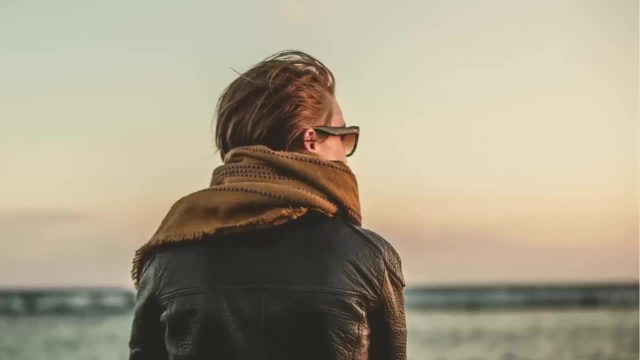 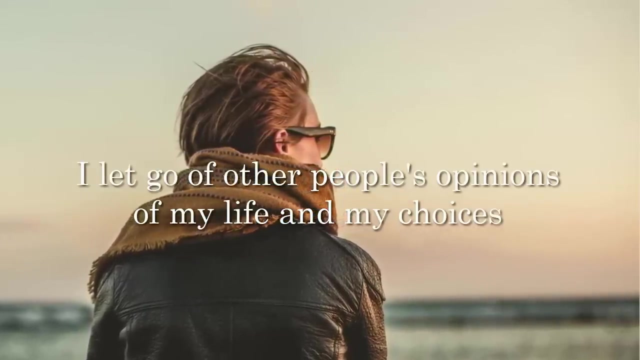 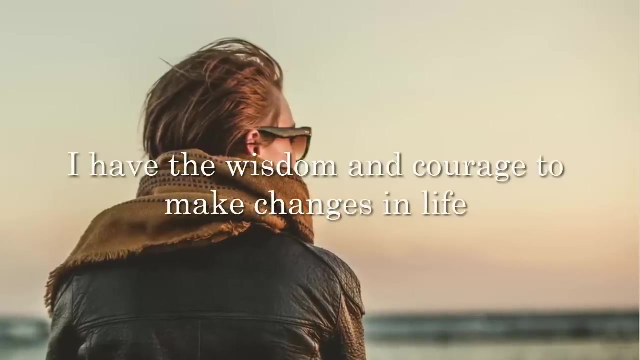 I literally enjoy every organizations I work with. Every time I think of my life, with others, Every day of my life for myself, I check in with myself to balance my emotions. I let go of other people's opinions of my life and my choices. I have the wisdom and courage to make. 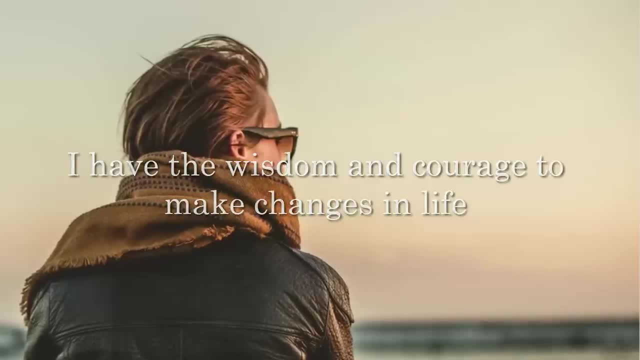 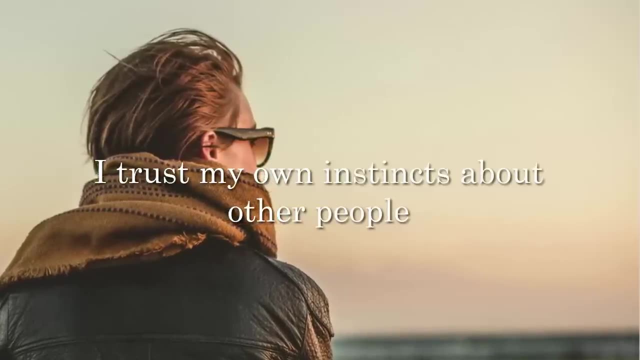 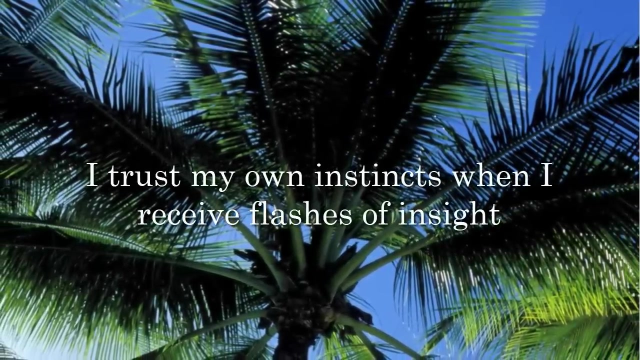 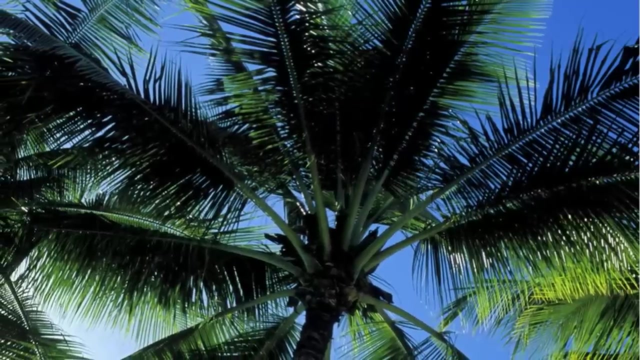 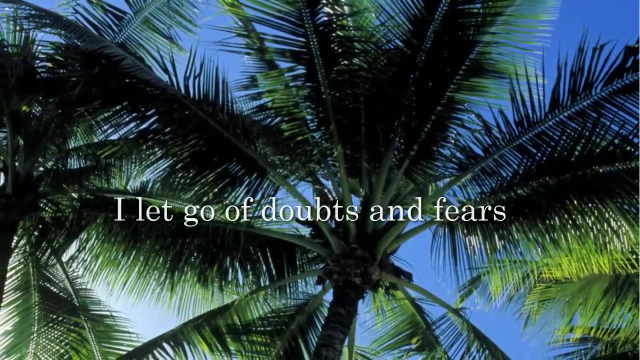 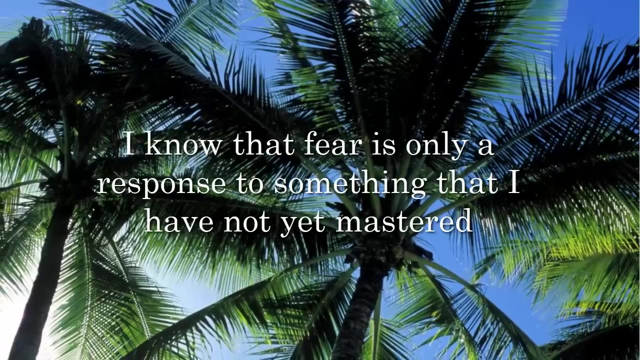 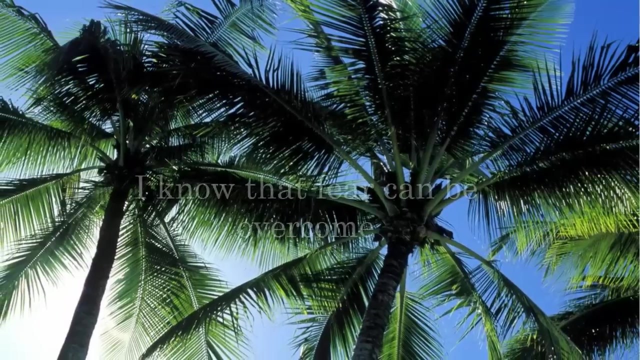 changes in life. I trust my own instincts about other people. I trust my own instincts when I receive flashes of insight. I let go of doubts and fears. I know that fear is only a response to something I have not yet mastered. I know 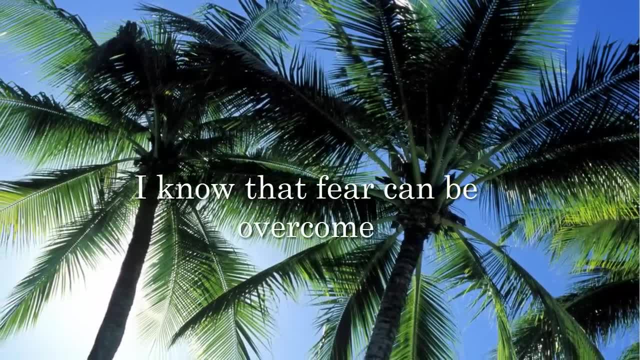 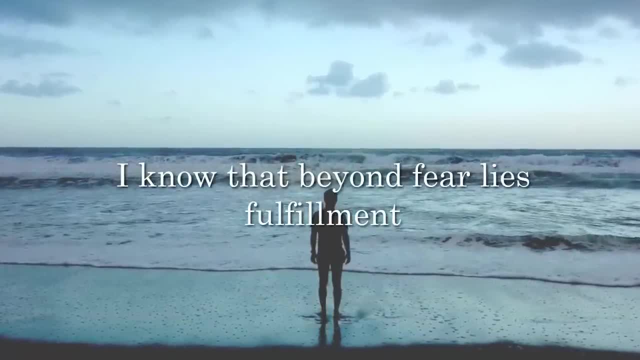 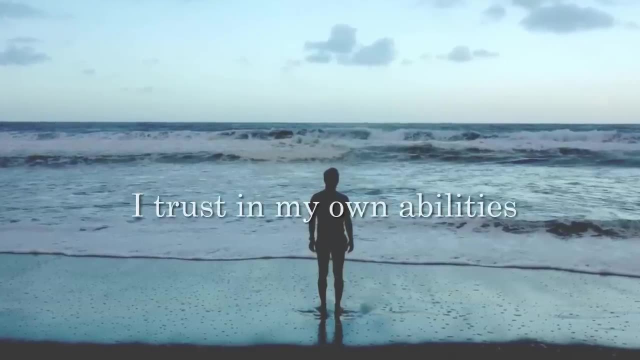 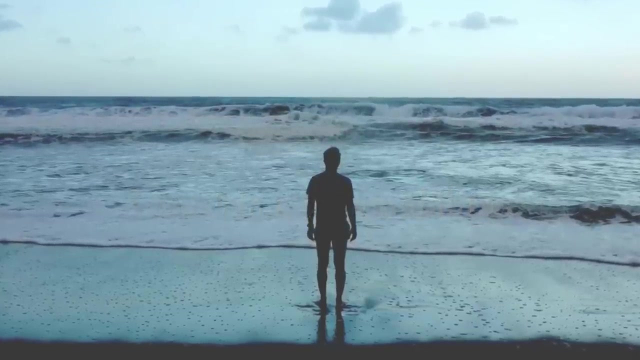 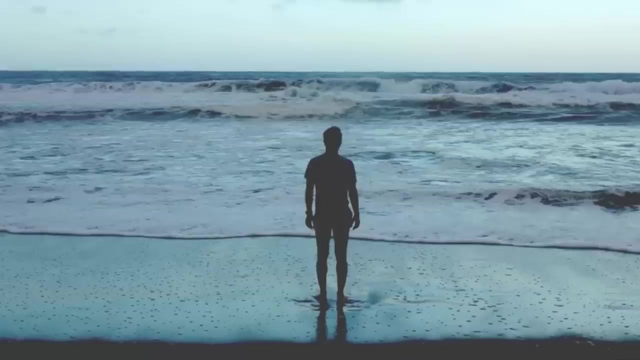 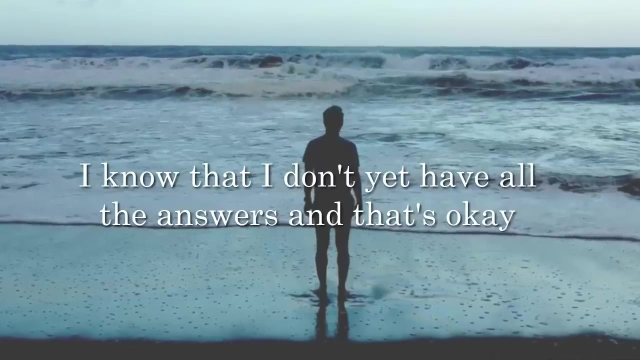 that fear can be overcome. I know that beyond fear lies fulfillment. I trust in my own abilities. I trust that everything is the way it should be in each moment. I know that I don't yet have all the answers and that it's okay. 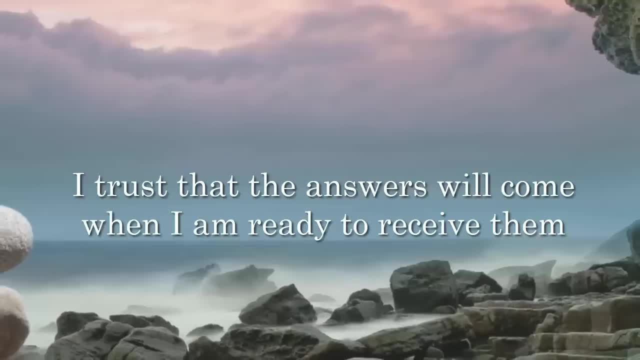 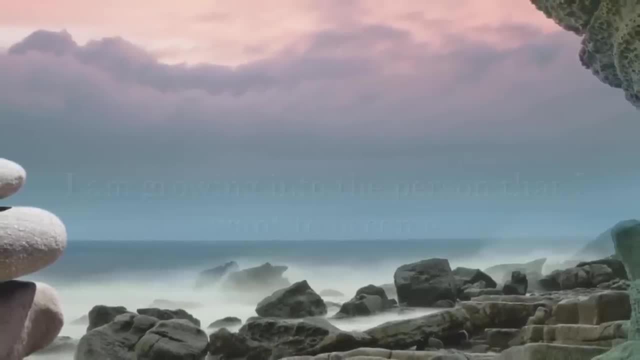 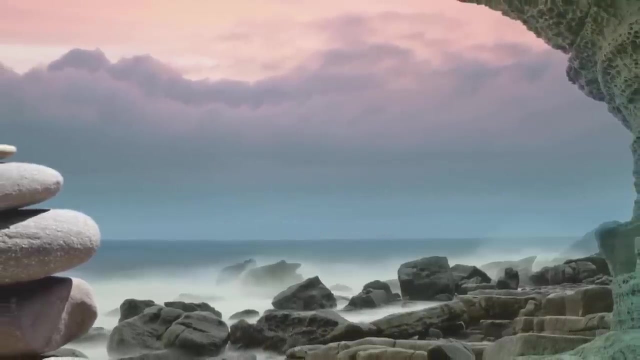 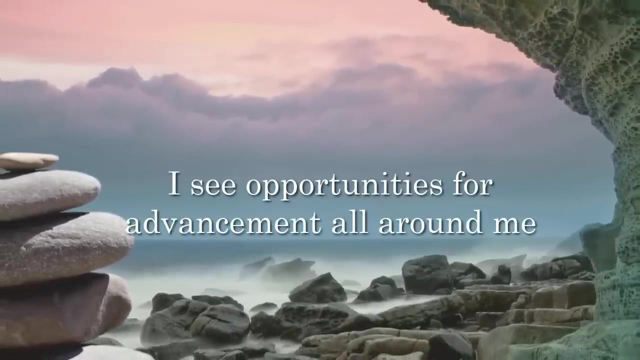 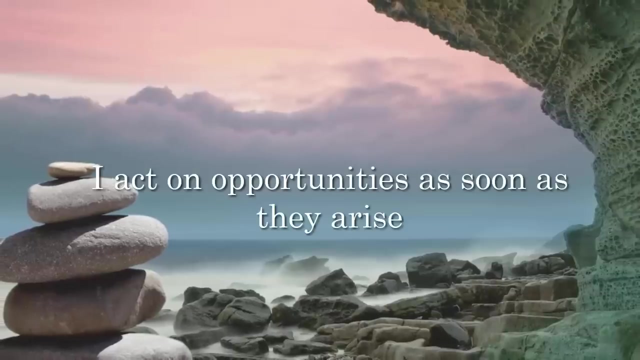 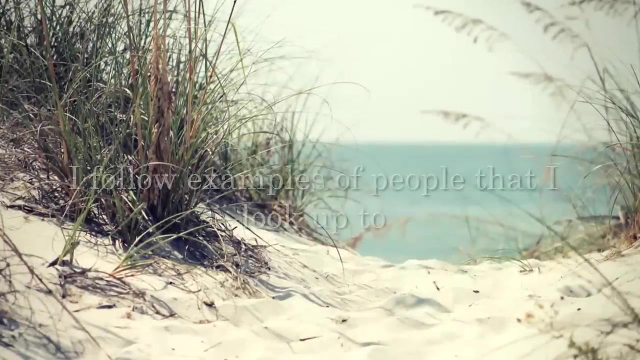 I trust that the answers will come when I'm ready to receive them. I'm growing into the person I want to become. I see opportunities for advancement all around me. I offer new opportunities as soon as they arise. I follow good examples of people. 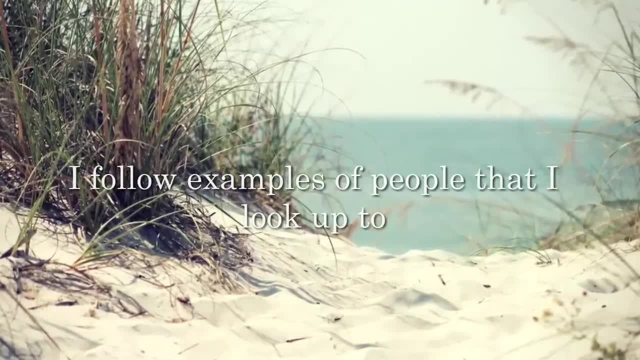 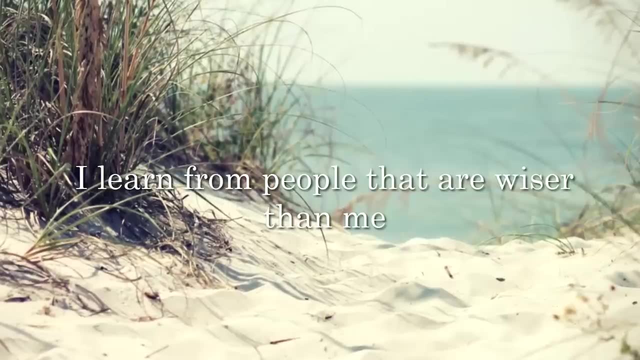 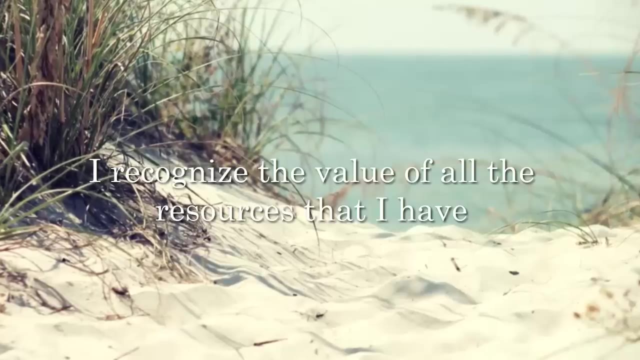 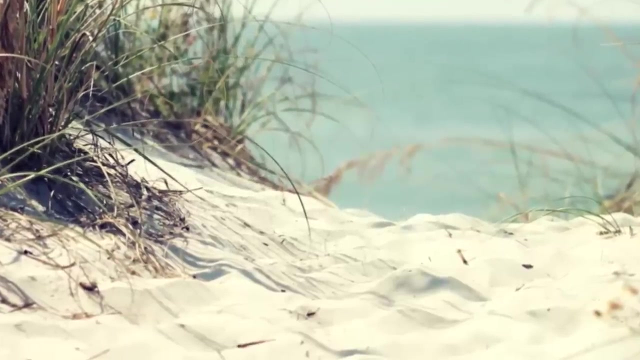 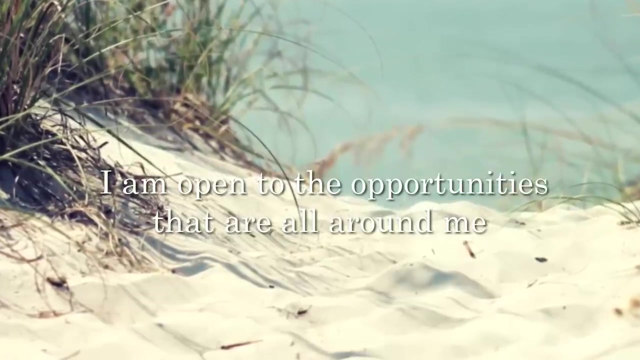 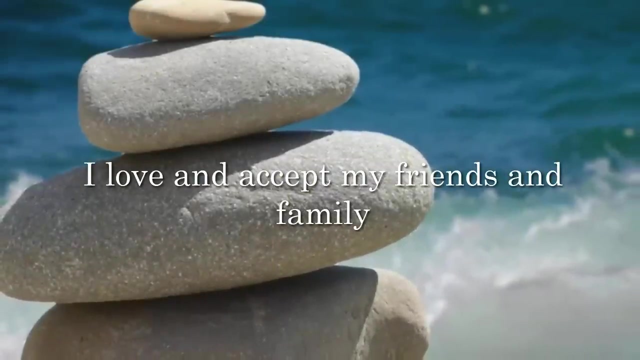 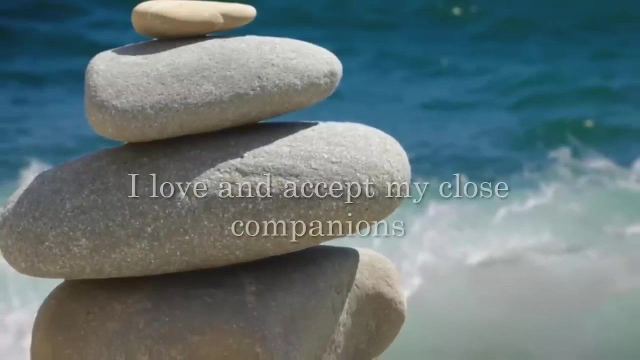 that I look up to. I learn from people that are wiser than me. I recognize the value of all the resources that I have. I have the power to be the best. I am open to the opportunities that are all around me. I love and accept my friends and family. 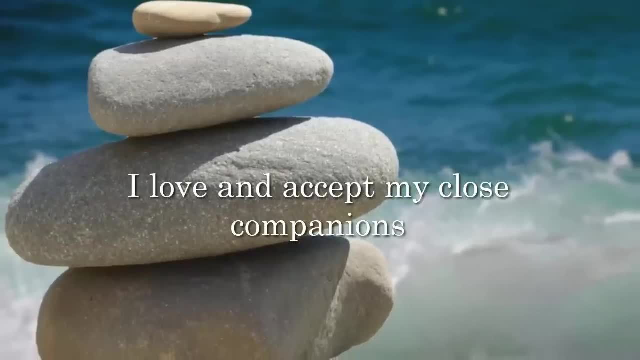 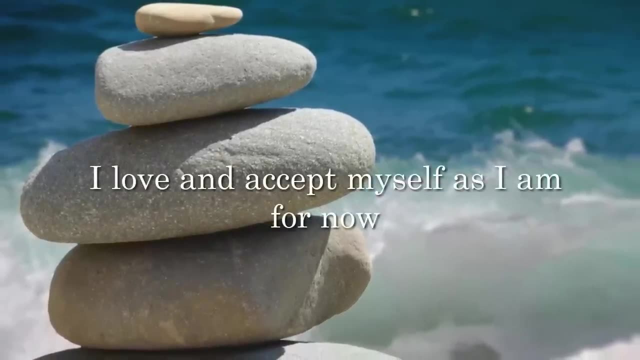 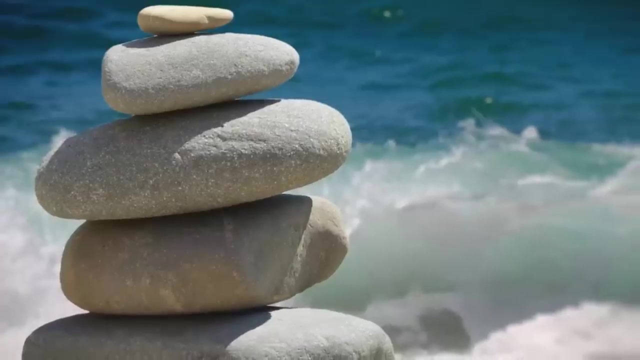 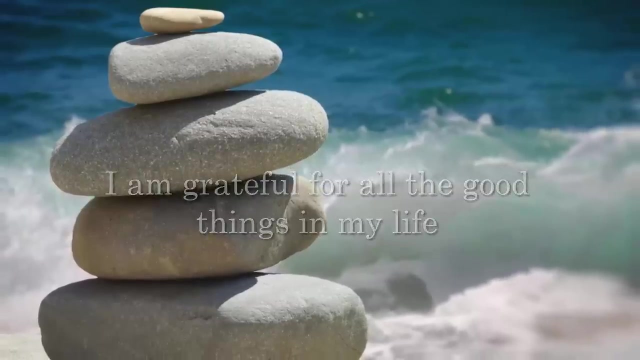 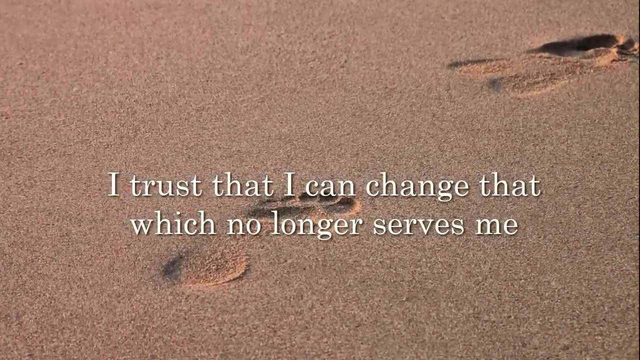 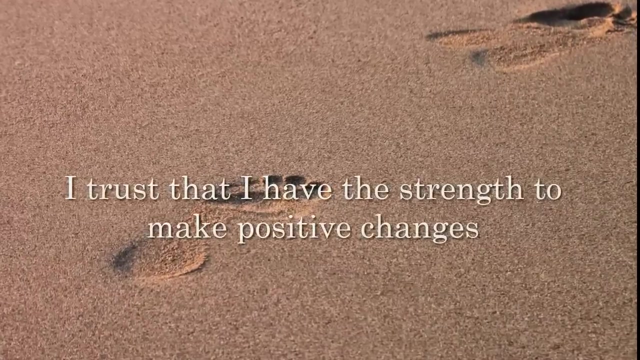 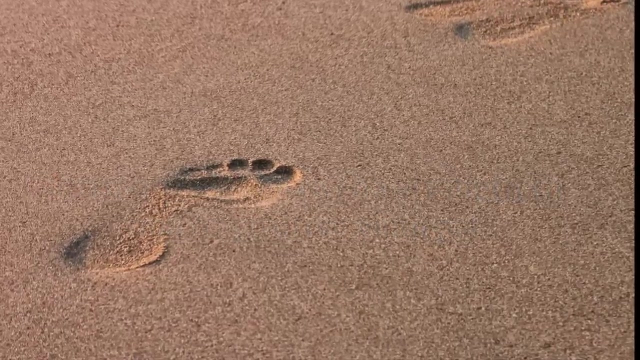 I love and accept my close companions. I love and accept myself as I am. for now, I am grateful for all the good things in my life. I trust that I can change that which no one else can longer serves me. I trust that I have the strength to make positive changes. 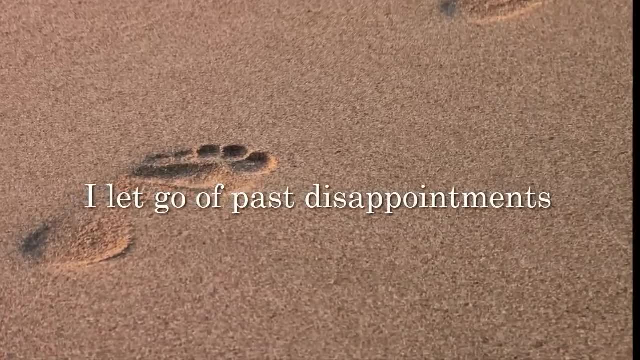 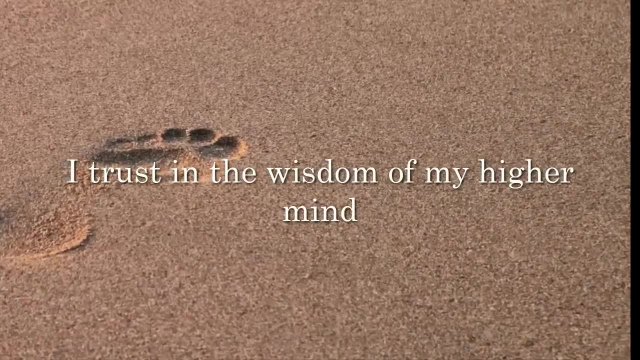 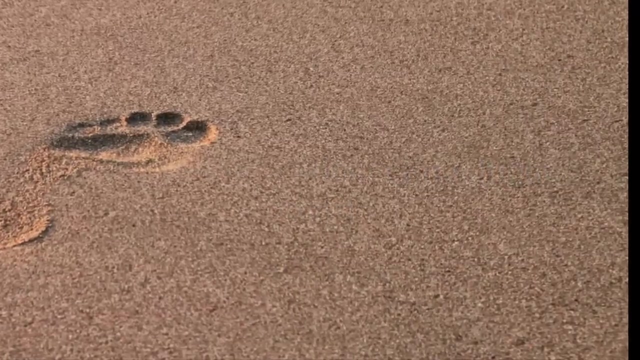 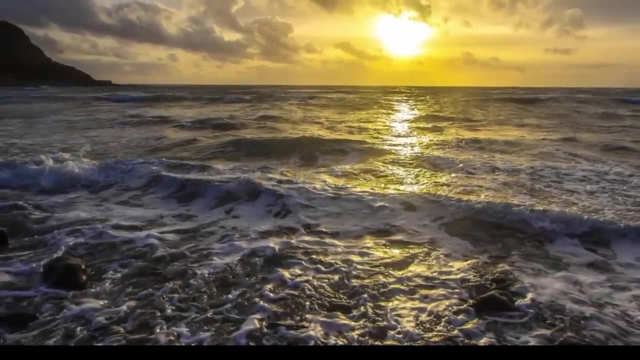 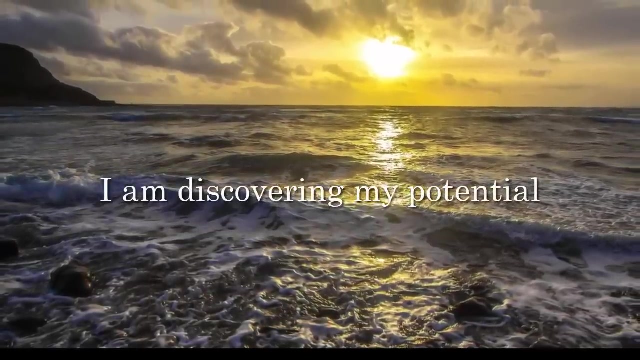 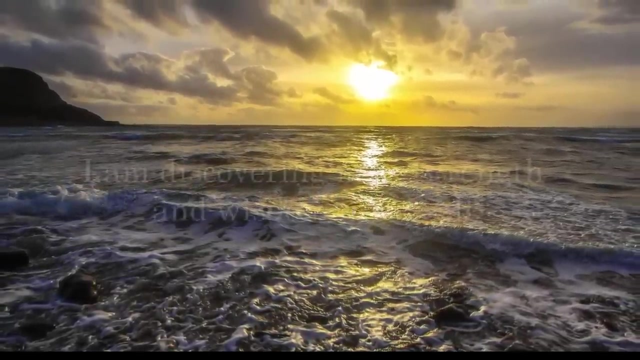 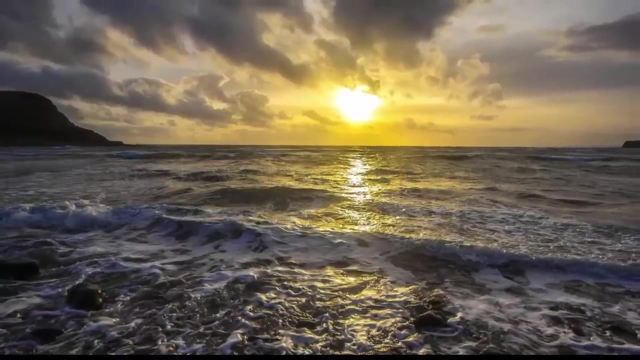 I let go of past disappointments. I trust in the wisdom of my higher mind. I look forward to discovering new places, things and people. I am discovering my potential. I am discovering more strength and wisdom in myself. I am determined to achieve whatever I hold in my mind's eye. 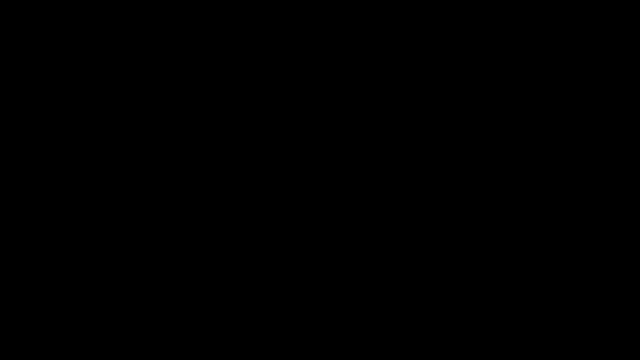 I am determined to be the best person in the world. I am determined to be the best person in the world.